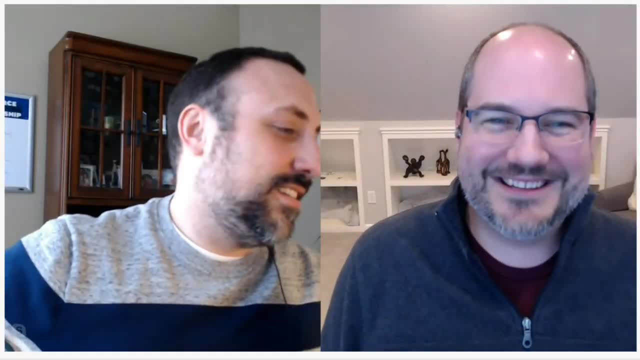 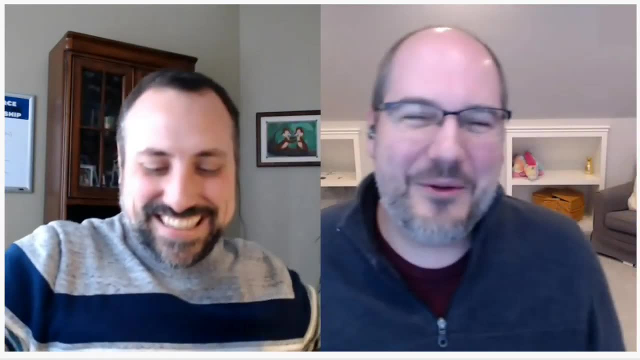 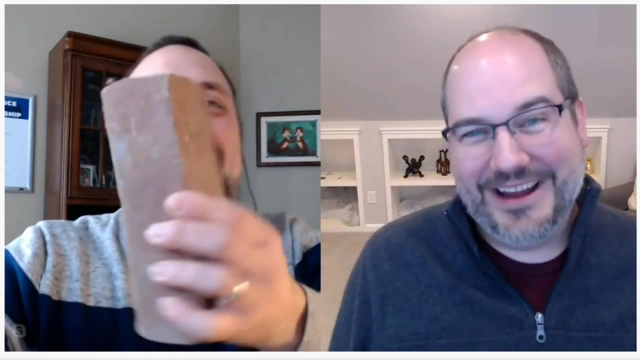 Well, I have a prop for today. What You never have props: A brick. Hey, you can't replace me with a brick. You can't replace me with a brick. It's not going to work. We'll figure it out, alright. 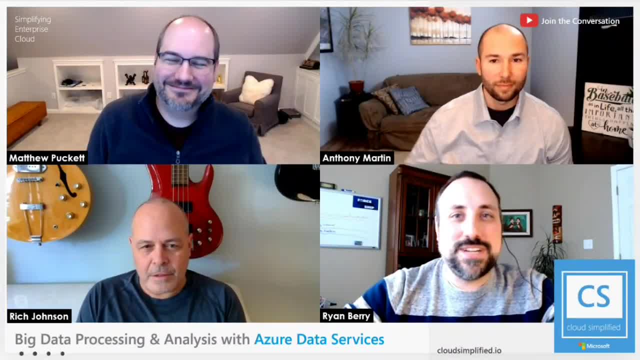 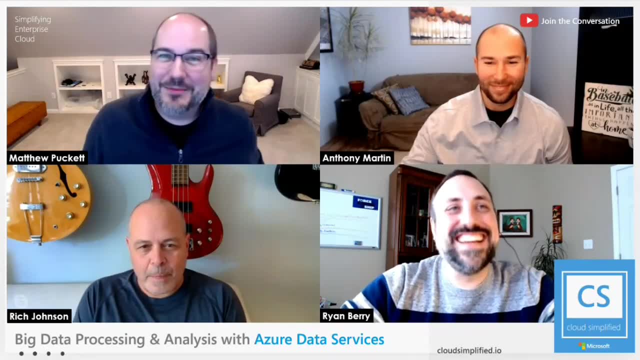 Well, hello again, Matthew Hey Ryan, How are you doing today? I'm doing well. Are you ready to try to simplify the cloud? Well, I hope so. I see we have two guests to help us do it. I'm looking forward to it. 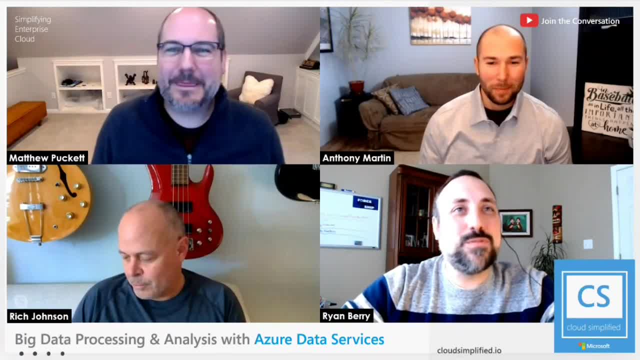 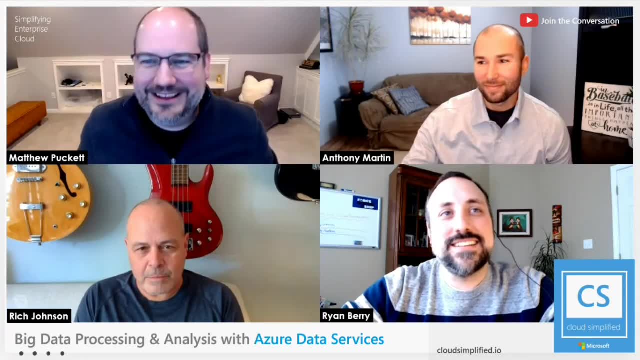 We'll give it a good try. Oh good, Good, I know it's been a while. I see you've got some new iHardware. Yeah, yeah, yeah, Headed up my games Slowly. smarter, right, I got a little rug going. 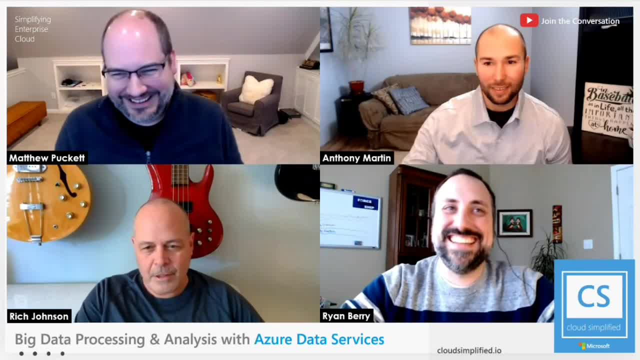 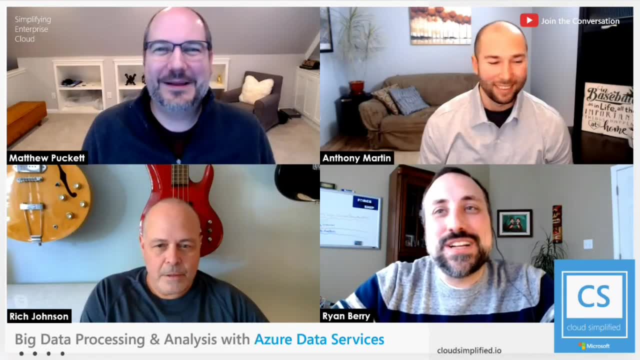 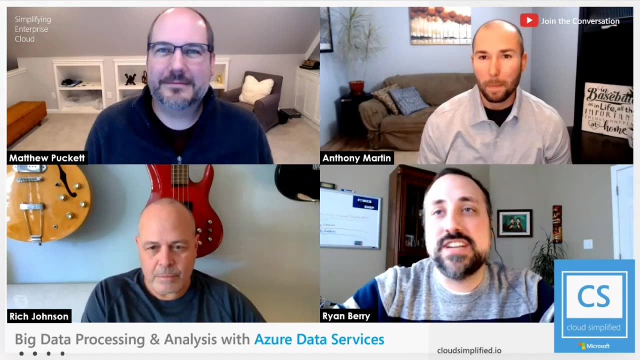 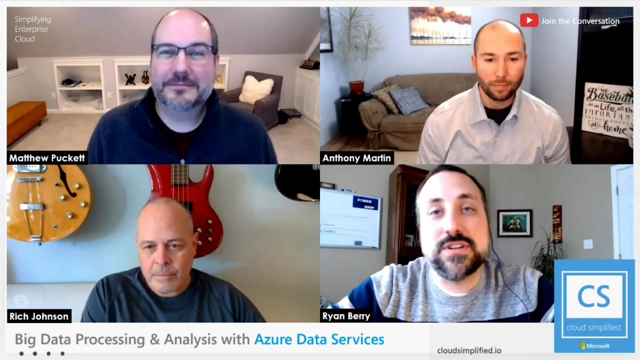 Yeah, that's quite a bit of rug that you got. Oh, that looks good. All right, So let's go ahead and introduce our guests that we have on today. Let's do it. Yeah, So we have Rich and Anthony, who are going to talk to us a bit about how they've used Databricks and machine learning to do some cool things for a customer of theirs. 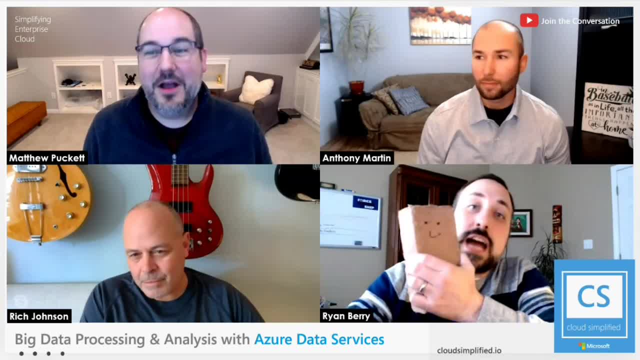 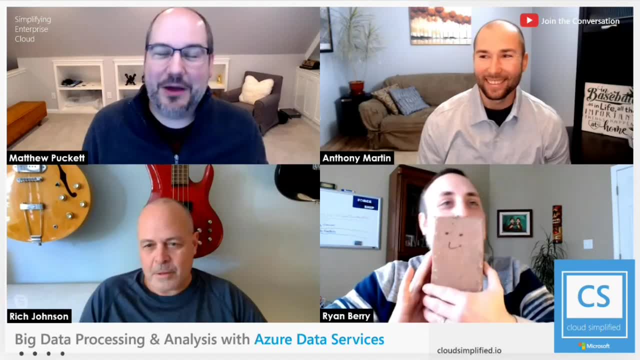 All right, What I hope to get out of all this is how they get data in this. Absolutely Hey, what's its name? You got to have a pet name for that, right? Yeah, Yeah, Is that Pet Rock Rocky? 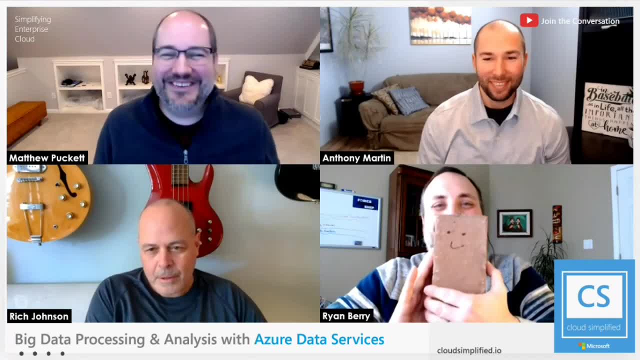 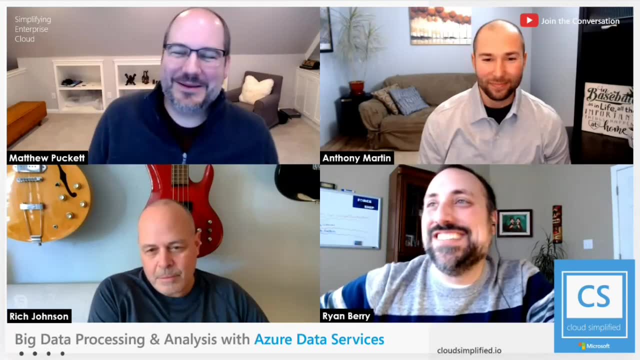 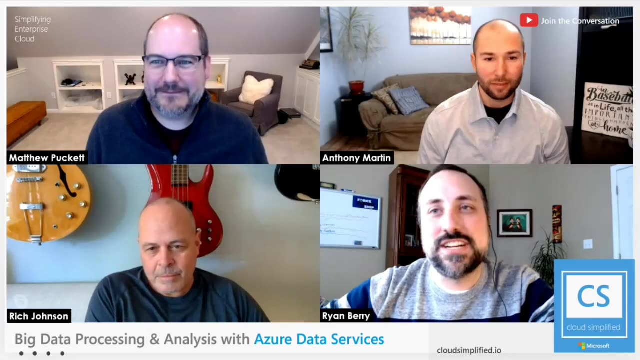 Oh, I need a Matthew. Oh, You can't replace me with that. I'm sorry. I have way more personality than a brick, I think. All right. So, Rich and Anthony, why don't you go ahead and introduce yourselves and give us a little, a little bit of a feel about what you're going to talk about today? 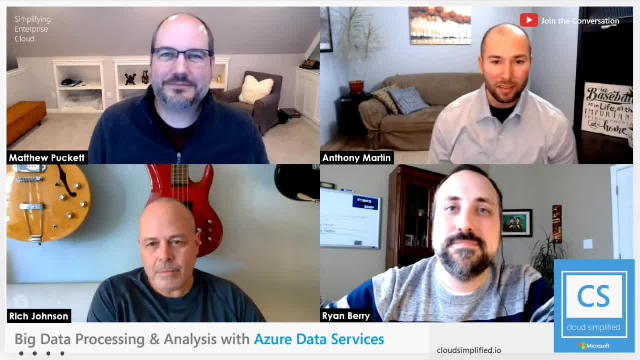 Sure, Certainly So, Anthony Martin. I'm a cloud solution architect out of the Buffalo, New York area, And what we're going to talk about is kind of a generic case study of a client that we worked with, an R&D. 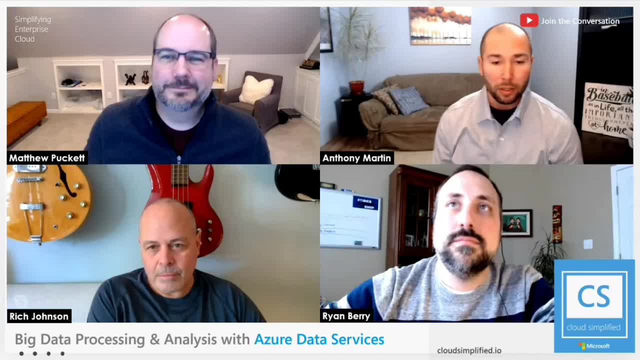 that we weren't able to do before, and what we're going to talk about is kind of a generic case study of a client that we worked with with together, along with another client of ours, Trey Talbott, to handle big data processing. 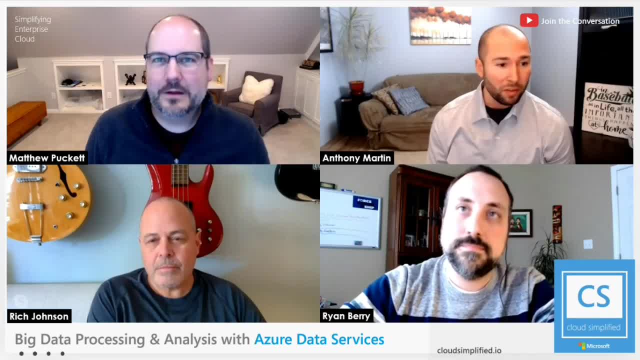 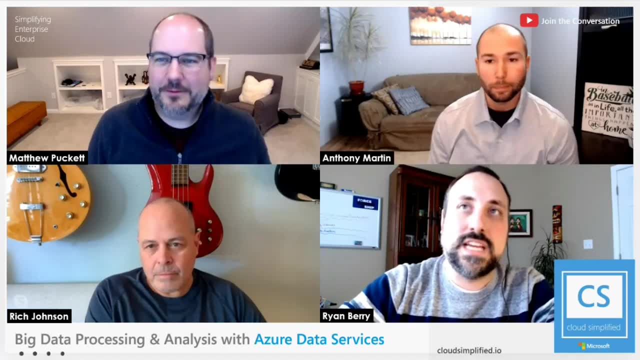 in Azure utilizing and kind of determining what's the appropriate services, because there's quite a few to choose through for the different requirements that we have with our client. Yeah, I know data is certainly growing at an explosive growth or explosive rate with 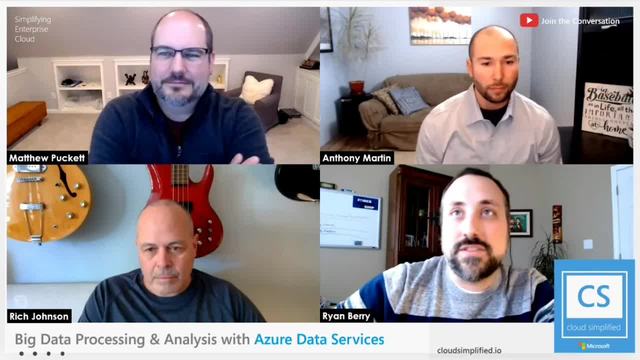 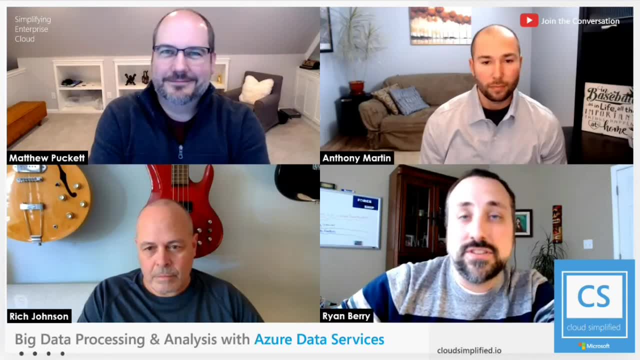 our customers. You know they're looking for ways to make sense of that data and be able to do interesting things to you know, predict the future if you will, or, you know, make informed decisions. You know so, and Databricks is just one of the plethora of services we have, I know. 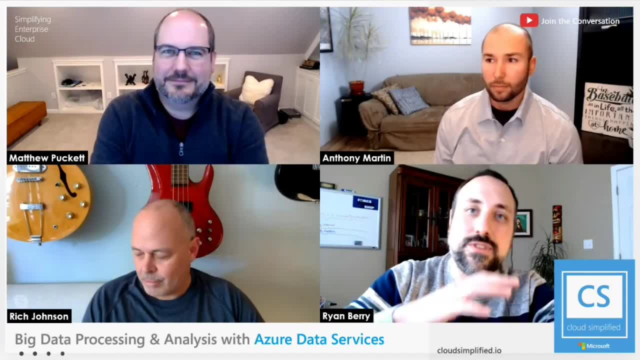 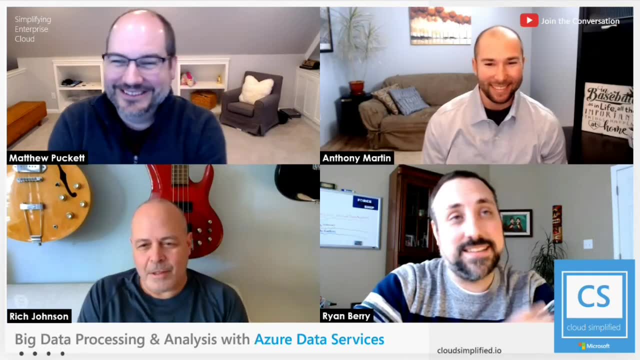 in Azure to be able to help customers do that. So looking forward to kind of hearing how this actually was applied to your customers. Yeah, I want to hear how a brick can predict the future, please. Yeah, yeah, I'm looking for that one. 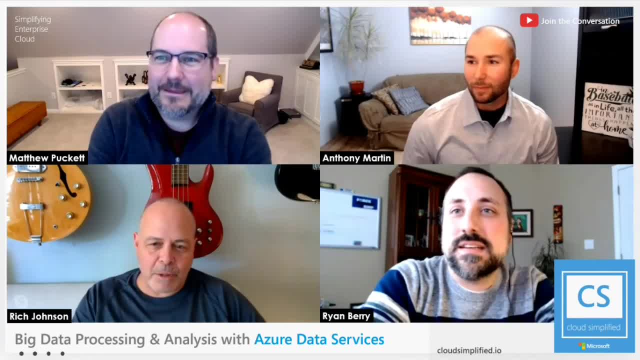 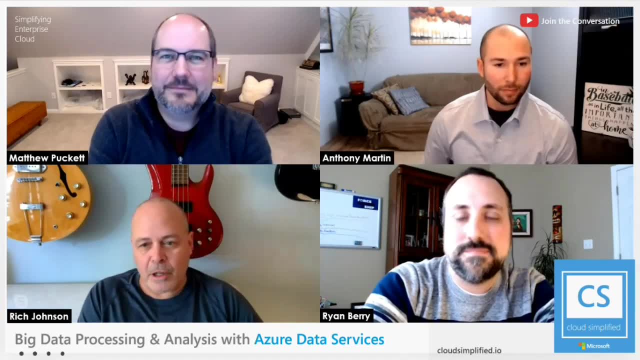 Yeah, Hey. so I'm Rich Johnson, I'm a cloud solution architect as well, And Anthony and I kind of Teamed up on this effort here at this particular customer that happened to have a pretty ungodly amount of data for weather data. 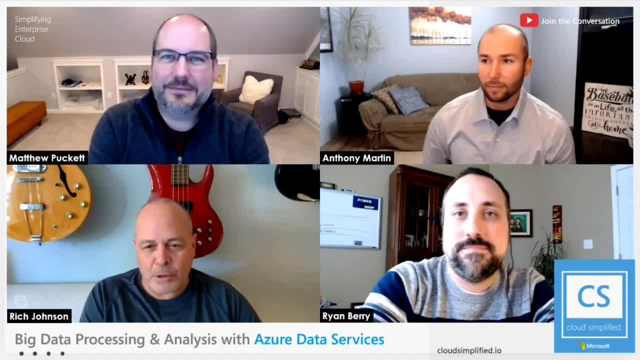 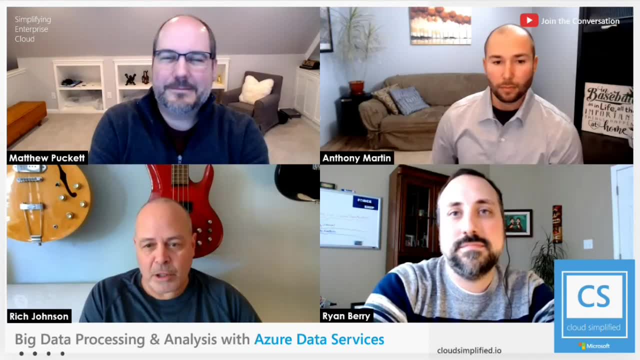 And you know they had spent some time trying to do some things on their own with another implementation, a Hadoop implementation, and just weren't getting very far. just the amount of effort to manage that service and to get the kind of performance for some of the simple. 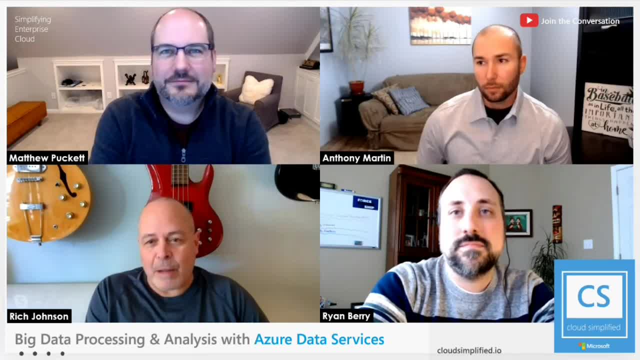 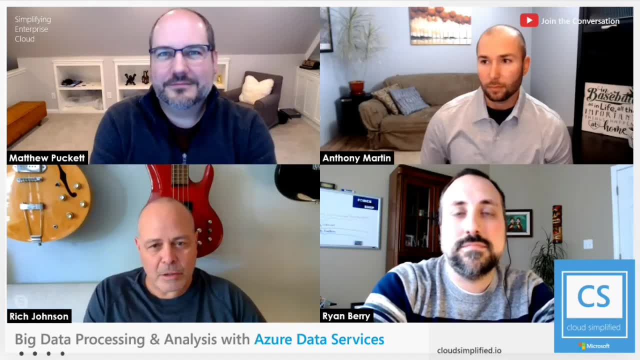 reports they're looking for. So this Databricks just happened to come along towards GA and Azure back in the spring And it's just like at that time Anthony suggested and others like, hey, let's try this new service that's just going to general availability. 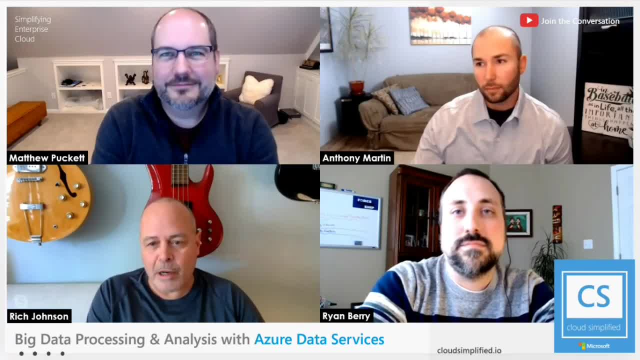 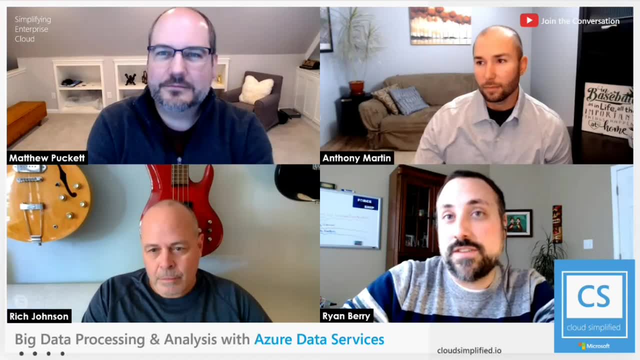 And we were quite surprised, and pleasantly surprised, with what we found and how well it worked. Okay, So you said two things that I'd like to click into a little bit. You said a lot of data, So like, can you quantify that in terms of, just like, sheer? you know the volume in terms? 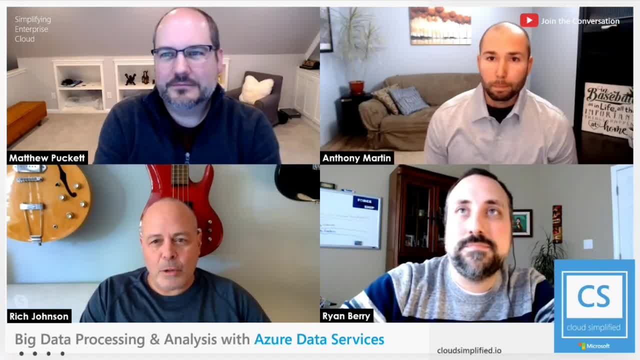 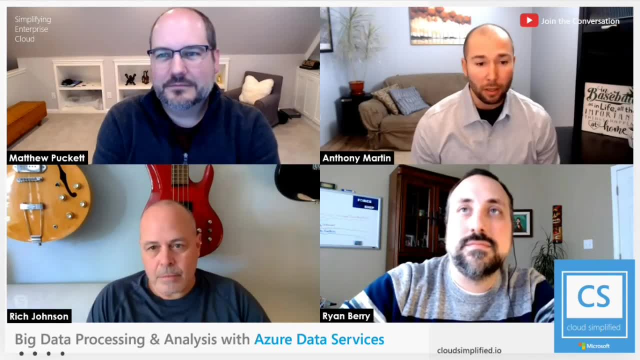 of size. Yeah, Anthony, you might want to go into that because I think you got a few notes on it, but it's pretty big, Yeah. So we have over 600 gigs of data- compressed data- coming in per day. 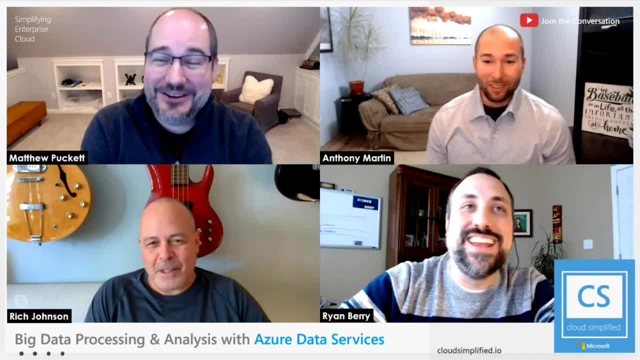 Per day. Holy cow, What Whoa, whoa, whoa. Back that up. 600 gig a day. Yeah, When you were saying 600 gigs, I'm like: yeah, that's decent. Yeah, I was like: is that really a big database? 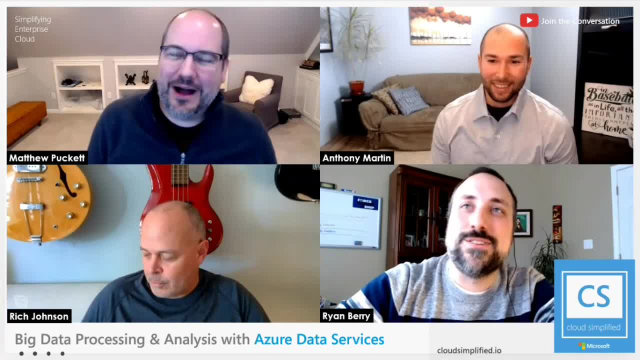 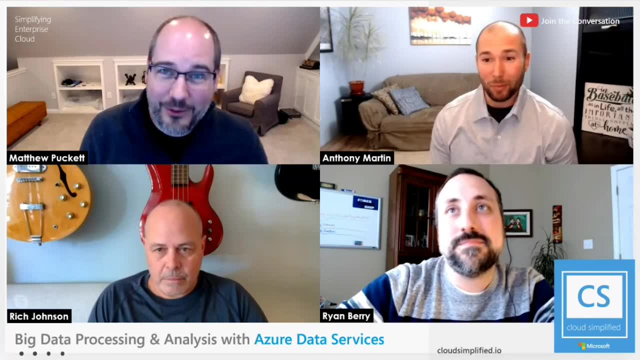 Per day was the kicker. so Yeah, Oh, yeah, Yeah, Wow, That is a lot of data, Okay, So in a month, I mean we're talking close to 20 terabytes or so, and you can extrapolate. 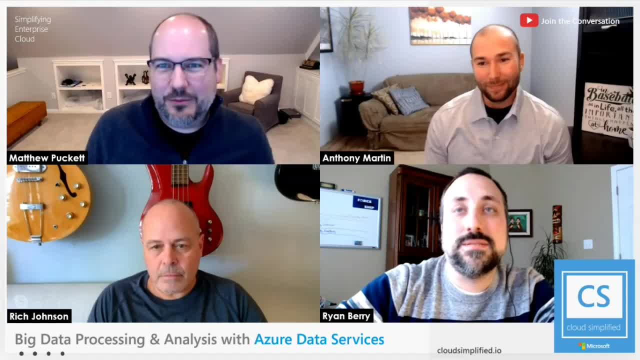 over. you know, for larger timeframes, for sure, You know someone's going to watch this video. you know, Ryan, and they're going to go. man, if we could have got that on on-prem storage, we'd be rich. 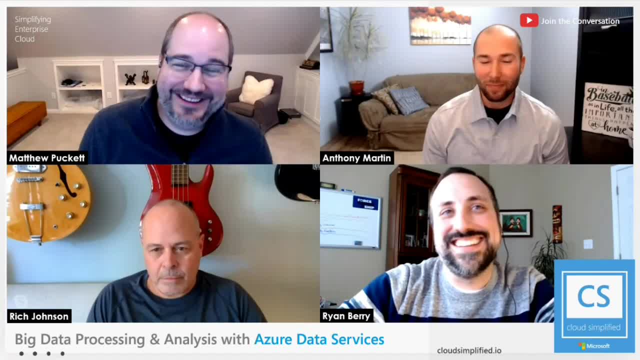 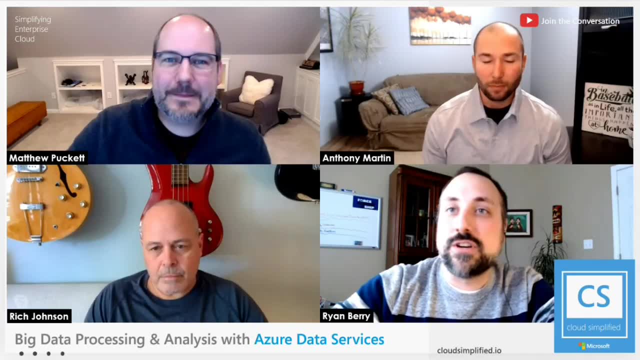 Yeah, Yeah. So we've got some storage vendors that would love to be all over that area. So, and then the other thing that you said was Hadoop. I know that's another solution for storing, you know, large quantities of data and being. 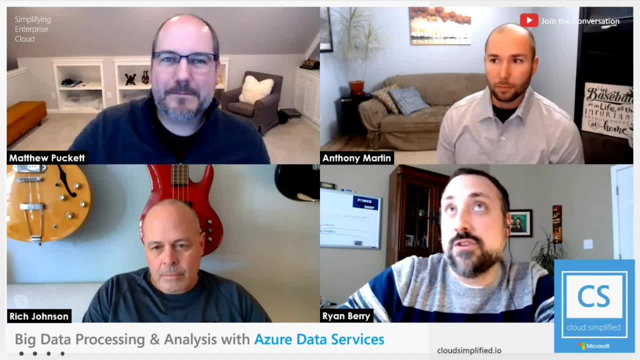 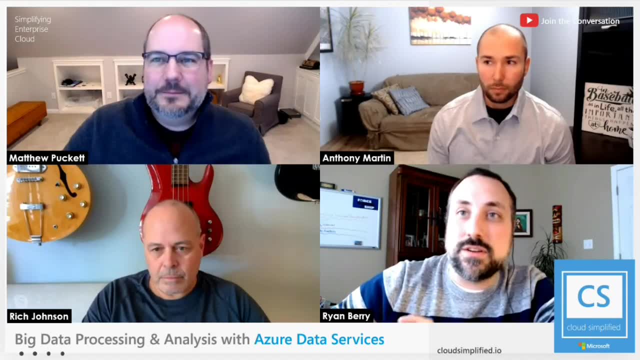 able to report against it, and you know it's not a- I don't want to say it's a bad solution, but do you want to highlight what maybe some of the challenges are in? you know, hosting in that environment or maybe what, what sorts of things that a customer has to? 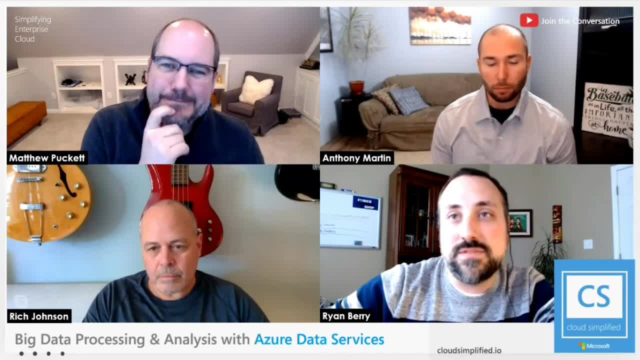 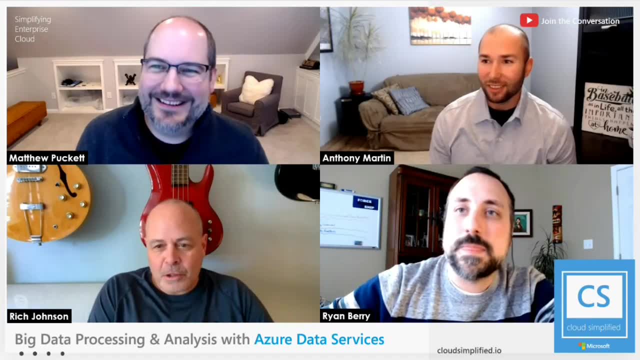 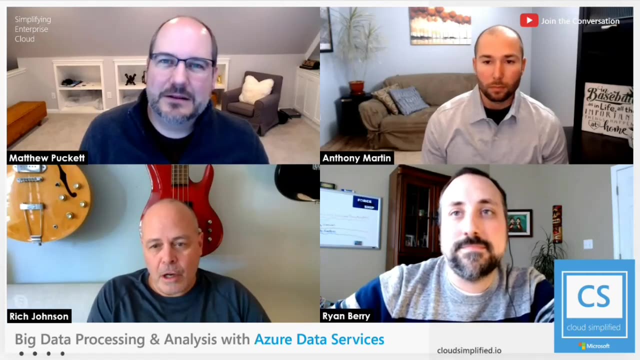 take on the responsibility for when they're storing data in that type of environment. Chris, you're on. Yeah, So just from a Hadoop standpoint right, there's a lot of care and feeding just to operate and manage a Hadoop cluster. 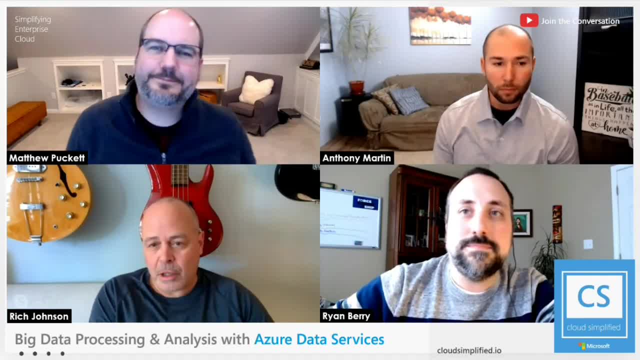 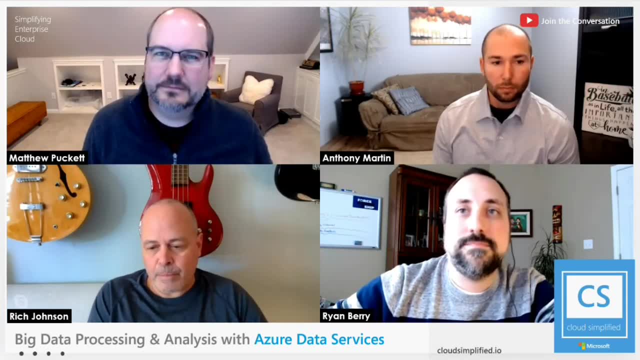 I mean you often need some very specialized expertise. Yeah, Yeah. So it just goes into that and that, not only that, and keeping up with patches and upgrades and on top of trying to tune things. it can become very challenging if you don't. 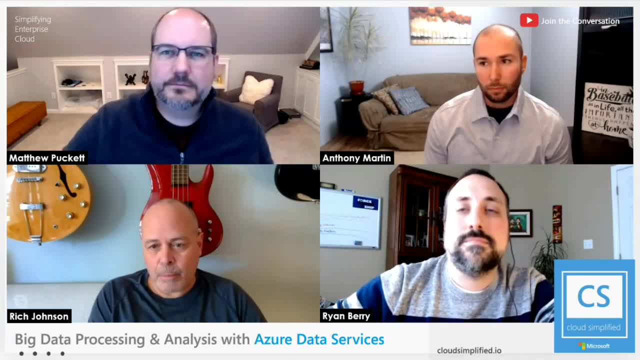 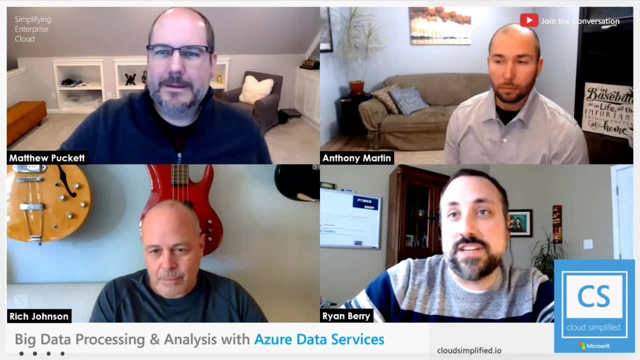 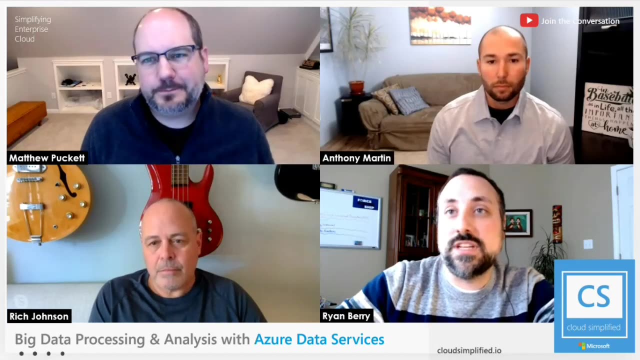 have those kind of resources and very deep resources on premise or on your team to actually do those things. Okay, I'm glad you said that, because that was what I was hoping. you were going to say: that using a service or a capability that is an as-a-service solution in Azure, you know, certainly merits. 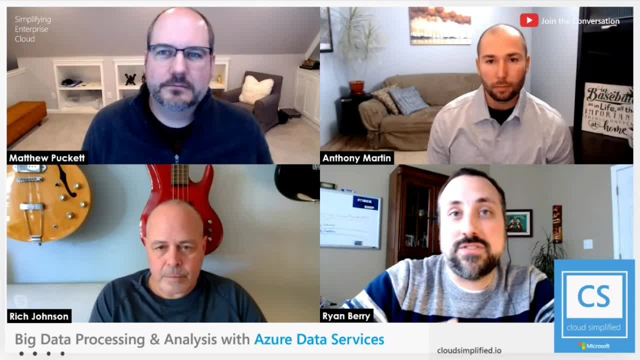 well or bodes well for business. So I think you know we've got a lot of people in our business looking to do interesting things, to explore data, but they don't have to worry about the, like you said, the care. 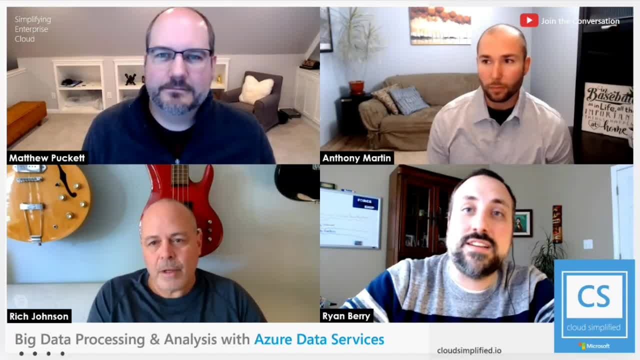 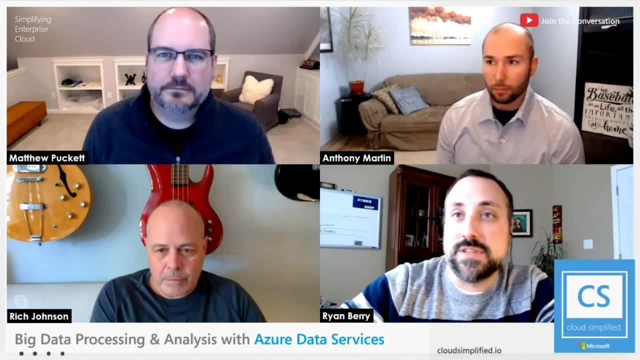 and feeding. you know the administration overhead, the. you know the technical intricacies of. you know how these pools and machines communicate with one another. We just abstract that all away from them in, you know, with the Databricks. 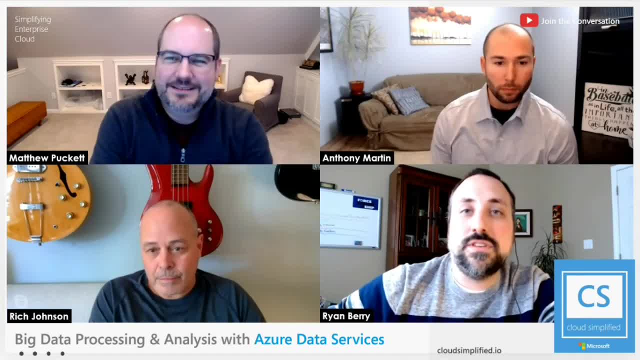 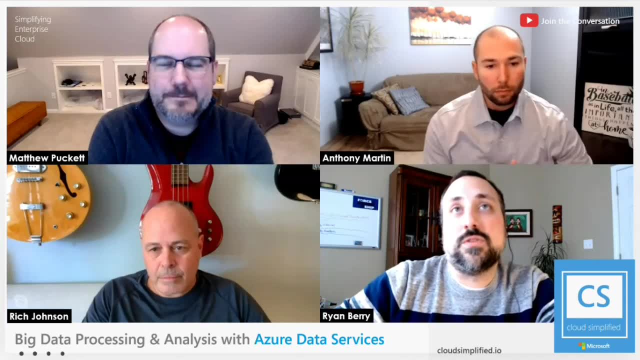 Exactly Okay. So let's jump into a little bit about what you guys did. You know we talked about, you know, a large amount of data, certainly Yeah. Were there other solutions that they had explored, and were they using Hadoop before? 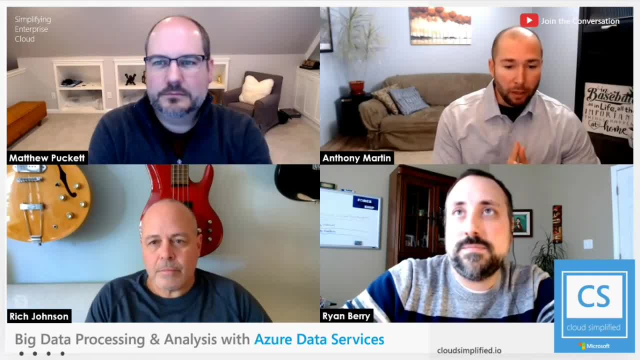 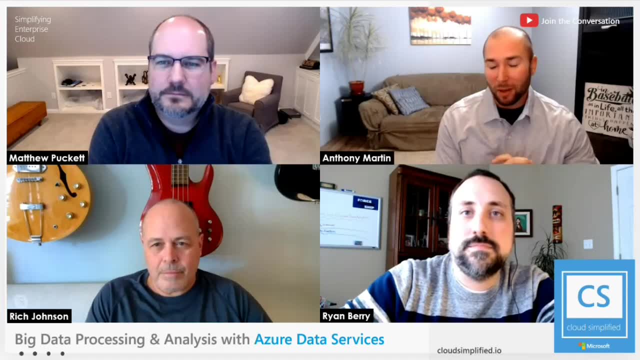 They were. so they did have an HDInsight cluster and, believe it or not, the CIO of this company had kind of gotten hands-on and was doing some of that work and you know they ran into some of the challenges in terms of performance, learning, curve, experience with the solution. 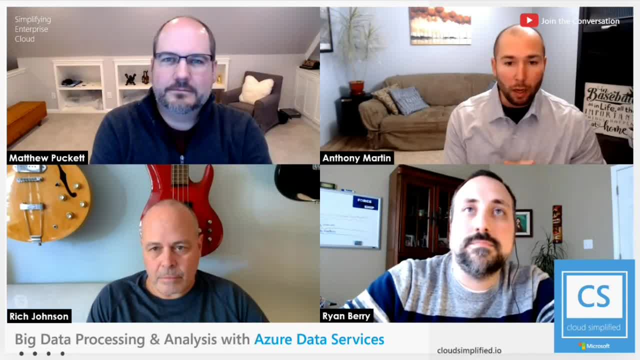 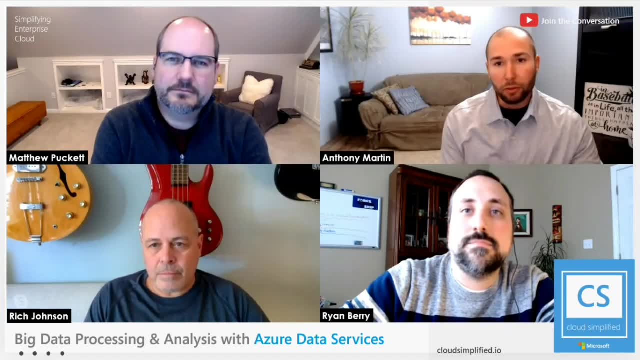 or an expert in the technology and they were looking for something to process it a bit faster. They had a lower, more cost-effective rate and they also had the need for a lot of different users inside the organization to collaborate on the end solution, to get insights out of. 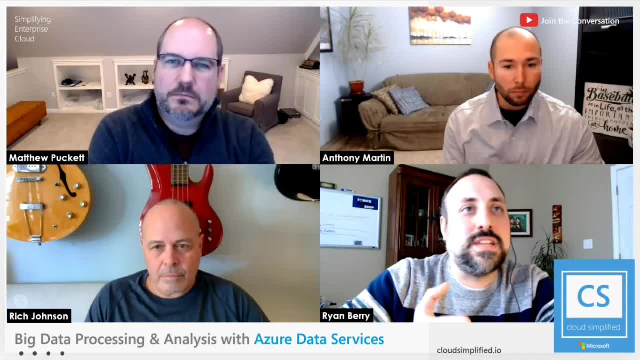 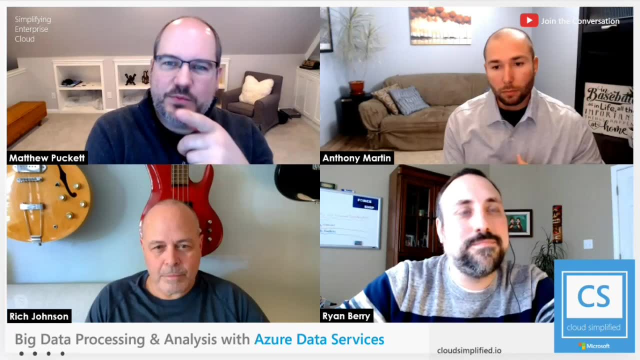 that data. Okay, Go ahead, Matthew. Oh, no, I just- I think that's one of the other challenges- is just not the data volume that comes in. A lot of times it's just now. you have to democratize the data. you know, that's kind of the buzzword. 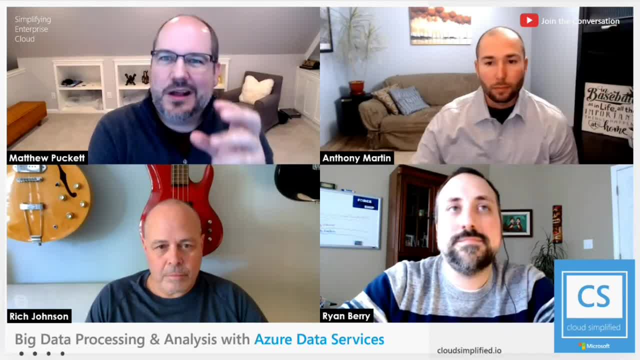 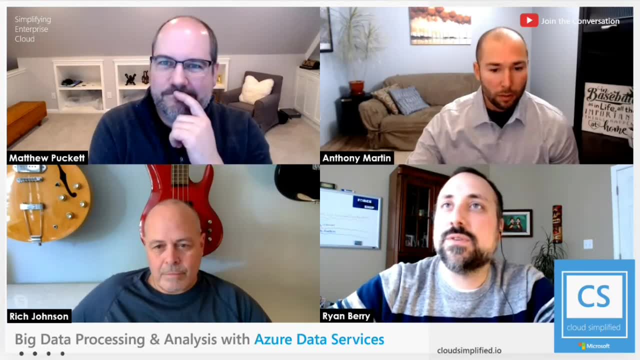 that's going around, right, Yeah, And when they get inside these really expensive, very complex data systems, they don't get democratized, right, Yeah, Yeah, Yeah, All right. So let's go ahead, and I think you had some slides that you're going to kind of walk through. 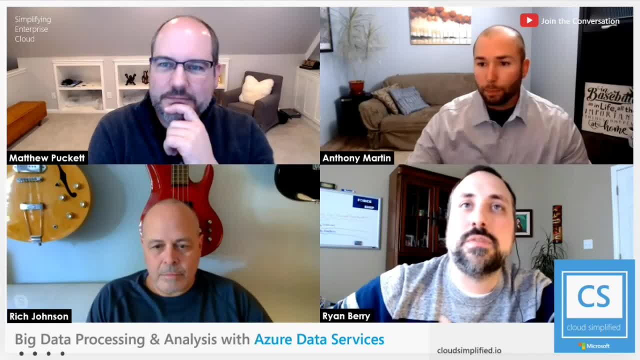 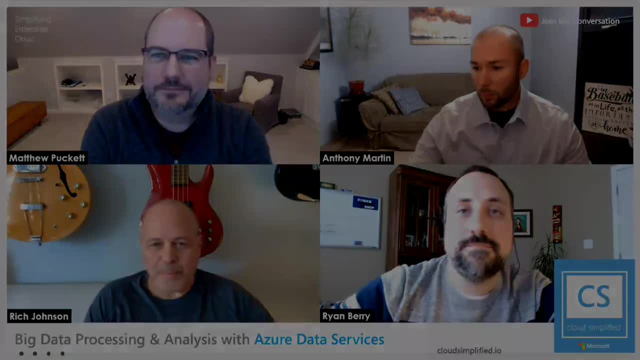 to get us kicked off and talk about, you know, kind of explain what you guys accomplished and what you started with, and then we'll jump into some demos. Great Okay, All right, So we were able to show our slide deck here, so this is kind of the generic case study. 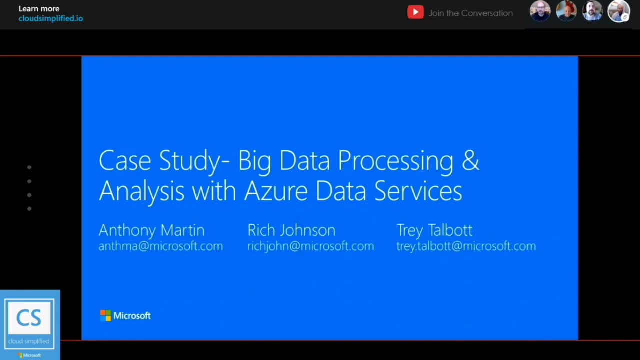 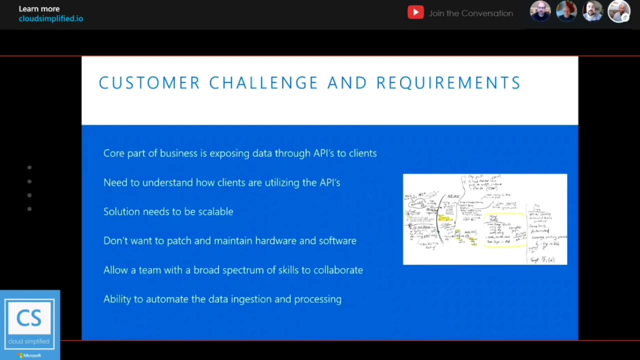 of how we did big data processing analysis in Azure using some different data services and Databricks. Okay, All right, So we talked through. you know what was the customer challenge, the requirements. what are we trying to talk about here? and we do have a little bit of a screenshot of. 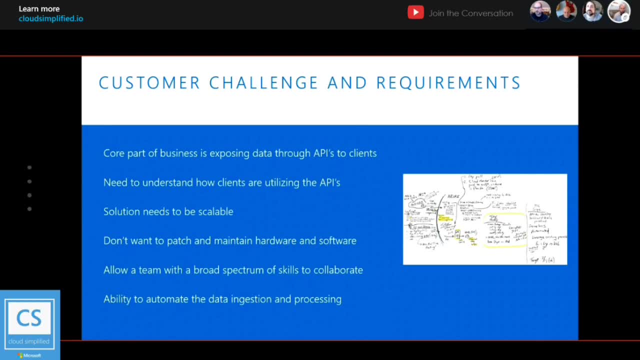 some early whiteboarding sessions as we were working through this. but really a core part of the client's business here is exposing data through APIs to their clients And that's as we talked about. there's significant usage: over 40 billion API calls per day. 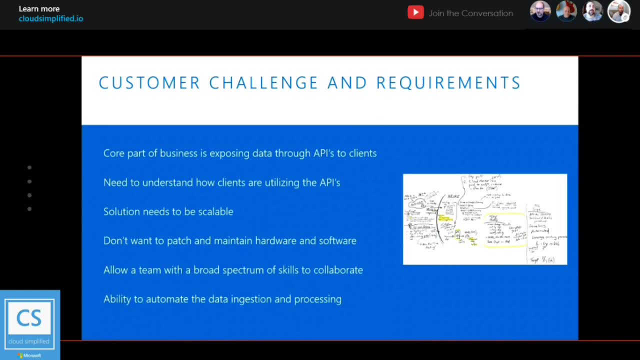 which is generating that volume of data that we talked about. This is generating revenue for the client. Okay, So it's really important to have some sort of caching layer in terms of how do you expose this API to clients? So they expose their APIs through a CDN provider, and that CDN provider is Akamai. 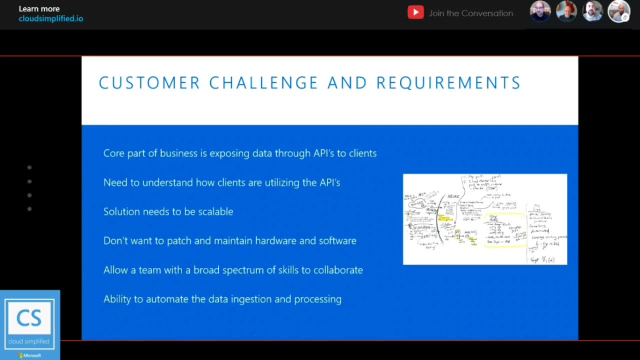 And that's because when you have that many requests coming through, you don't just want that hitting your particular on-premises or cloud-based data store. You need it where your end users are, so they use a CDN for that. So this is weather data. 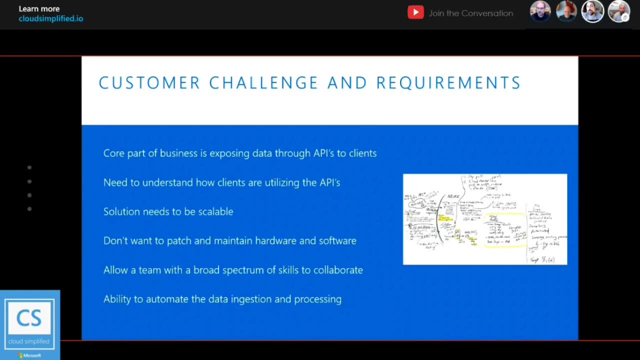 I'm looking for weather information for my Zipf. Okay, So I'm looking for weather data for my Zipf code. It doesn't make sense for somebody sitting right next to me who also is interested in weather data for my Zipf code to hit the database hot. so that's where the caching layer can. 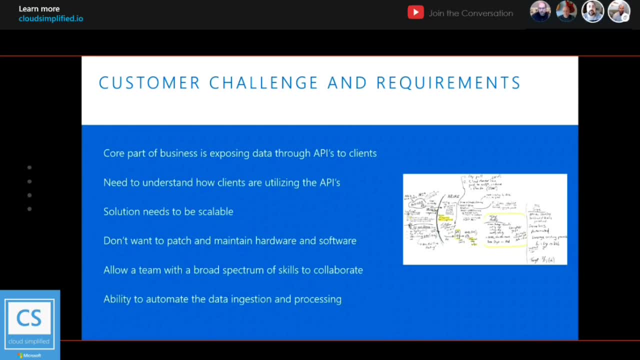 come into play. right, Exactly. And if you think about that weather app that you have, you're looking at, hey, what's my forecast today? What's the next five, What's the next seven? Right, I'm going to check different locations where I might be traveling, so that sort of behavior. 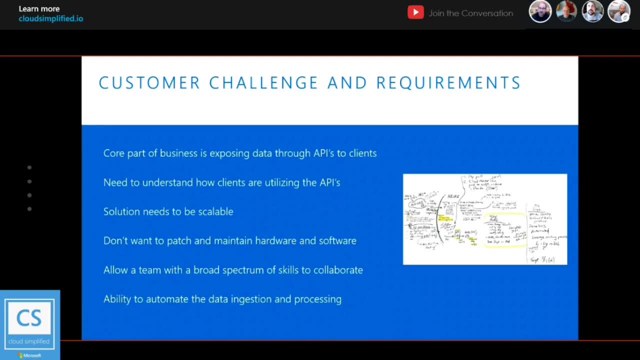 Okay, Yeah, And so you said the customers are already making money on this, right? Have you guys done an assessment of what kind of- Yeah, What kind of a return of investment kind of forecast is? Is it a year two? 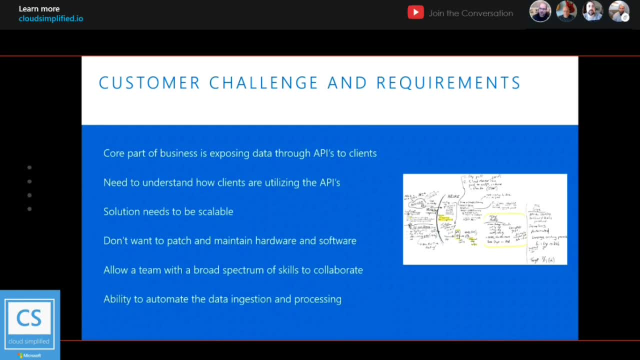 You know, how quick did they come back with monetizable value here? That's a great question, but we have not made it to that point, Not yet. Okay, That's fine. That's fine. You said money. I woke up and I was like, oh, free money. 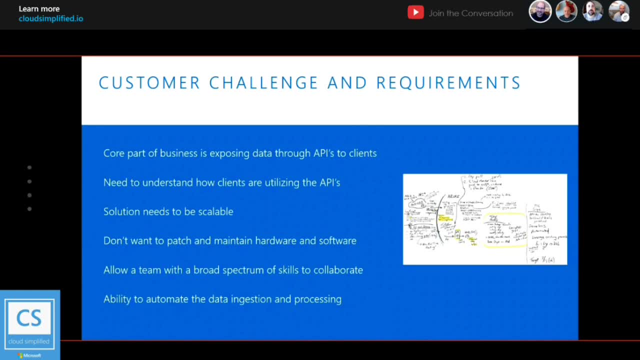 But it wasn't Some of those commercial clients. based on the amount of hits on that API, they're able to monetize it. so that's kind of the thinking there: Okay, Okay, No, No. So because of all that, and if you think through it, if it's not hitting your infrastructure, 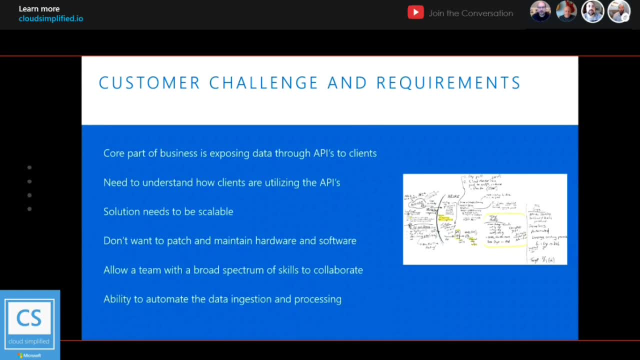 how do you know how clients are utilizing your API? So you really need to understand that is so. in terms of what sort of trends, what times of days are the most frequency? how can we combine this data with actual weather to understand client usage patterns? 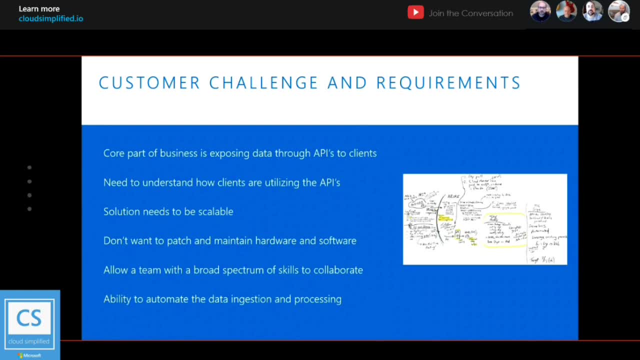 Are they only checking when they think storms are coming, and so on? Is there abuse of the APIs happening from different- I mean from different- cell phone providers or technology providers? So all that sort of information to understand and gain insights from how the APIs are utilized. 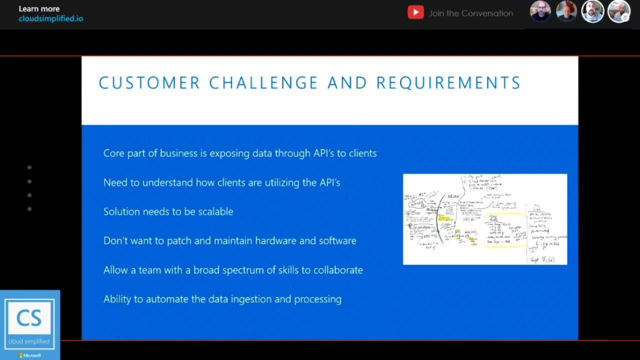 helps them make business decisions. Okay, And I see some other bullets highlighted here that we already talked about Not wanting to patch and maintain hardware and software. that's the Hadoop path that, like I said, is perfectly valid and viable, but that was a problem they wanted, or a challenge. 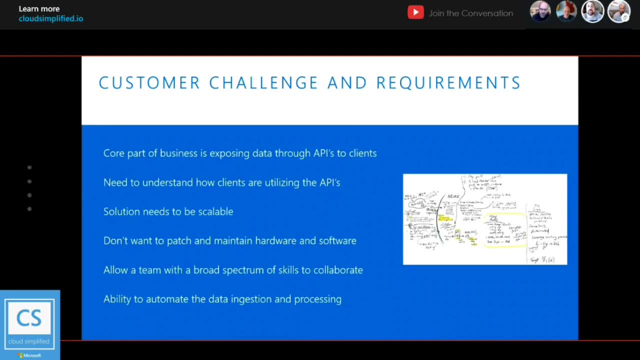 they wanted to overcome in this solution, Right, In this customer's case, Exactly, Yeah, Okay, The solution needed to be scalable, not only in terms of data, which it's growing and growing over time, but the different types of data processing they wanted to do. 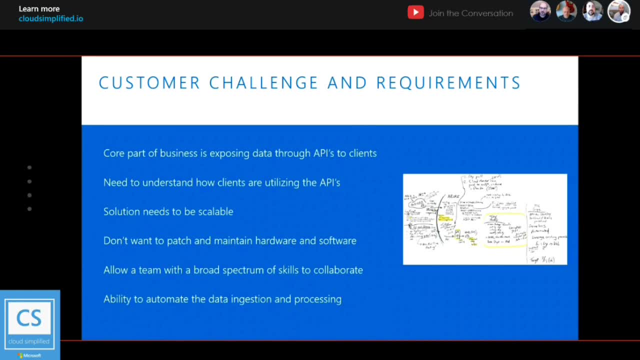 So if they wanted to do, let's say, batch processing today, so they want to operate, maybe they'll run this on some sort of nightly frequency or run it on a certain time of day, If down the road they decide, hey, we want to do this more of a stream processing solution. 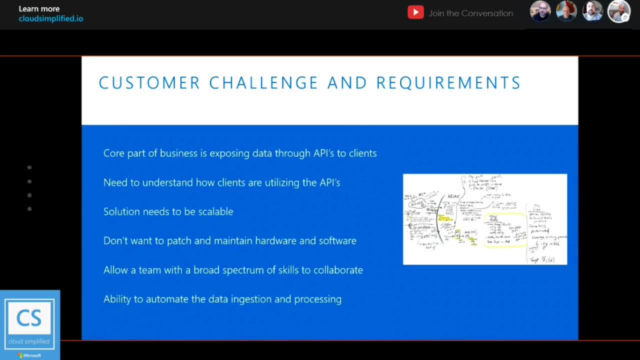 or if we want to add some machine learning on top of that data. they didn't necessarily want to Throw apart the solution or add different pieces and parts. They wanted something that was going to scale in terms of data and the different types of data processing they could perform on that data. 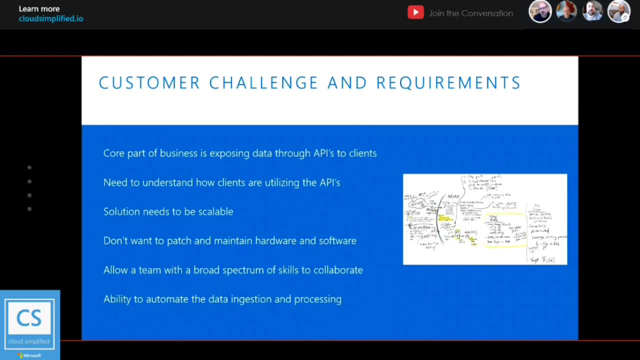 Okay. So did you guys share then how long it took from conception to pilot? We didn't share that. We haven't talked about that yet. Rich, do you recall the timeframe? I would say, and it wasn't a full-time effort, Anthony, on my part, but I would say from: 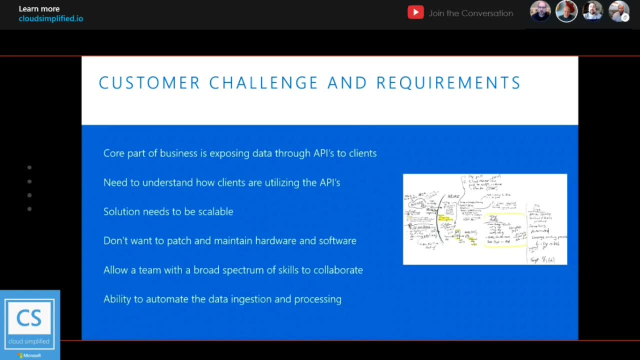 the concept, what they're trying to do, to moving data around to things like Azure Data Lake Store and then actually getting some reports and significant queries out there. probably a three-week period, Holy cow, Okay, Oh, what, Wow, Three weeks. 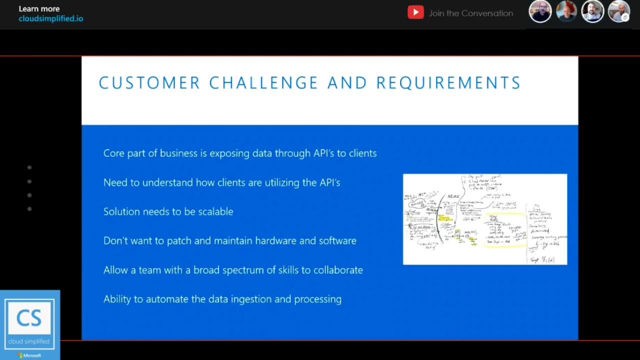 I thought you were going to say three months. I was like, oh yeah, that sounds pretty decent, pretty average, but three weeks, That's fast. Wow, That is fast Okay. And we were surprised, like I said, kind of on the ramp up and learning curve, both being 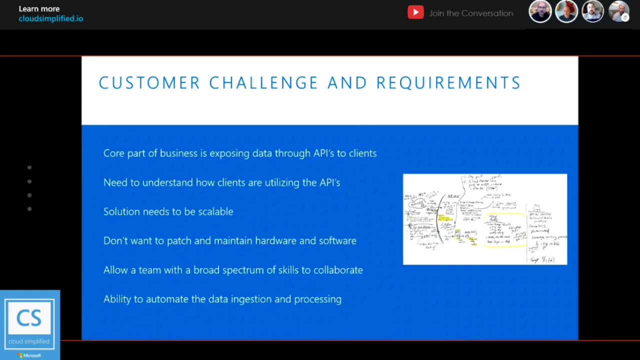 brand new to Databricks, so quite a week. Yeah, I wanted to put in a comparison for another customer. I'm working or helping right now with some plant floor-related solutions and we talked to them about Databricks two weeks back and did a very high-level overview for the customer and talked to them about a week. 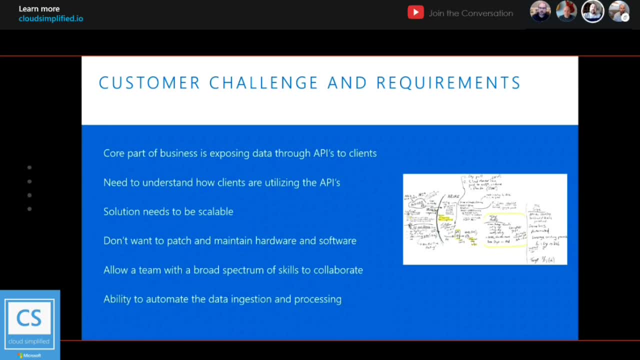 and a half after we spoke to them and they were able to get up and running themselves and moving data into it. We had expected to go in there and have to do a lot of hand-holding But you know they had some technical expertise so we were able to rapidly mobilize around. 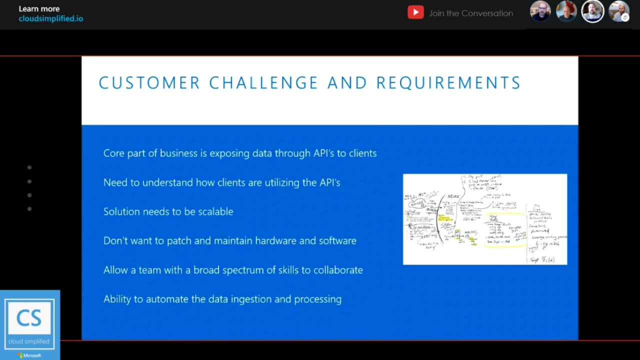 Databricks and you know they've got, you know, millions of records going into it already. I don't know how your regions are, but it's very difficult to get an actual Databricks architect or someone to work with. 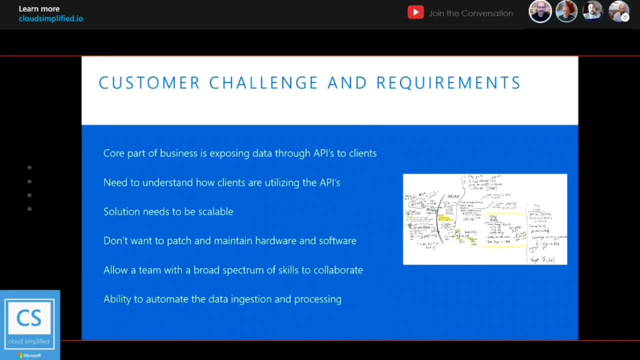 Those guys are so busy. Just about every customer I know in our region is either taking a hire or doing something significant with Databricks, so it's a good testament to how useful and powerful a tool is. Cool, Okay, Yeah, carry on. 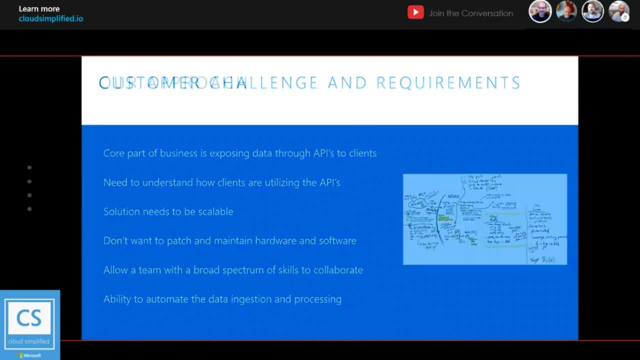 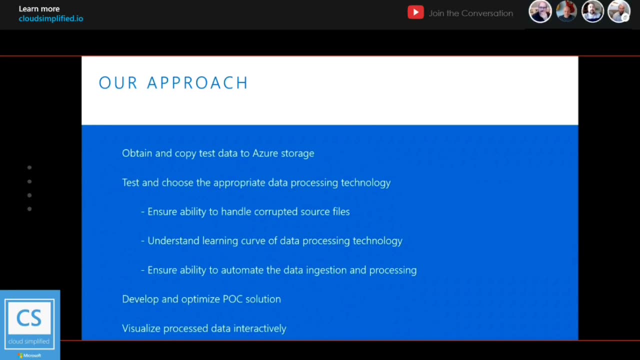 I don't want to derail or interrupt, but just wanted to kind of throw that tidbit in there. I'm pleasantly surprised with kind of the rapid development capabilities of it as well. Oh yeah, Yeah. So that's a good segue. 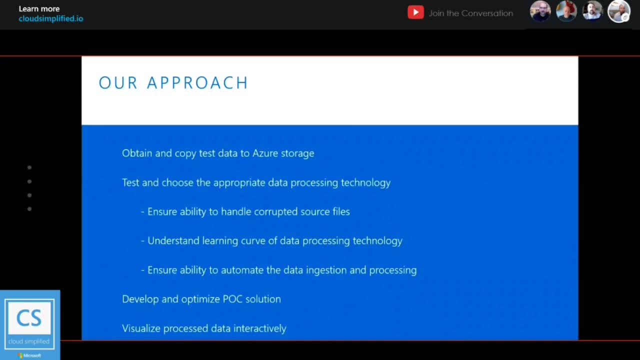 So let's talk through what our approach for this POC looked like. So the first thing that we wanted to understand was: what does this data actually look like? So we worked with the client, We got a sample, some sample test data, and we loaded that to Azure Storage. 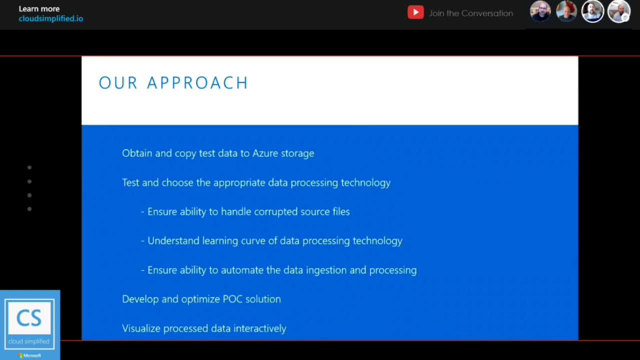 You know, as we kind of mentioned, we weren't too concerned with the storage. We didn't have a lot of data processing mechanisms, but there's lots of different data processing technologies to potentially work through in the Azure ecosystem. Rich and I kind of picked a couple that seemed the most appropriate and we kind of divided. 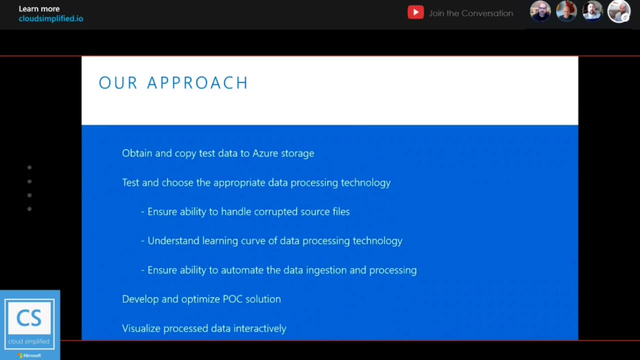 and conquered here. So we tried a couple of different things out and ultimately we decided based on some of these requirements that they had here. so they needed to be able to handle corrupt source files. A lot of times, from you know their CDN provider, they get some corrupt files. 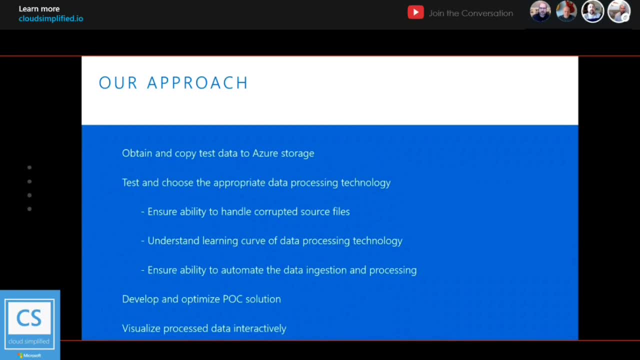 That's just happened, So we wanted to make sure that we could work through that pretty seamlessly. The learning curve was another big piece that we've talked about already. They need to be able to pick it up quickly. We couldn't just take a long period of time and have someone that's really worked with. 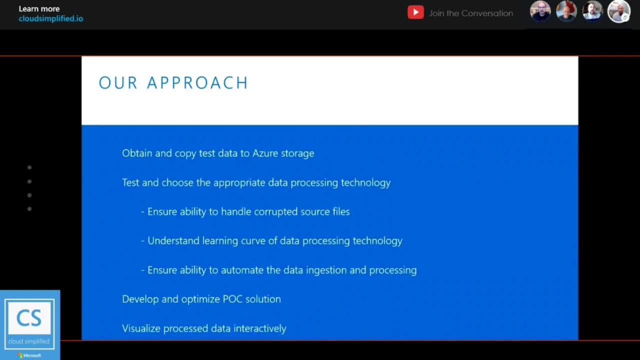 the technology for a long time to pick this up and work with it, And they also needed to, of course, it needed to be automated. They didn't want just someone that would spin up the cluster clicking buttons through the portal. They needed to automate it, schedule it so that they could focus on their business. 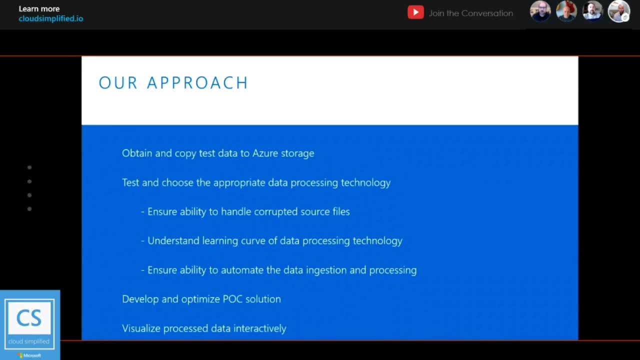 So once we kind of divided and conquered, we pretty quickly saw the Databricks looked very promising And that was. we showed it to the client. they liked what they saw and then we kind of utilized that as the service that we were going to work with going forward. 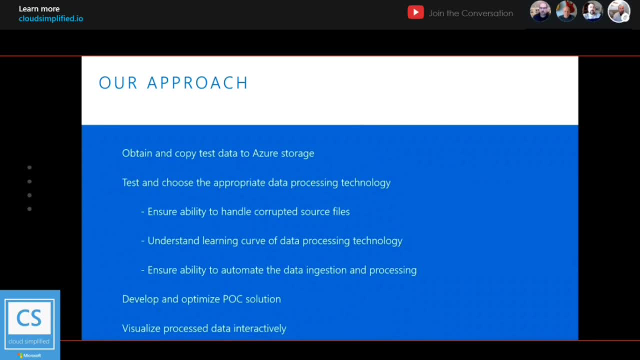 So then, Rich and I kind of then came together, We flushed out the rest of what the POC solution would look like with Databricks, And then finally, we added some visualization technology, So not only could we work with the data and process it and get the correct formats that 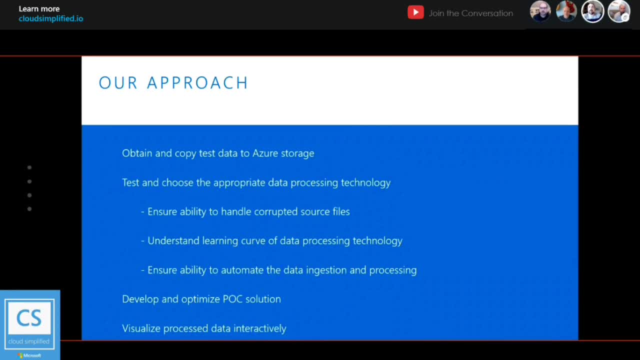 we wanted. how can we start to visualize and gain some insights from that data as well? I got a question for you. So, other than the source files potentially being corrupted and whatnot, Did you guys have to worry about any data scrubbing data- I don't know the word- integrity? 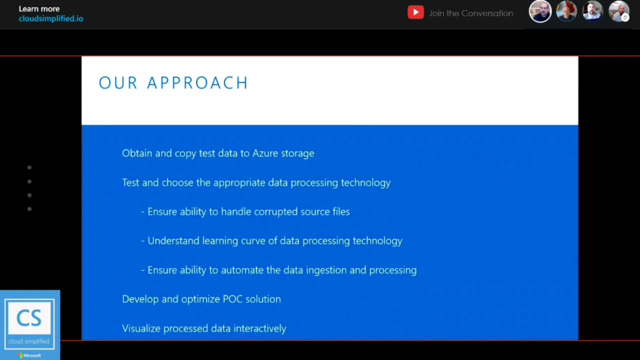 but really kind of just kind of, the data's clean, it's not bad data. it was good data for most of these sources, Or did you guys pretty much already kind of walk into a really nice green field and it's pretty sterile and a lot of data is pretty intact, other than maybe some corruption along. 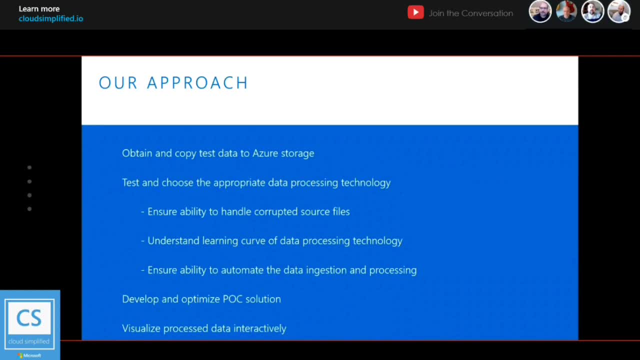 the way Outside of the corruption there wasn't. we didn't come across any issues with bad data per se, but the data did need to be broken apart And we'll see a little bit of the demo, because when you're accessing APIs, the query string 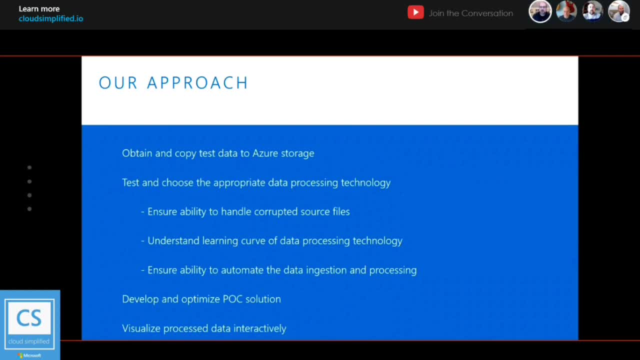 that comes across is has a lot of. they jam a lot of information into like a single. understand the different pieces and parts of the API that are being hit and what are the parameters that end users are supplying to it. required some manipulation to report on it. 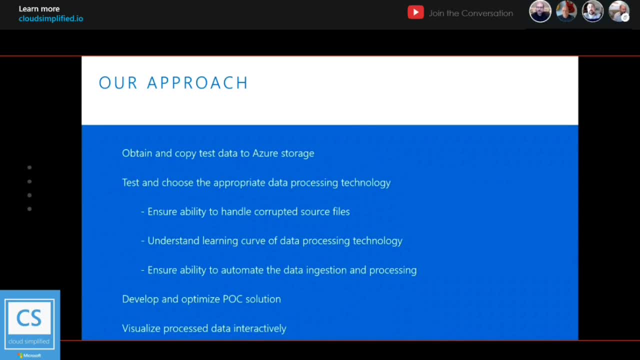 Okay, I got you And the further understanding. I mean, obviously they're ingesting data as well. Is that the case here? that they're getting data from vendors or, Yeah, Other, you know other- weather sources and so forth that they're aggregating? 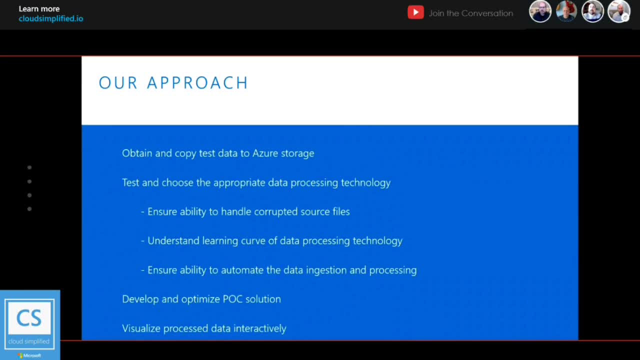 Is that? is that what's feeding? So there is different pieces of the organization that get weather and data from other third parties. Okay, But this piece was really. Hey, we have these CDN log files on how I, Okay, Okay. 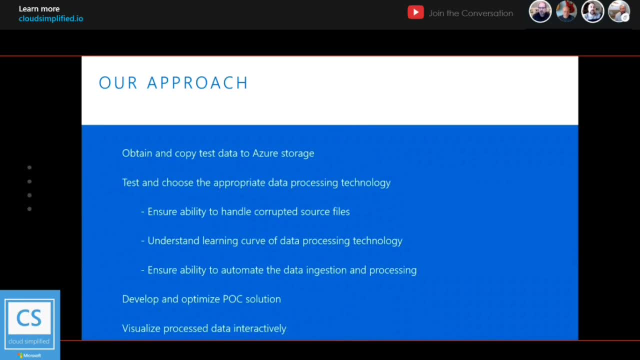 Got it Okay, Yeah, So it's coming from that, Okay, I see, I see. Okay, Of course, there's definitely some benefits for potentially combining it with other data that they're looking at now. Okay, I just wanted to kind of understand that that flow. 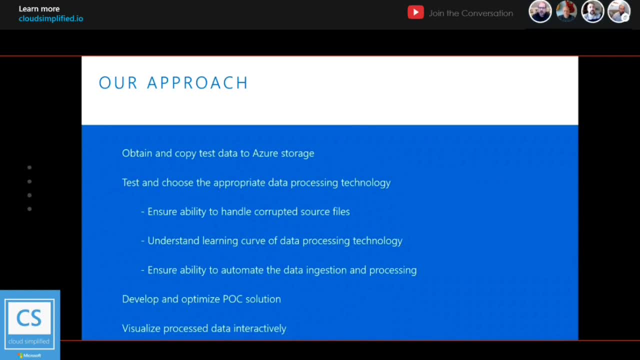 Okay, I got it. How real time was it? How close to real time was it? So ultimately they've initially that they're landing on a daily processing solution. Okay, All right, So at least 24 hours, that's 600 gigs, man. 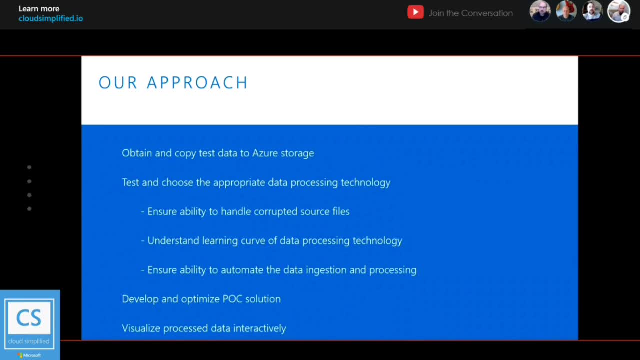 Yeah, Ryan, I don't even think you could work that fast. That's a lot of logs. Yeah, Just a few. Yeah, Okay, All right, I'll be quiet. Sorry for the interruptions. Yeah, Yeah, Yeah. 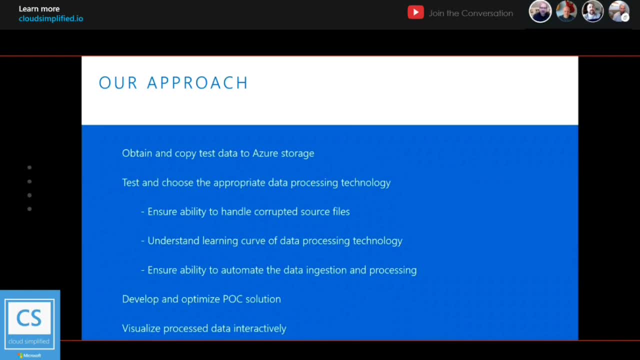 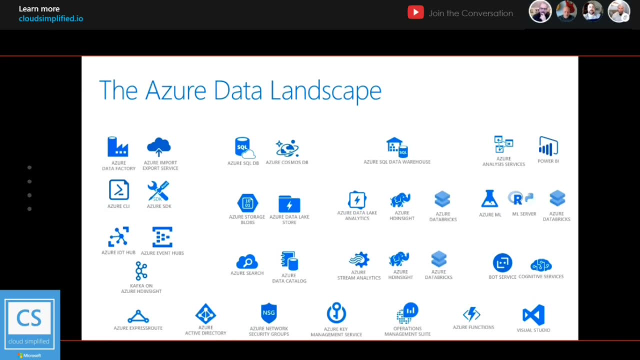 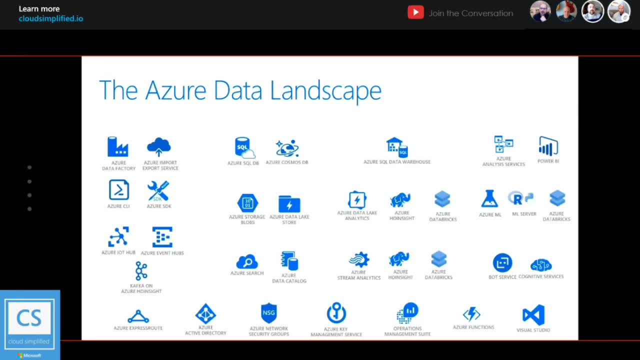 Rich was going to kind of walk through and give an overview of some of the different pieces and components that are available. Okay, So I just going to real quickly. Rich, I see a slide here. Lots of stuff on it. Help me simplify. 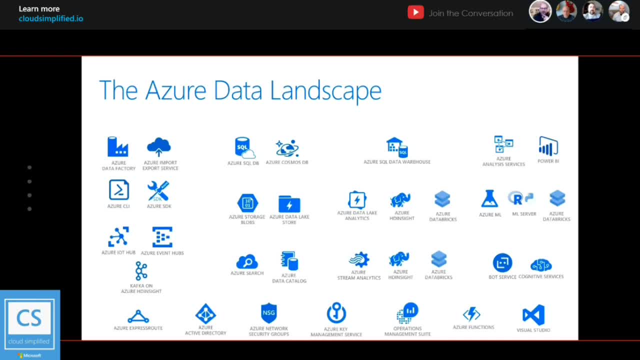 So this: I see a lot of components. so hopefully for the customers that look at this, they don't, they don't. oh my gosh, it's so big. All right, if I had my digital pen work and I'd circle them and simplify them to like. 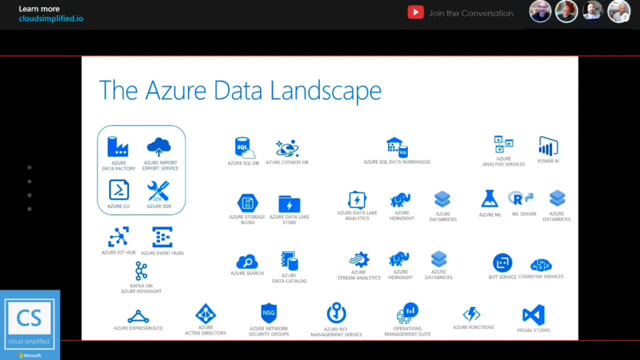 there you go, Okay, Okay. So there you go. So Anthony's already had to be, but you know I've been at Microsoft about 20 years and you know I witnessed the birth of Azure and Microsoft and, like many of us, old timers- 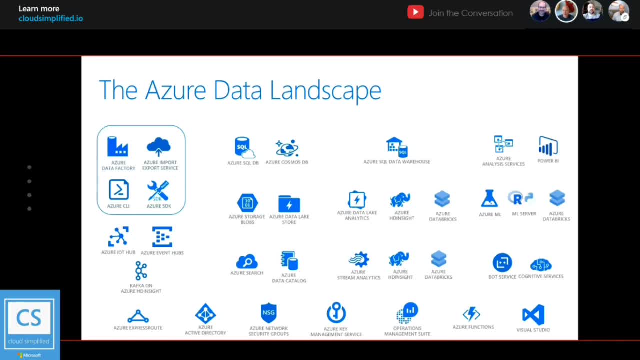 I was a skeptic that this thing really gonna take off as a people are going to give it enough time to mature and take off that it'll actually become something significant, useful. So I've witnessed, I've gone from that whole spectrum of doubt and disbelief. 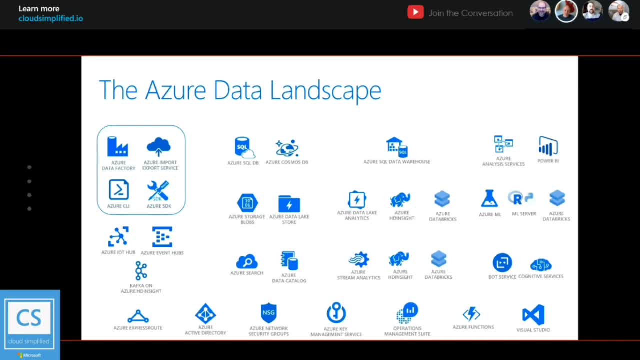 having seen other technologies to the point where definitely a believer And especially when you look over the last few years, the sheer amount of data, services and scale that that's practically limitless for our customer and how quickly we can spin things up versus. I was an old guy. 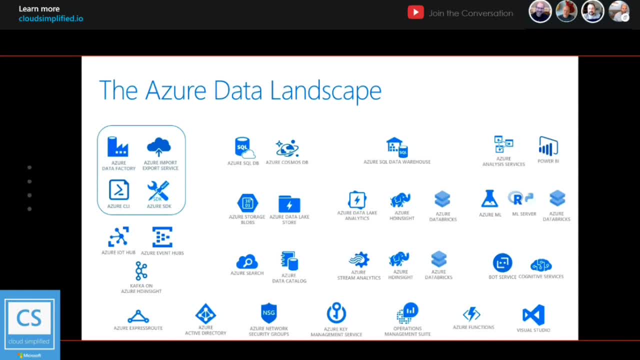 installing racks of servers and I agree You were in diapers about that time- to witness that, how quickly we can spin up. you know, 60 compute nodes on a petabyte of data in minutes versus. Hey, I got to plan this. 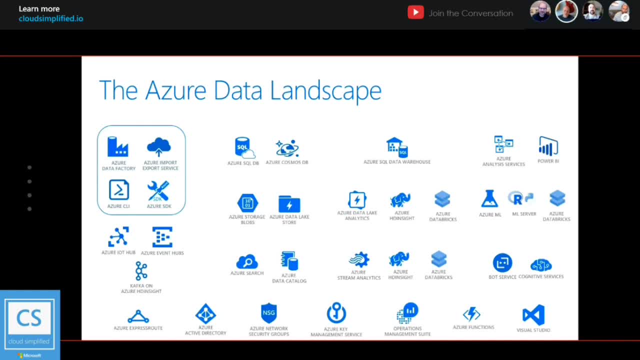 I got to, I got to justify it, I got to get budget for it And maybe six months later you started having hardware arrive in your data center and having room to put it somewhere and enough power to power it. So the fact that this stuff has really taken us this far and we can do things- 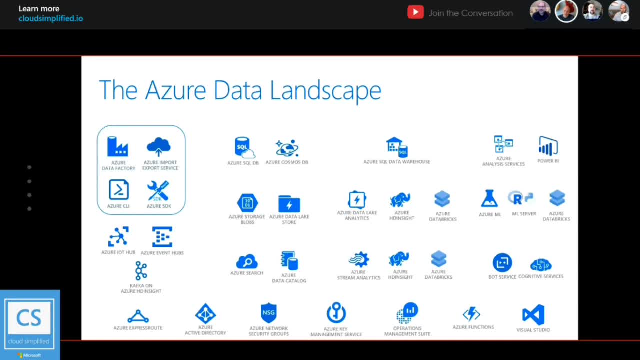 like, like we've been able to do with this little POC for this particular customer is just significant. So definitely a big believer. And, as you guys know, I was working in the same kind of a role here at Microsoft. You just see how quickly now that the snowball has really started rolling. 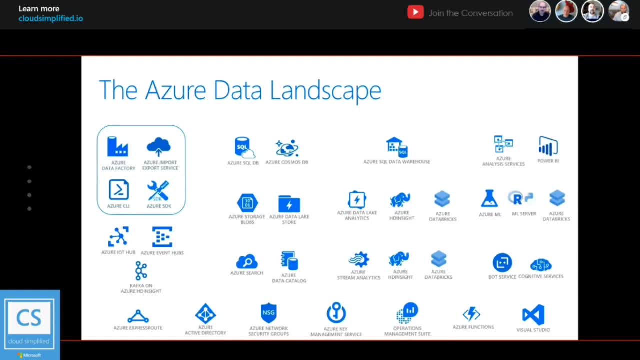 how quickly people are realizing, for large data and analytics, what they can do in the cloud. It's just, it's almost impossible to do in your own data. Yeah, I hear they're looking for a pitch man rich and you know if you're interested. 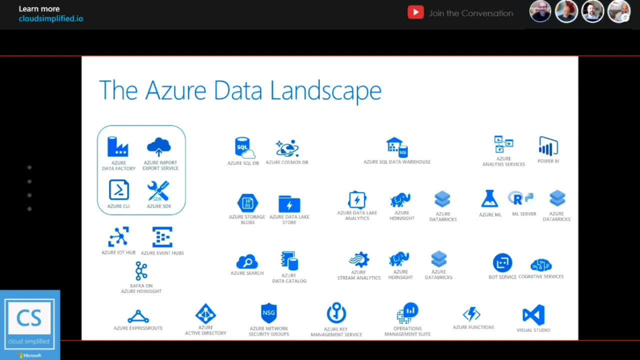 I might be able to make that connection for you. All right, I had to do that day in, day out, but yeah, we do, Don't we? Let's just kind of jump in a slide, So I won't spend it. 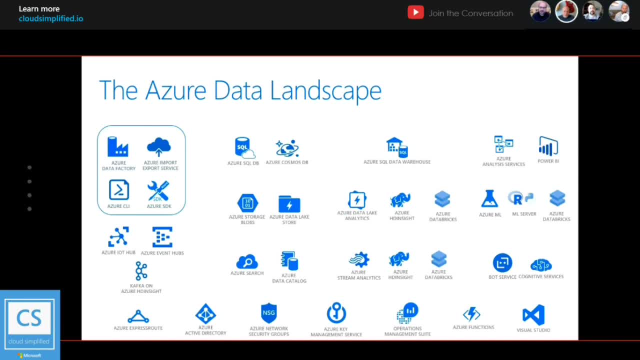 There is a lot. that's kind of a busy slide. but if we look over to the left, you know we have some services for getting data into into Azure or from another cloud provider or wherever- things like data factory or import export services. 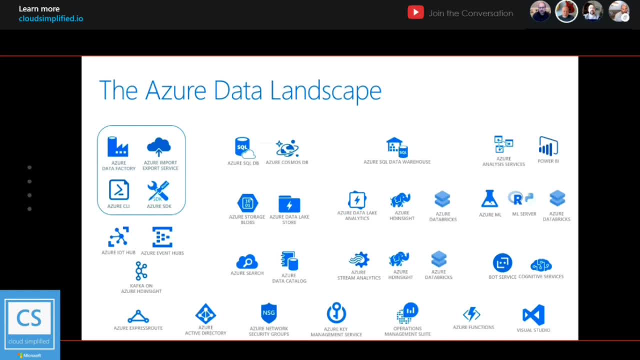 And then even underneath that, some of the IOT type technologies for streaming data on the left, lower, left there. So things like Azure IOT hub and event hub. they provide a means in the in this IOT crazy world where we're. 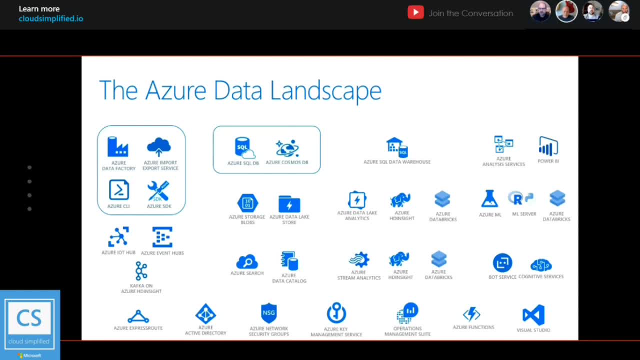 we're. you know, take the example of a manufacturer who's just instrumenting, maybe a 300 ton press, all kinds of sensors and data points that can be gathered off that and streamed in real time as they're manufacturing parts. So we use technologies like that kind of hot path technologies. 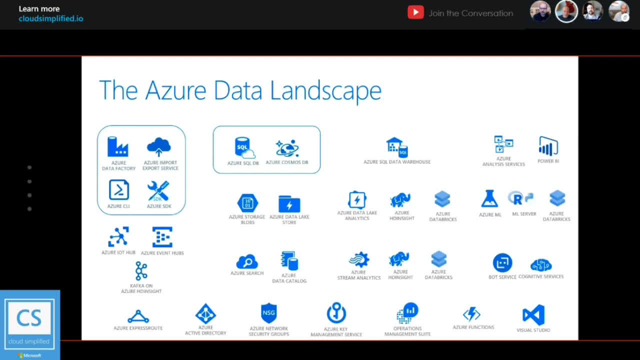 We're can stream live data from a machine into these event hubs and then use services like off to the right here in the center- Azure stream analytics tools that can read that data in real time and then do something with it, push it to storage. 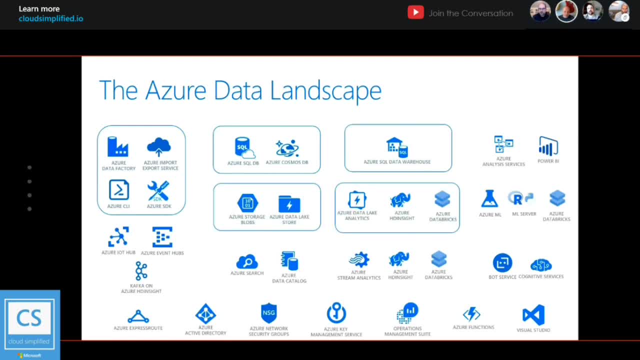 You see some of those you know storage providers. there are services there like Azure storage blobs, Azure data lake store, Azure SQL data warehouse, So they're just a plethora of storage areas Once you receive data or ingest data into the Azure cloud. 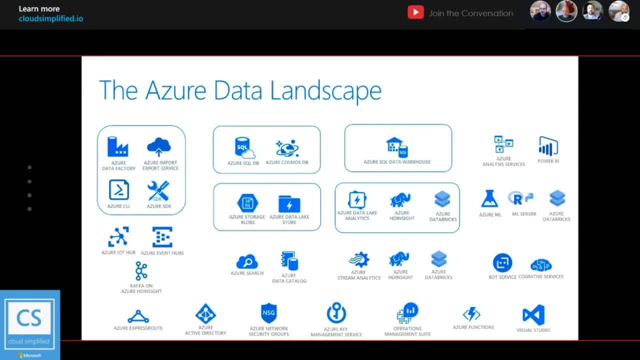 all it means is it provides you a ton of a ton of options to put your data somewhere. And then this notion of- I know you guys have talked about it before and it's just something that can't be understated- This notion of, and separation of, compute from storage means that 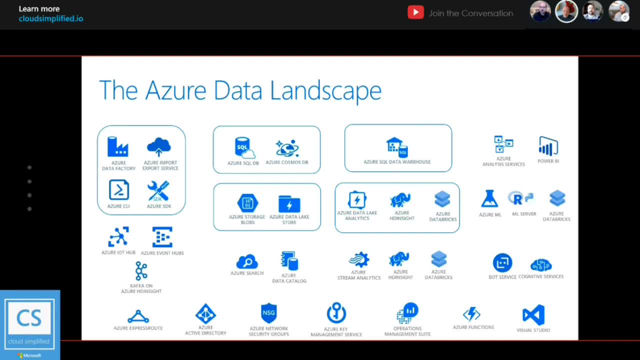 Hey, I don't buy a database and storage and they're all coupled together. If I land on my data right in a data lake store, blob storage, I can bring up different compute engines. It's almost like the database or these data bricks, clusters. 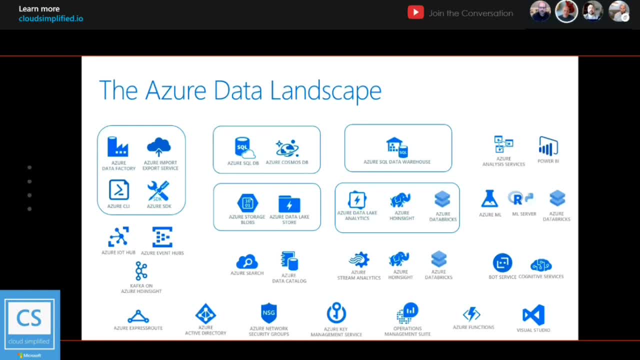 They're just temporary, They're just compute, like programs that we bring up when we need them to do some query or loading work And then we tear them down when we're done with them. And the fact that we can have these multiple services operate in the same. 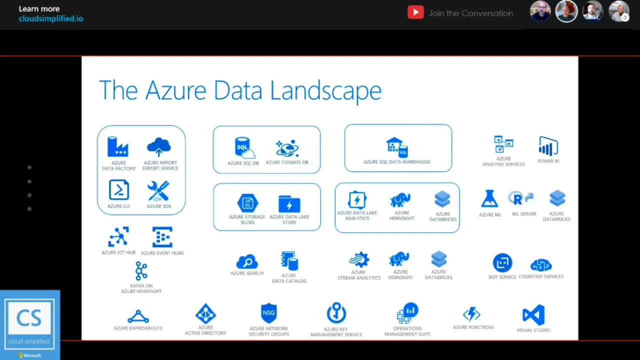 data in one place you know allows us to really have your cake and eat it right. You don't have to be. it's not an either or situation either: or this service or that you know. you can choose what tool or service makes sense for your organization and. 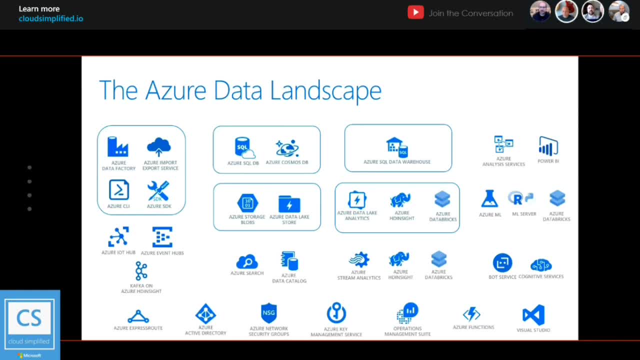 operating that data in one place. So in, in in your customer's case. you know, on the left hand side I'm kind of picturing, you know, the flow from left to right, but that's the ingest path going to a landing zone. 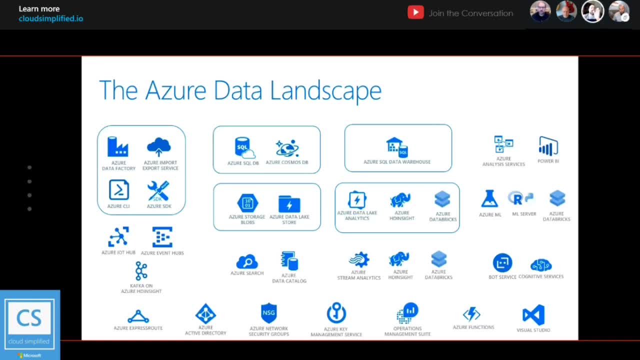 And then the right. you know there's a lot of reporting and analysis options, but so these logs they're coming in via, you know, using something like Azure data factory to actually process these as they're, as they're arriving or being uploaded from the. 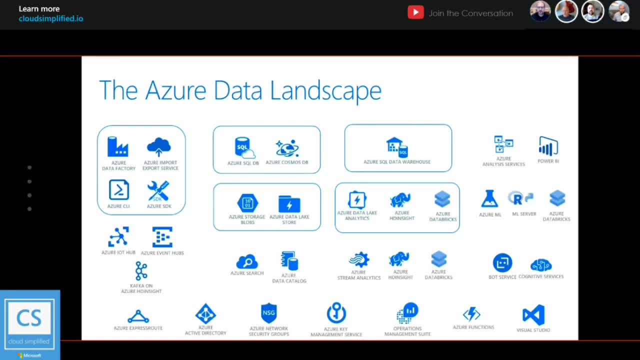 from the CDN Is that. is that what you guys? we didn't use a data factory. We're using a different copy mechanisms, but you may have an update on it. I think this, this particular customer, is now doing a different ingest path to get. 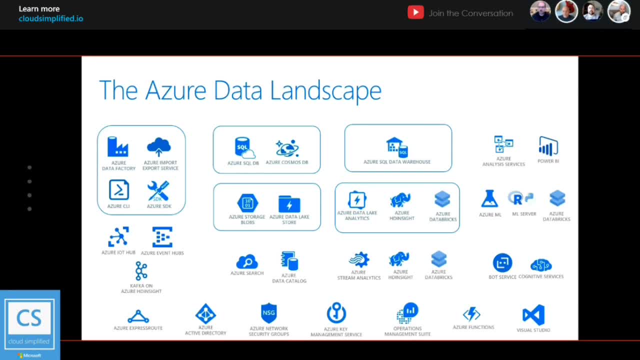 that data into storage, Yep. So they started with just running some, some Python scripts to pull the data from an FTP server provider, to land the data to Azure storage And they're all kind of, at the same time, kind of looking at Azure data factory as well. 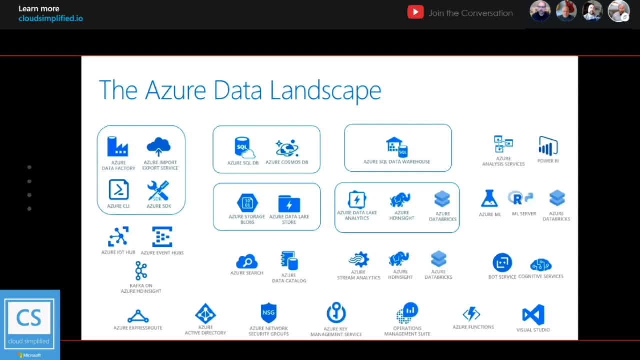 So they're still kind of determining what that ingest service looks like, but they're kind of. they're pretty much swappable in terms of how do you get the data in When you want to kind of orchestrate the end to end pipeline. 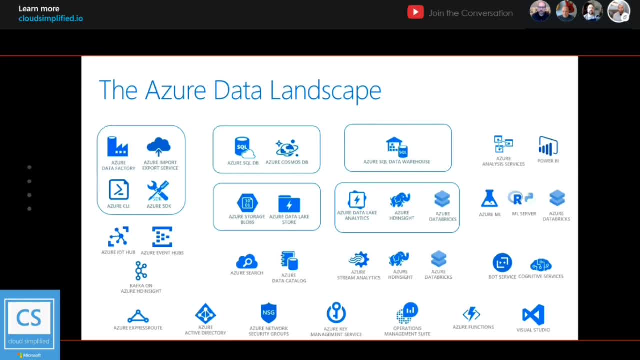 So I want to pull all my data in all these different data files, but now I want to process it and then I want to do something else. That's where Azure data factory has some nice pieces for the orchestration of getting that end to end pipeline. 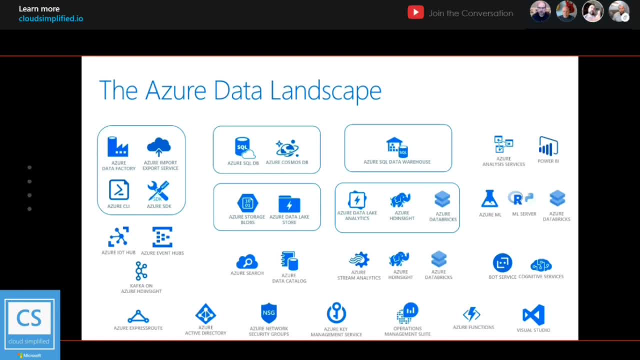 Okay, So so this case they're their vendor, uploading log files, the FTP, to some landing location or some Python scripts that take that, move it into storage And then ultimately you, you end up doing stuff with it And from the analysis and kind of processing side and Databricks. 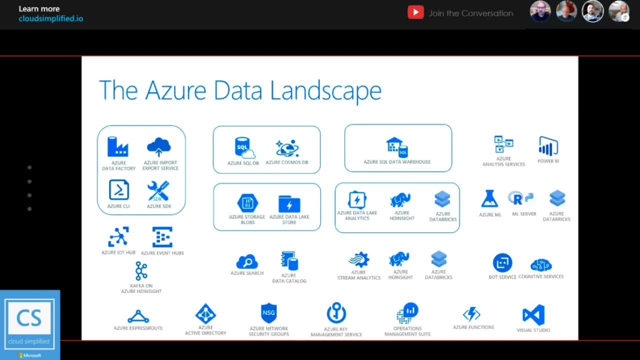 the kind of the the following the red red thread, so to speak. That's the flow. Yeah, Okay, Got it. Okay, Yeah, We'll get you know the next couple of slides. we'll get in a couple of the common common. 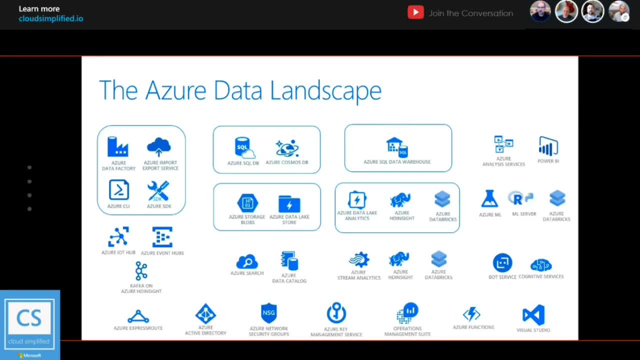 right, Cold and hot path type just to gathering data and making it accessible, And then I'll just quickly finish up in a slide. I mean, like I said, off to the right then. So the center runs, you've landed data. 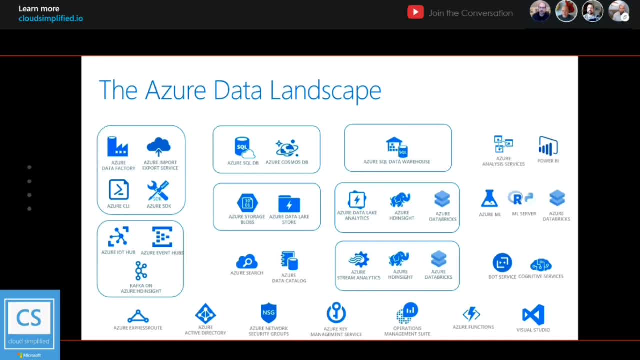 You can do a lot of refinement, uh, aggregation, curation of the data. there. That it's a very common pattern when we're looking at big data. right, We pull in a lot of data sources. It's a lot to handle. 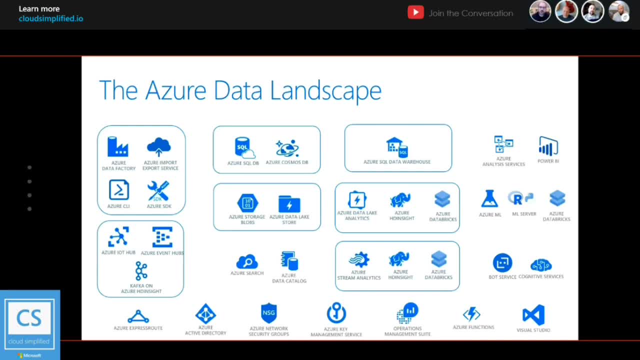 but why don't we really aggregate it or refine it and and shape it into a format that's going to be consumable for different personas or different business segments, perhaps in your organization? So, once we've done a lot of that refinement with these big data, 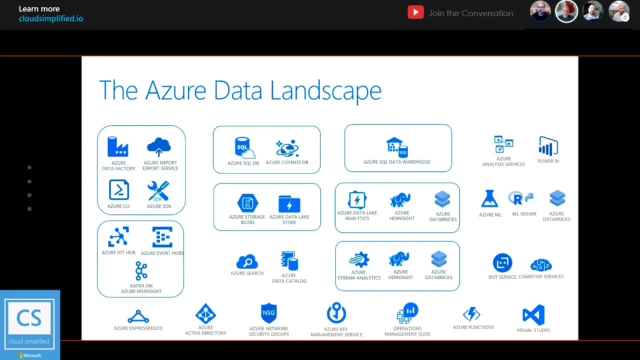 tools like Azure Databricks. right then it may becomes more accessible to reports and dashboards. Like you see, Power BI at the top right and then even the machine learning aspects- very significant how quickly we can take data scientists and allow them to. 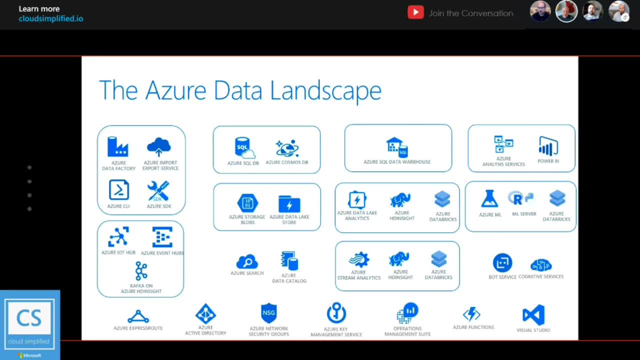 use tools, are familiar with our studio or working in Python, and actually act. you know, push that, push their algorithms or models right onto the Azure Databricks cluster. It's a very pretty short ramp up for them as well, too, instead of just working on a workstation isolated by themselves. 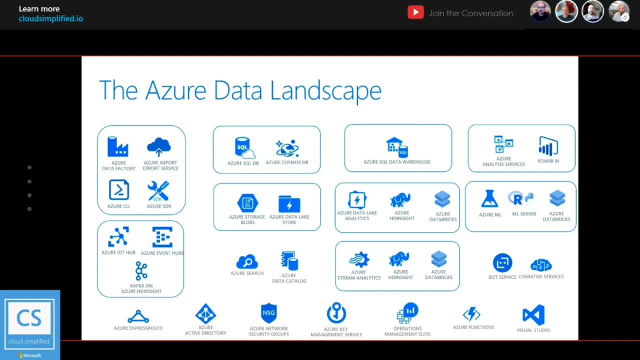 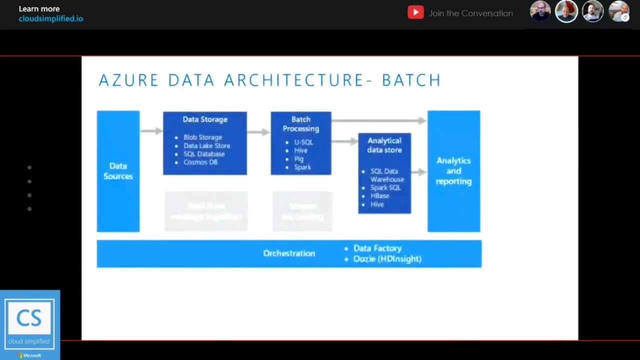 So all this is up in Azure. I mean just, and we'll see some of that and the demonstration parts of, well, how easy that becomes, Okay, So, yeah. so this is a you know, taking that previous slide that I chart on the previous page. 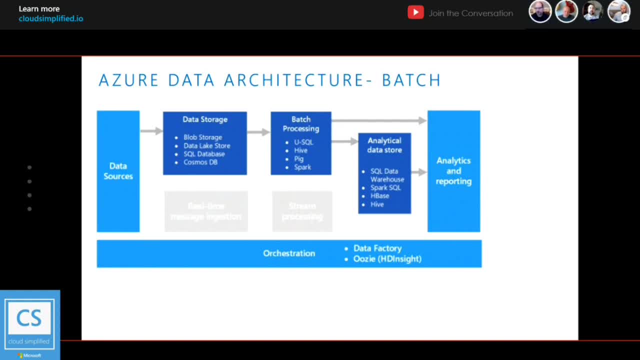 I mean, this is a typical batch architecture where you have a lot of data sources and whatever means you use- maybe it's Azure Data Factory or just a FTP job or whatever- You typically land that data into some type of storage and more and more. 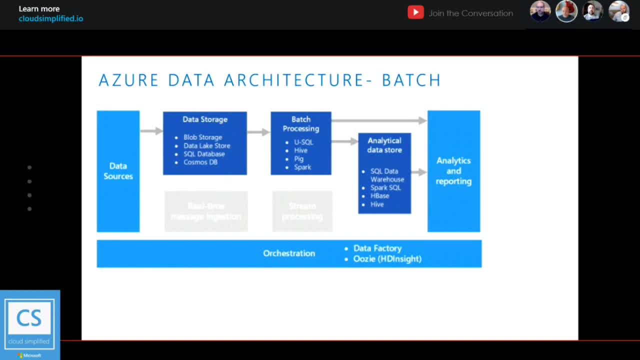 you know, Azure Data Lake Store and Blob Storage are kind of converging in terms of capability And you know we've seen a generation two of Data Lake Storage has come on online recently and it's providing all kinds of new scenarios. 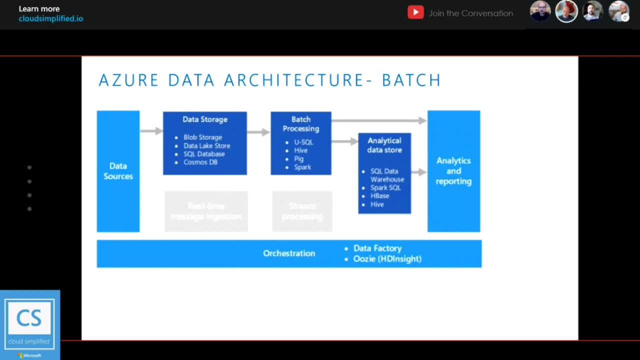 But that seems to be our really that's our future direction and go-to is the Data Lake Store And, of course, on top of that then you can bring different services like Databricks, Spark, our own internal Azure Data Lake Analytics tool called uSQL. 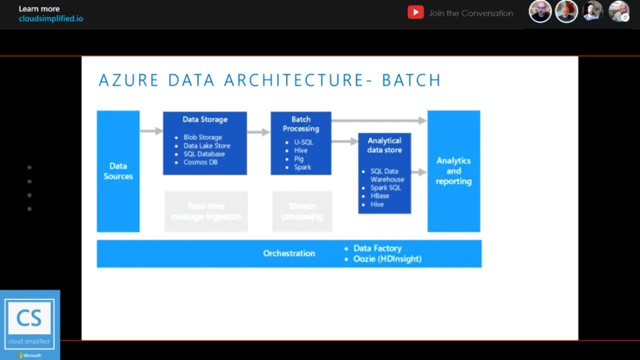 So these different, you know compute engines can operate on this big data and then do something with it, Like I said, maybe refine it or aggregate data and then push it into something like a SQL Data Warehouse service or another HBase cluster. 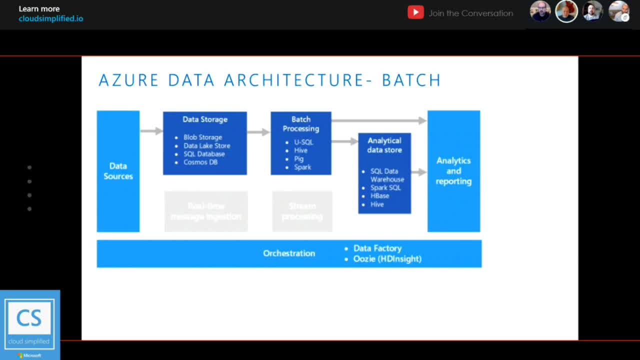 something you provision in Azure and then off to the right provide all kinds of reporting. So this batch architecture, cold path is a typical. something similar we did for this customer right. We were taking that 600 gigabytes of data doing a bunch of batch. 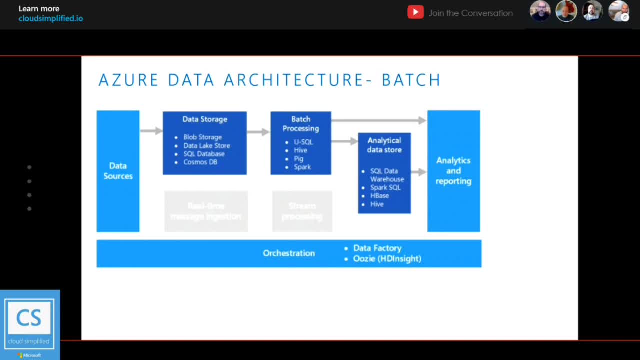 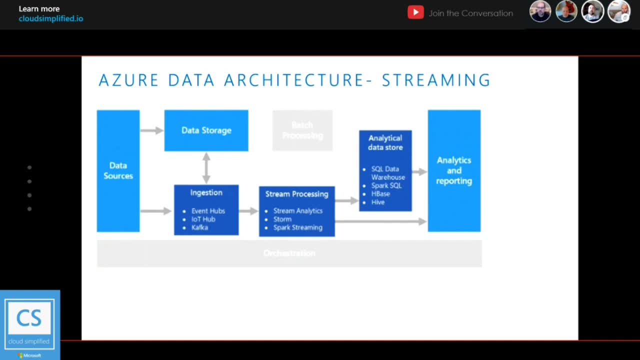 transformation, with it landing it somewhere and then making it more accessible for other types of business intelligence tools. Okay, The next slide is a typical streaming architecture, So you had seen it like down in the bottom ingestion point here: Event Hubs, IoT Hub, Kafka. 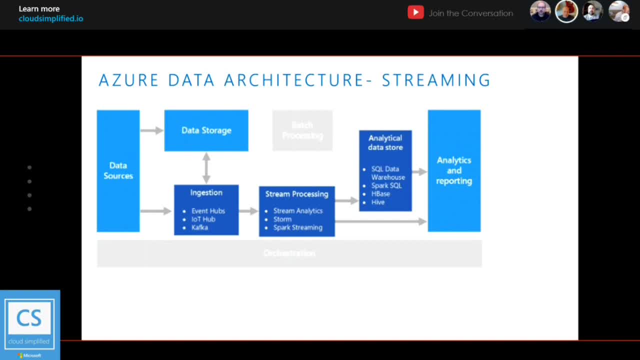 some of the open-source services for large message or event type ingestion. So this provides like a real-time streaming. So we can- we can land data, as I mentioned quickly from things like, maybe in your manufacturing, a PLC or a vibration sensor on a machine or electrical meter on a. 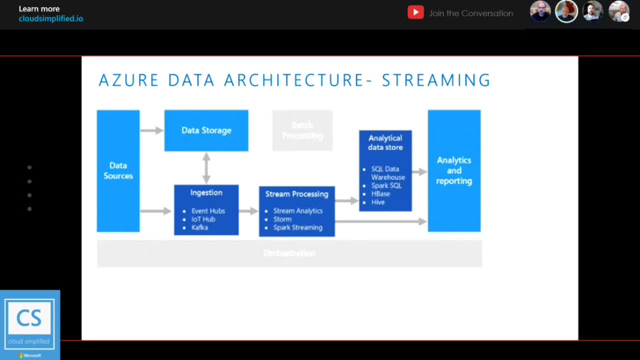 machine. we can capture all those messages in real-time in mass, you know, millions per second- push them into technology like IoT Hub And then from there we can use tools that can stream that data in real-time as well. And the use case we're talking about here. 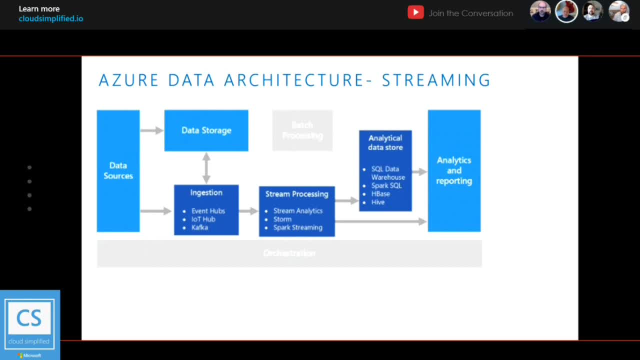 this is probably the ultimate goal is for them to use something like Spark streaming to take this weather data from some of their providers almost in real-time and capture that weather data and Spark stream it into, perhaps a Databricks table that in the same time gets pushed out perhaps to a SQL data warehouse. 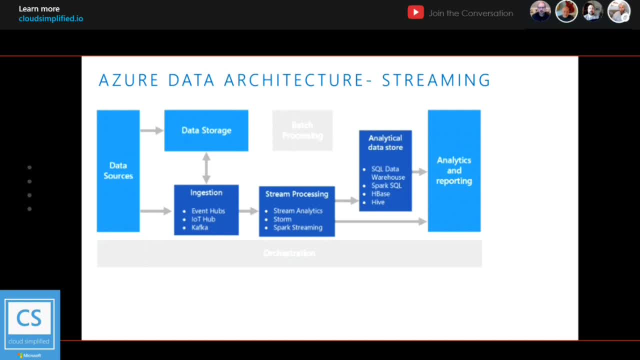 and an analytical data store and then made available for very near or very real-time reporting. Okay, So for this use case, I mean, these are just capabilities in Azure that facilitate streaming in real-time analytics. You mentioned them, exploring this for weather data before processing and 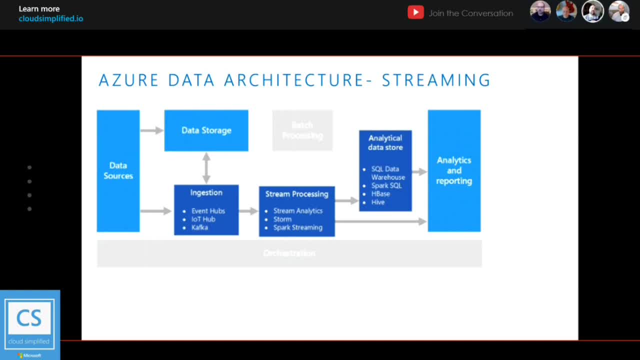 analyzing their logs to be able to make informed decisions about how consumers are using their service. That's kind of more of the previous slide, where you have them batching this data and it's being processed in 24-hour intervals. I think you said right. 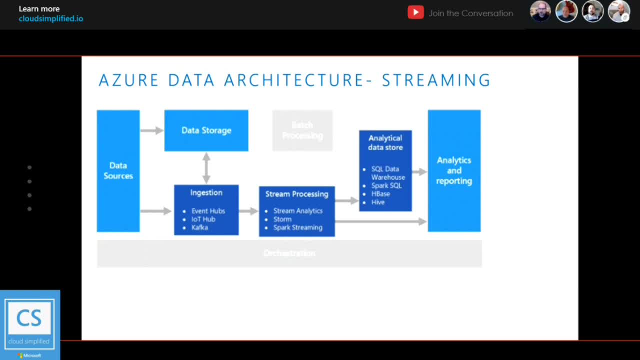 Right, Okay, All right. Well, this would enable new scenarios. right The ability? maybe, if you're a restaurant chain or a customer, you need to know whether, in more or less real-time, that impacts decisions you're making right in the store with preparing food or 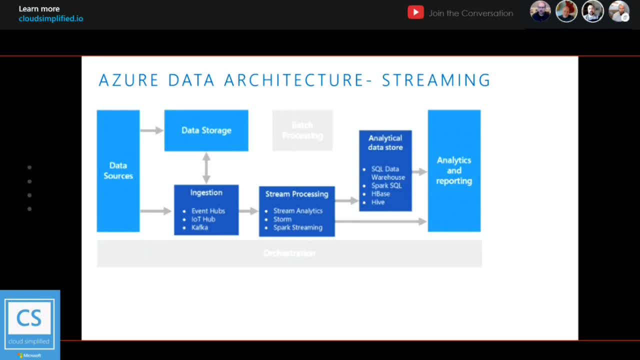 whatever, if you're a restaurant chain or something. So this streaming architecture would allow that up to the second or up to the minute type of processing that when you're making decisions about the data. It could even have a use case around these log files from the CDN provider, right. 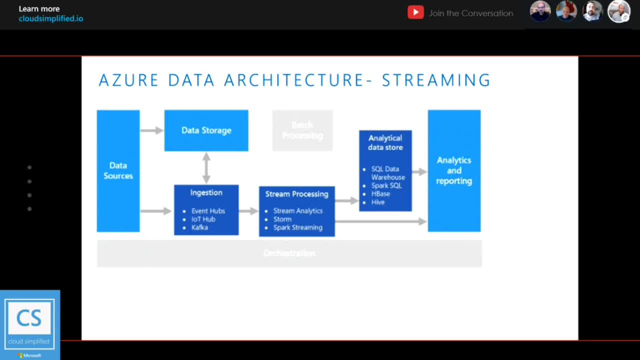 So, hey, if all of a sudden we're processing this and there's a lot fewer number of API calls than we're expecting, hey, what's going on? Is something occurring? Is there an issue? Yeah, that's a good point. 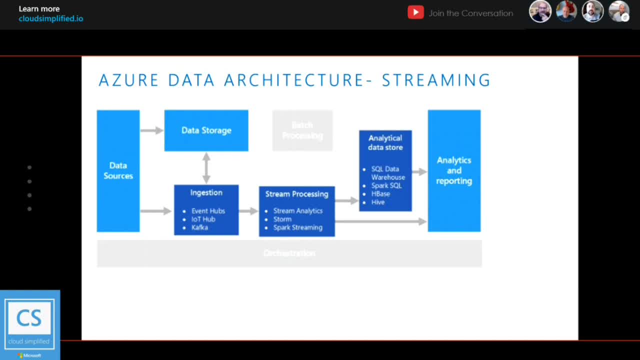 True, true, That's a good point. anomalous behavior analysis: Yeah, maybe something's broken in the platform. Yeah, I think that's often overlooked, as another great value out of data is when things suddenly disappear. People don't think about that often. 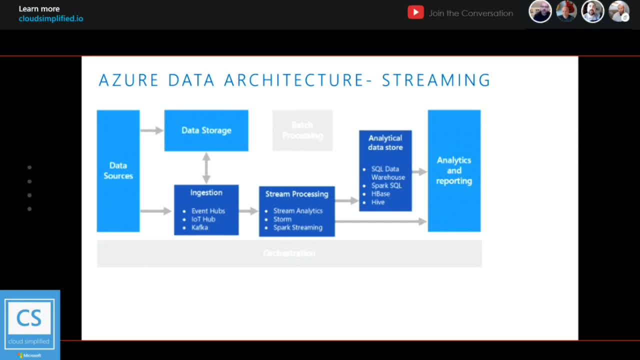 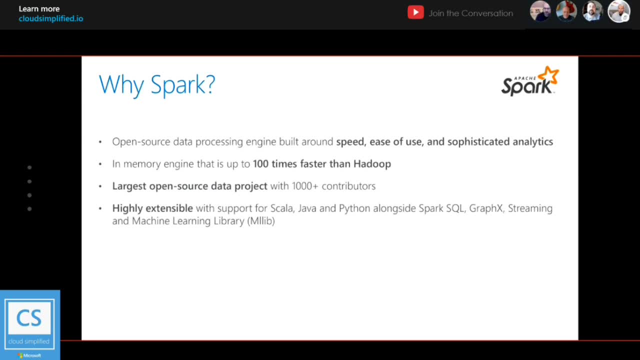 They usually go, what else? but anyway, Yeah, okay, cool, All right. so we've talked about Databricks, but really, what is behind that technology? And it's important to know that Databricks is really a commercialized product offering of the open-source Apache Spark. 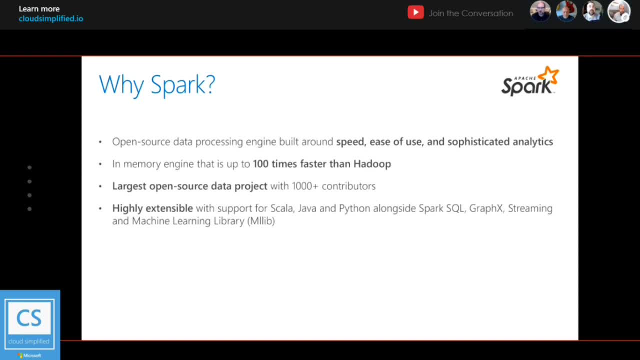 And Apache Spark has really gained a tremendous amount of popularity over the last five years or so. And what it is? it's this distributed data processing engine that really provides some pretty fantastic performance and ease of use. So, to simplify things here, what is a distributed processing engine? 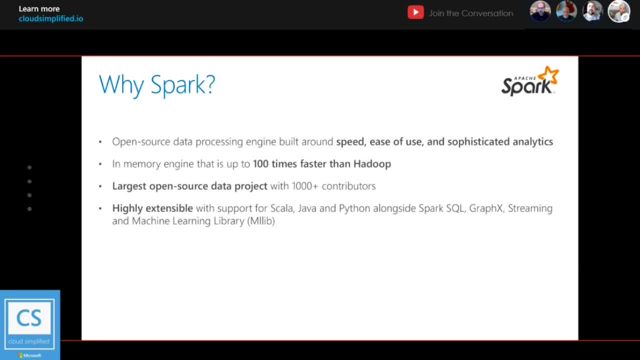 Really it's the idea to take a large amount of work to be done to break that work up amongst different machines in a cluster and different virtual machines in a cluster operate on that data individually and then return that result set to the client. 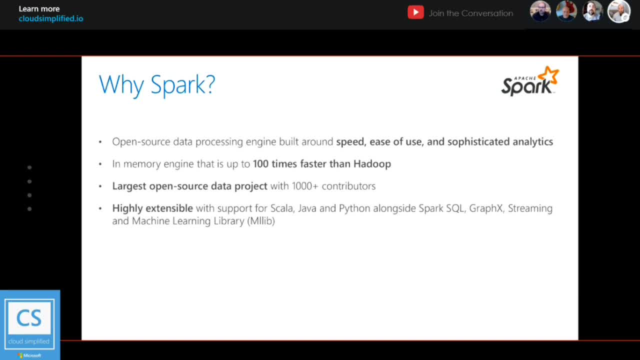 As we were first trying to schedule this use case, it was kind of around the Halloween time and that's a very common analogy that I see for distributed processing engines is, if you think through, Halloween candy like maybe, perhaps bags of M&M's. you know, if you had a bag of M&M's? 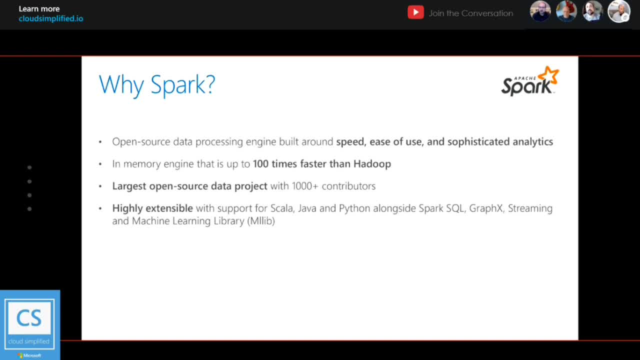 and you wanted to count all the ones in there, you could probably do it pretty quickly. But what if you have tens or dozens or hundreds or thousands? You know, for a single person to do that it's going to take a pretty significant time. 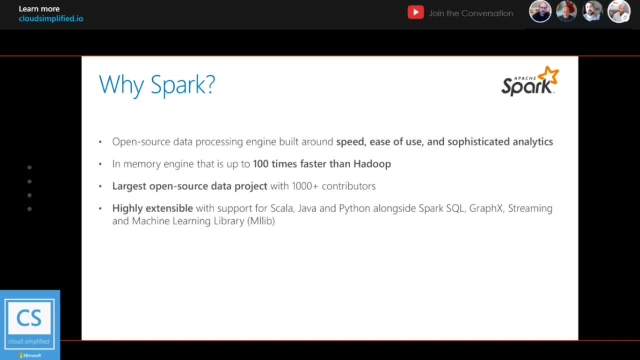 But if you can get some friends, all of us together, we start operating on those individually, we can ultimately perform that job. Yeah, that's a good analogy. So really it's using kind of high-throughput compute behind the scenes. 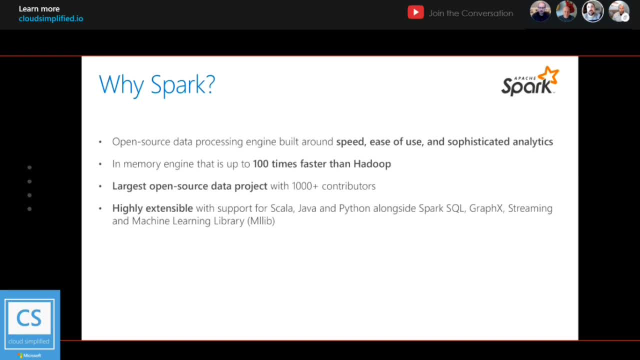 because Azure can facilitate that or surface that very in an expedient, easy manner to customers. because we have, you know, within the realm of physics, virtually unlimited compute capacity that customers can tap into Exactly Okay, And you know the way that it's doing this. 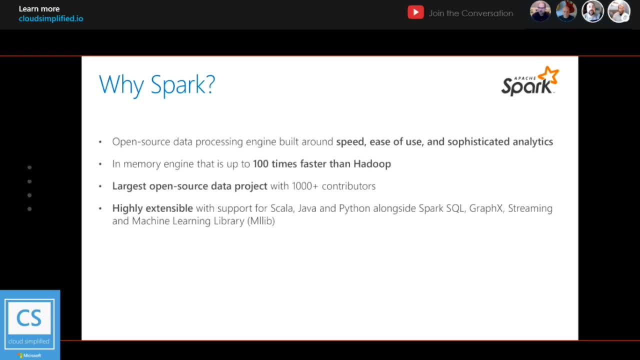 it's passing this work across the different machines in the cluster. it does that through this in-memory engine and that's one of the ways that it achieves a lot of its performance advantages, versus a Hadoop-based technology, where it's very common for the hoop. 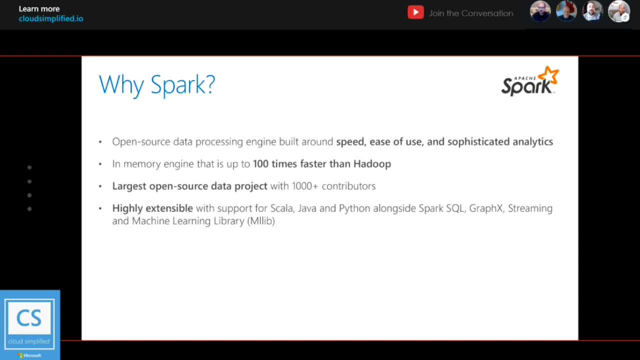 when it needs to move data across individual nodes in the cluster right Or storing intermediate states or steps of the job. it would write those intermediate pieces to disk where the Spark technology tries to operate in-memory as much as possible to get those. 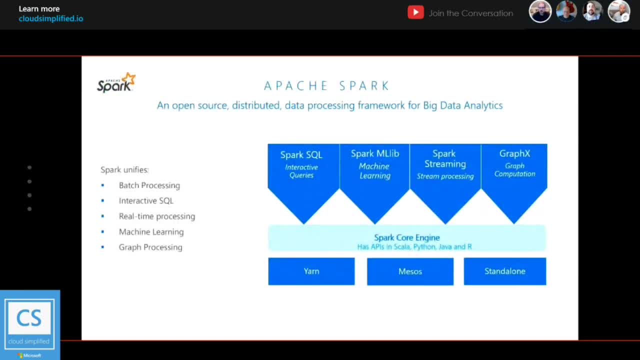 Okay, Okay. So what are some other reasons that Spark has gained this popularity over the couple of years? And that comes to that: it's really unifying a lot of these different data processing capabilities. So not only can I do batch processing, I can also do stream processing or real-time processing. 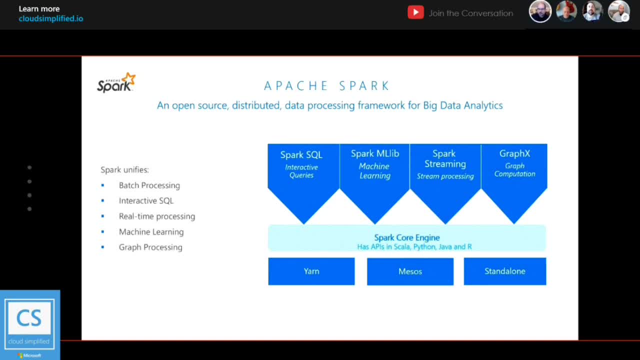 I can do machine learning, I can do graph processing. I can even work to handle interactive SQL and data requirements. all through all of these APIs that are exposed to you, that you get to pick and choose which language that you would like to work with. 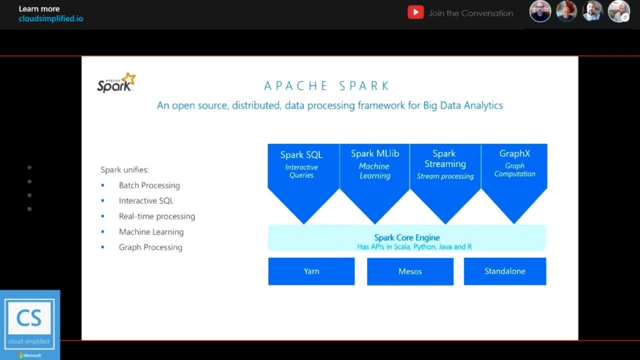 So, in terms of learning curve, you know some of these languages that you can work with in these APIs. someone in your organization likely has one of these skill sets. So the languages that you can work in: Scala, Python, Java, R, SQL. 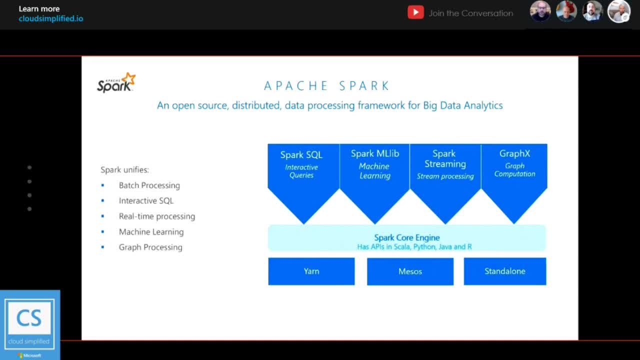 are likely going to have someone in your organization that can work with this to speed up your ease of use. Okay, So me personally. I came from a pretty big SQL background, so being able to work in SQL was a huge benefit, But I was also pretty surprised by how quickly it was. 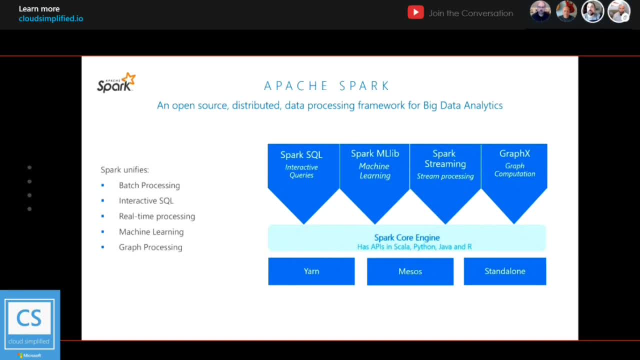 and how easy it was to learn the Python language as well. Yeah, and that's the example I used earlier. The customer that I was working with, their data scientist, had a pretty good background in Python And you know the little bit of instruction on. you know what Databricks can do. 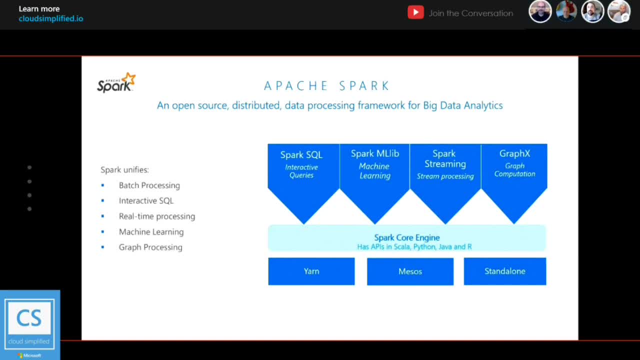 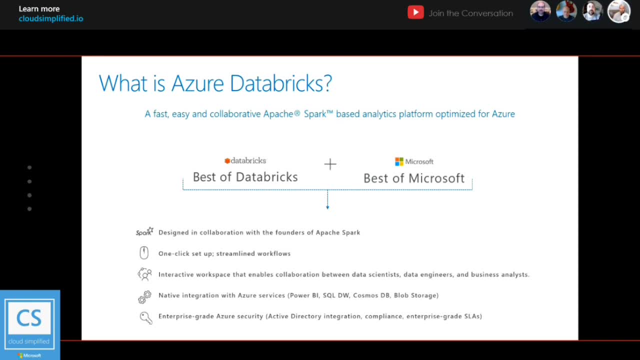 they were off and running Right. So, yeah, Cool, Great. So Azure, Databricks, So kind of. we talked about the different data services, We talked about Spark. now, Well, Databricks. What is Databricks? 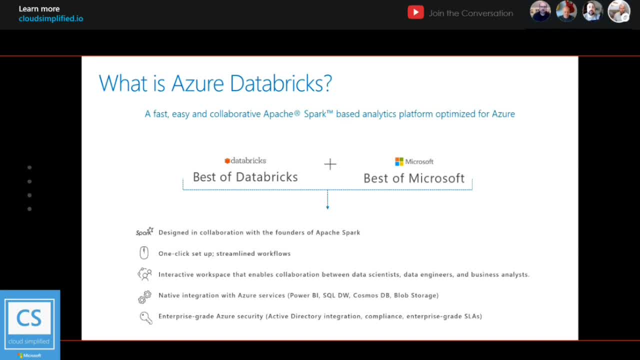 So Databricks is this commercialized product offering that builds on and enhances open source Apache, Spark, But it's also offered in Azure as a first-party service, So that's pretty unique. What that means is: you're not, you don't have your own credentials to access the Databricks environment. 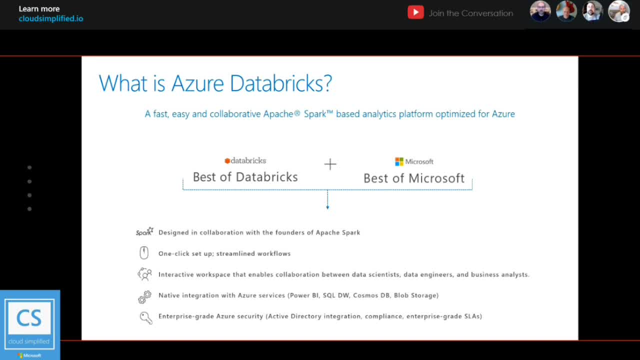 It uses Azure Active Directory. It's a single sign-on environment To get to this collaborative workspace. you're going to the Azure portal. You're opening the workspace. That opens another browser entry. You get that single sign-on pass-through so that you can get started up and running and developing quickly. 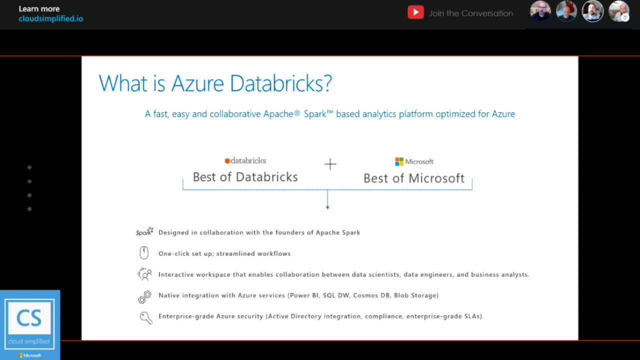 So customers could deploy this in their own environment, right? So it would be in their own environment inside of the Azure platform, or I just mean, like you know, it's a commercialized product. I was just curious. No, it does not work on premises. no, 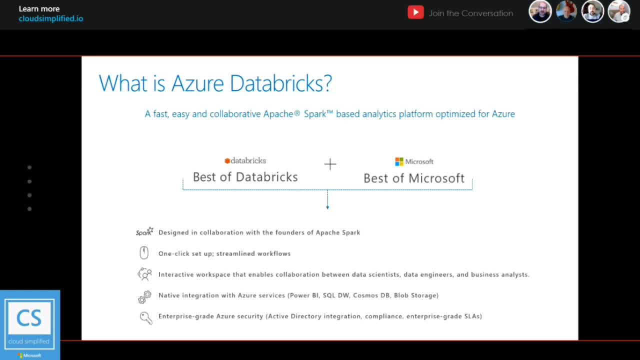 Okay, Okay, Sorry, Ryan, You can't steal this. No, no, I just wanted to air that out. That's sometimes a question, You know what? Yeah, Yeah, No, Okay, Yeah, You could potentially set up your own Apache Spark clusters on premises. 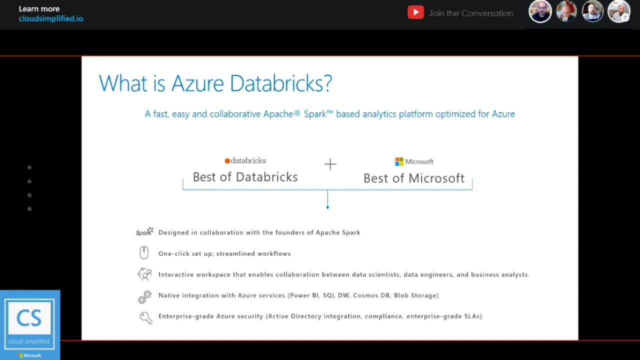 That can be done, Okay, But you wouldn't be running Databricks on premises, Yeah, Okay, Yeah, You know the. I guess the next train of thought here was, you know, being that first-party services. it has a lot of this native integration with a lot of the other Azure services that we talked about previously. 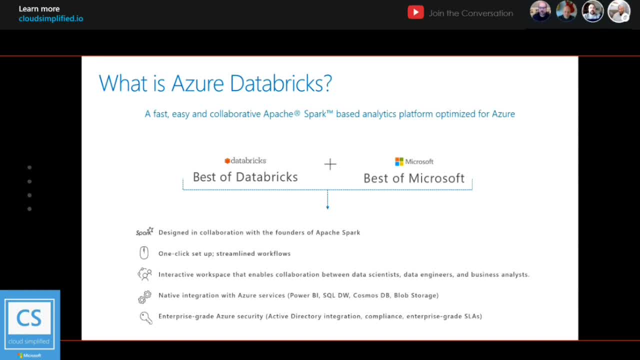 So Yeah, Being able to, once you process that data, land it to some other services, whether that's just pure storage, whether that's SQL Data Warehouse Cosmos- if you want to visualize that data with Power BI- that integration with these other Azure services really works. 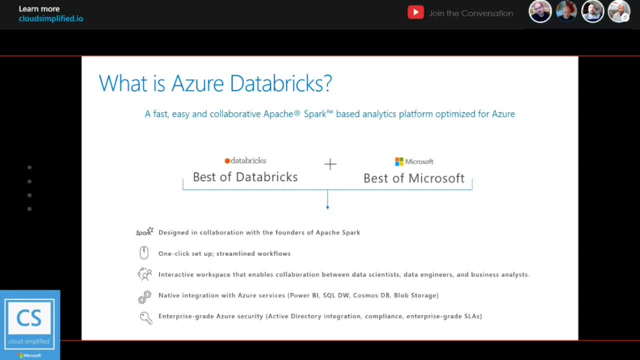 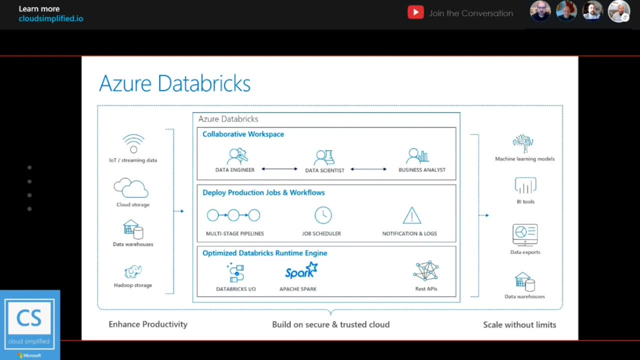 pretty nicely as well. Okay, Cool, All right, The last slide on Azure Databricks here. So what are some of the features? functionality it offers: It offers this collaborative workspace- think Jupyter Notebooks- but it has Databricks'. 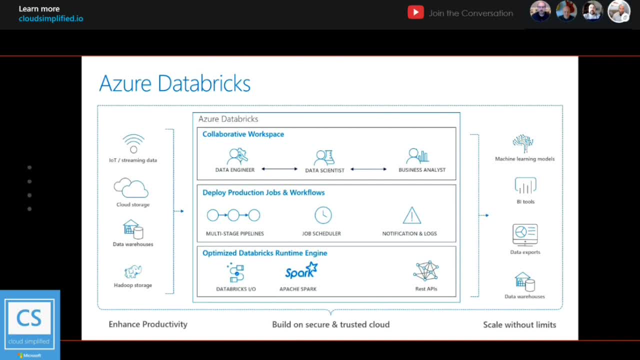 own kind of spin twist on it, And this really provides a lot of different end user types to collaborate in a single location, So you can work from a single notebook. you can add comments. It provides the ability to, once you've actually finished your notebooks and you feel like. 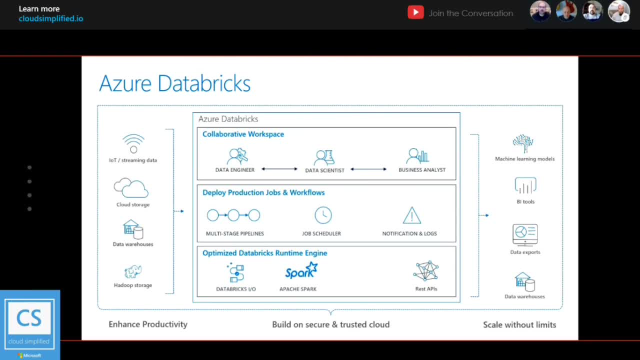 it's ready to go. you can productionize those jobs and workflows through some schedulers. You can also set up things like alerts and notifications when things may be failing, And that's all going to run on the optimized Databricks runtime engine. 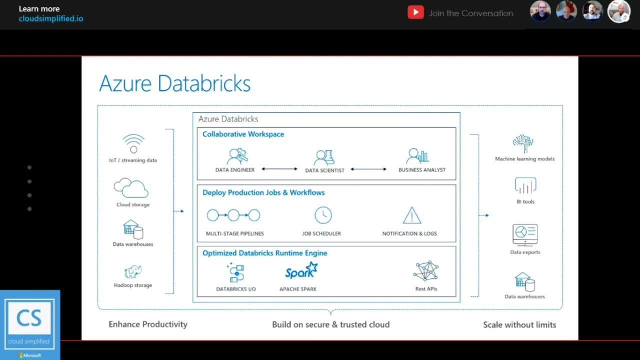 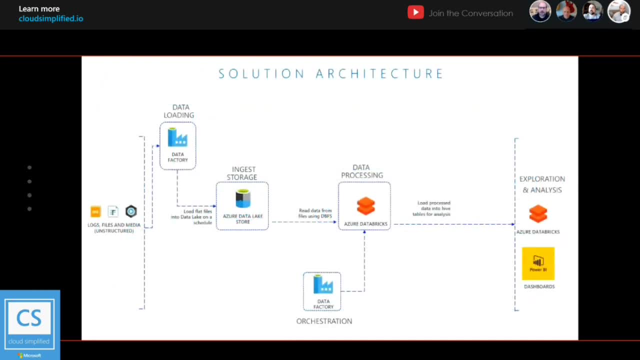 And a lot of those. the features and functionality for the API APIs are exposed through various REST APIs that help you get up and running pretty quickly. Do we have tutorials? Do we have like a place to go where a customer can start working with? maybe some examples? 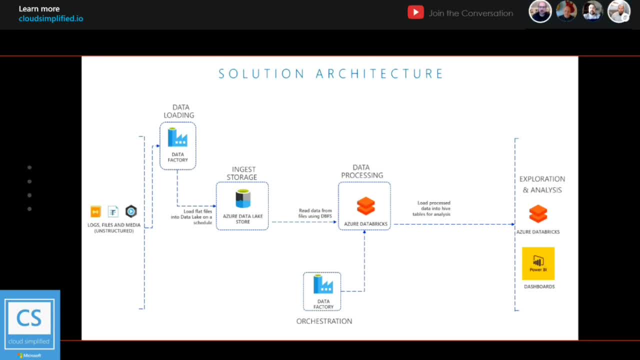 Probably out of GitHub. There's plenty of examples out there, So probably docsmicrosoftcom, forward slash, Azure, Okay, Kind of walk through getting started documentation there, And I'd be shocked if there weren't links. There are links in there to various GitHub repositories as well. 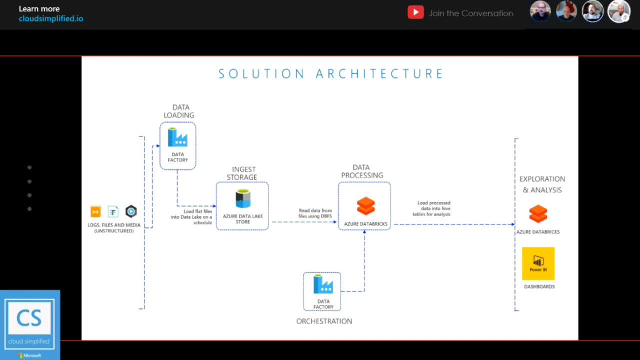 Okay, Okay, Yeah, If you have any to share for the audience, you can definitely pass those along. We'll get those in the show notes. Yeah, Yeah, Actually, subscribers want to know What did the solution architecture kind of look like for this given customer challenge. 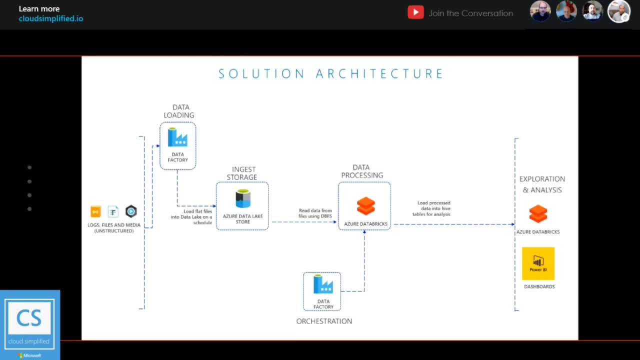 So we talked about this a little bit, but this hopefully puts it into pictures for you to more easily comprehend. So really, that data loading piece, How do we get those FTP files? How do we get those files into Azure? So that's, you know that data factory slash Python scripts that we're running and it's. 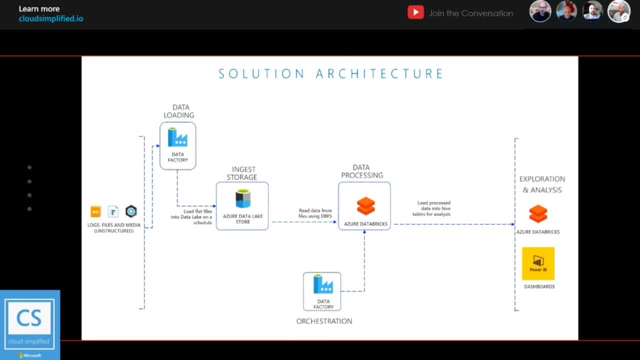 also going to land that to Azure data like store, So that's where we ingest everything. We then use Azure data factory to kick off a Databricks notebook That's going to process those files And it's also then going to create some hive tables so that we can start to visualize that. 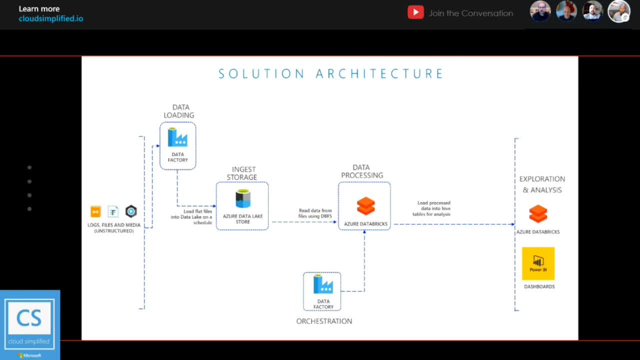 both interactively through different notebooks. Okay, So at this point there's been no human interaction, from data load to table creation to prep for visualization. right, Because when you said it kicks off a Databricks workspace, that kind of flipped the flag on. 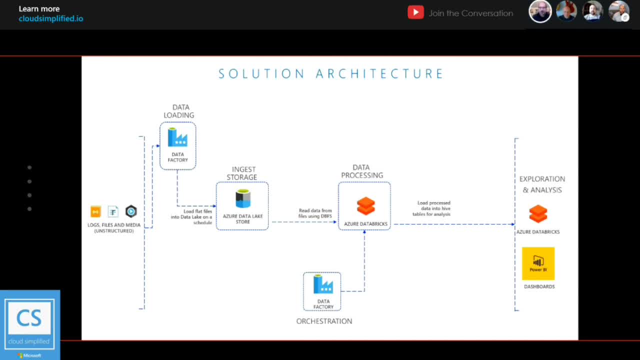 for me It was like: oh wow, we really can create data in an automated way and save ourselves a lot of cycles. right, Yeah, Yeah, Yeah, no right, Yeah, Exactly Yeah. There's no human interaction other than the analysis that's happening at the far right. 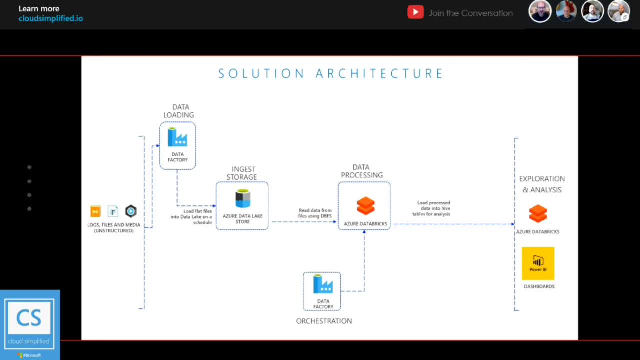 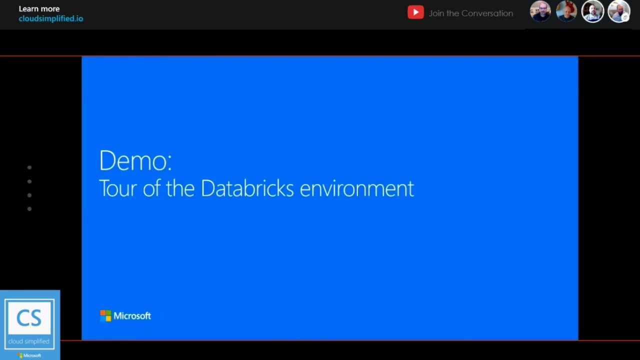 of the screen. I'm out of a job, All right. So you said you had on that note. so you said you had some demos to kind of walk through a little bit about how this works. Yeah Cool, I'm really curious to kind of see how it's all assembled there. 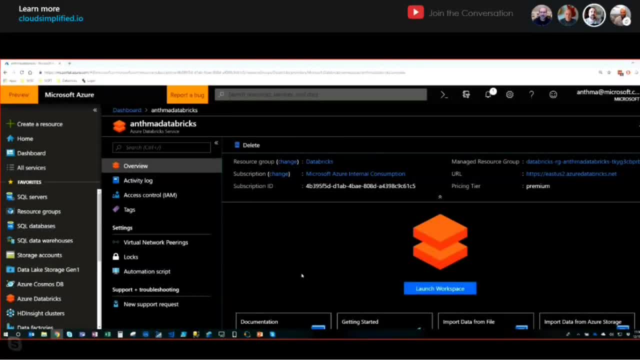 So now we're going to click into the brick right. You know I was holding it up earlier, but Click on that. I want to see this. Hey, you'll be on YouTube forever and ever and ever. It'll go viral today. 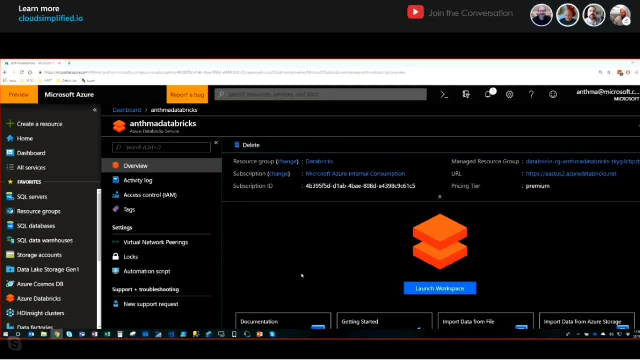 All right. So let's get started and show you what kind of what this Databricks environment looks like. What's it all about? So here I am in my Azure portal. I have an Azure Databricks service spun off, And this is where you can start to see what that integrated AAD authentication looks like. 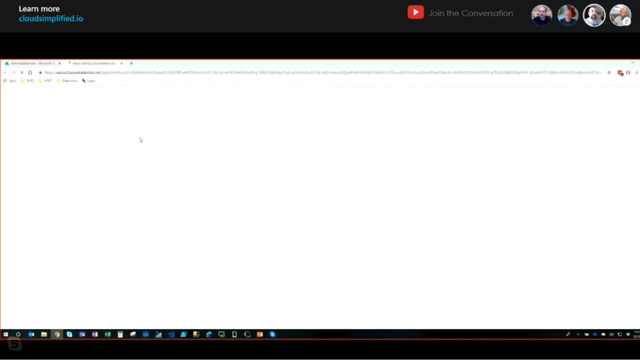 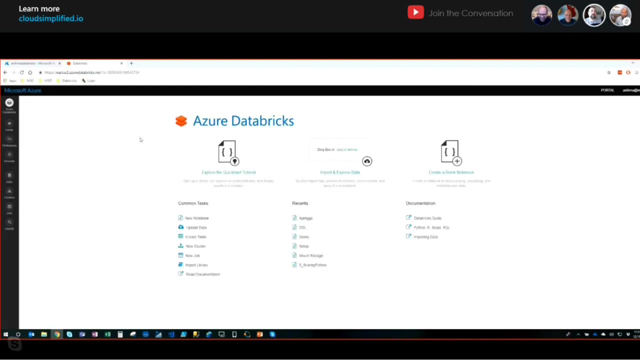 So I can just click Launch Workspace. It's going to pop up a new tab in my browser. It's going to go through the AAD sign-on And in a second or so we should see what this Databricks environment looks like. 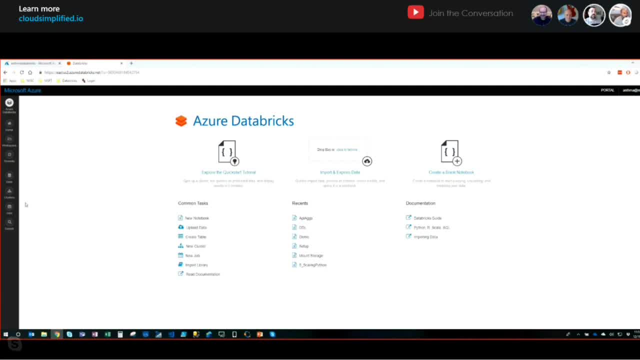 Great. So here we are. This is going to be your main landing page. Some things to pay attention to? Probably the clusters. So everything's going to operate on a cluster. Here I have my interactive cluster set up called Sparky. Here you can. 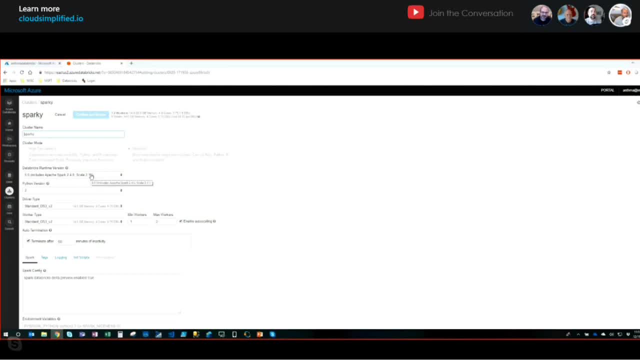 This is where you can kind of edit the configuration. So there's different runtime versions. I can run different versions of Python. There are virtual machines under the cover, although we don't- We're not responsible for kind of maintenance, patching any of that. 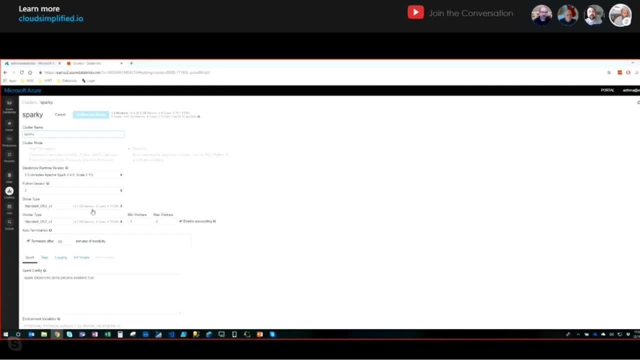 We're just picking a size that's going to have an associated memory and cores with it. And this is one of my favorite pieces to Databricks Is the automated scaling that's built into it. So I can say: hey, you know, I want my minimum number of worker nodes to be X. 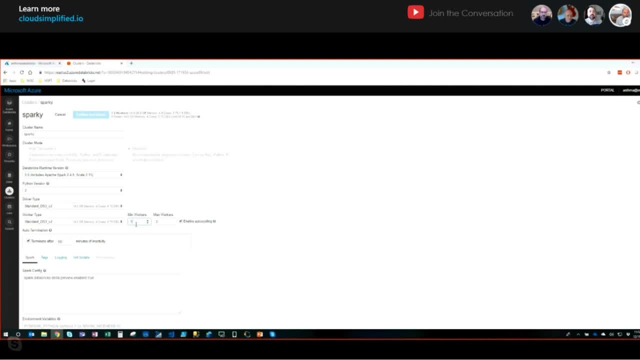 And I want my max number of worker nodes to be N, And this little checkbox will enable auto-scaling, So it'll look at the amount of work to be done in the cluster And if there's jobs that are in a kind of a waiting or a queued state. 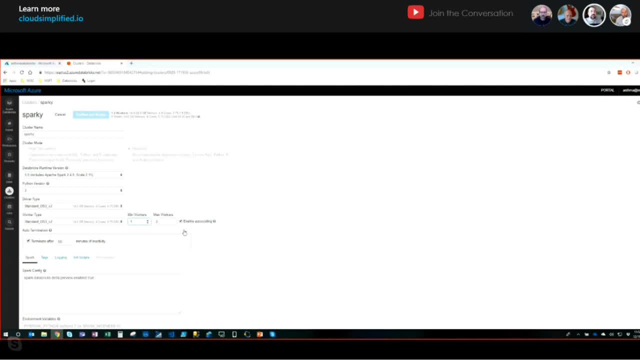 it'll automatically scale up, slowly and slowly until it hits that max workers for me, So it allows you to contain the cost then at that point, So you can. Yeah, exactly, I don't notice here, too, is that I don't see where, like in our VMSS services. 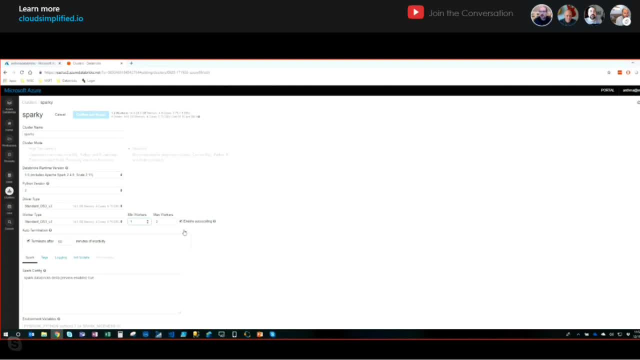 you set the thresholds for the scaling event. This looks like it's all again abstract away from customer, But our best practices are our choices of when we scale up those nodes. You know along those lines of containing cost, one of the big things you know. sometimes you'll wake up in a panic with 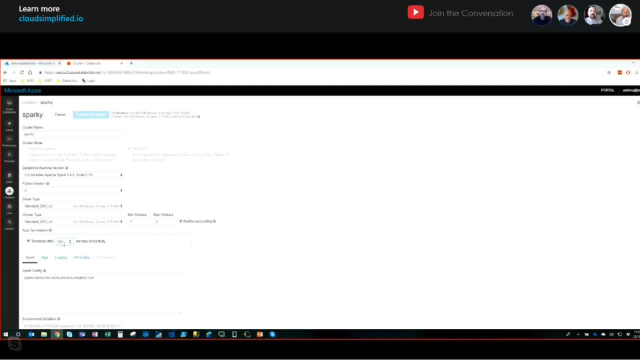 you know, particularly HDInsight clusters. Hey, did I leave my cluster up and running? That's going to consume significant consumption. Never To auto-terminate is really handy. So hey, if I forget to turn this thing off or no, work's being done. 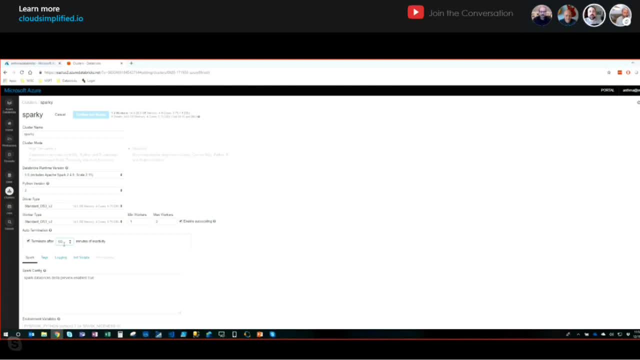 just go ahead and kill that in the background. for me It's kind of like the shutdown rules on a VM, So it's a good way to again help control. Okay, So with that defined, you know, just being a development environment. 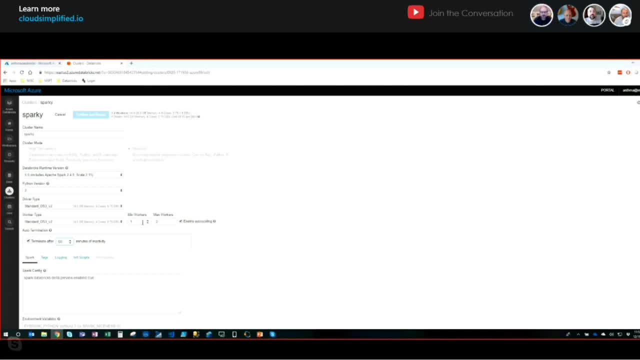 I got it set up pretty simply here. So just you know between one and two worker nodes, But from there we can get to the workspace, And the workspace is kind of this notebook-based environment where we can collaborate on different projects. 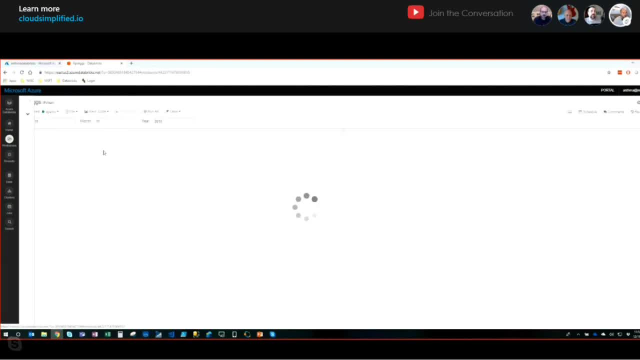 So inside my demo, I'm going to head over to this specific notebook called API, Ags or Aggregations for short, And I'll kind of just kind of walk you through what this looks like Really within this notebook. you'll notice that we have some different parameters. 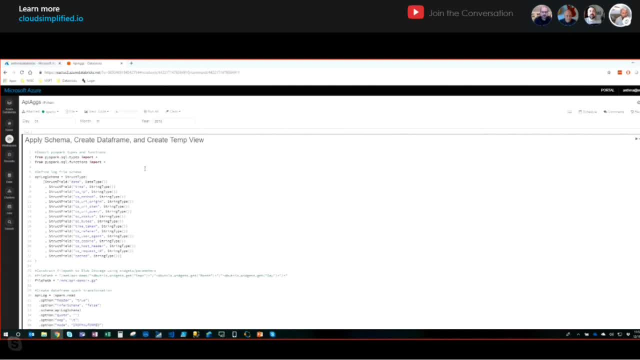 or widgets defined at the top, And that gets to that kind of batch processing nature of this. So what we want to do is data is going to be stored Inside of our data lake And it's going to be partitioned into different directory structures. 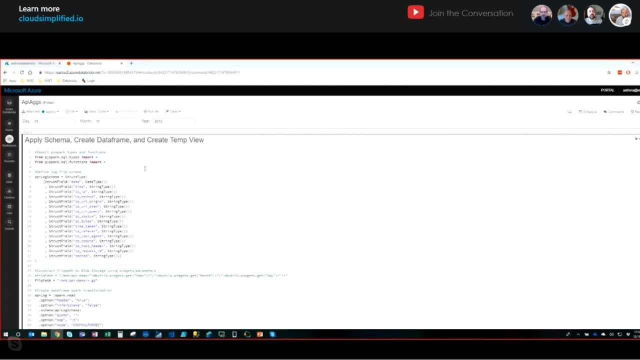 based on the year, month and day So that we can operate only on the specific files that we're interested in. So that will be utilized inside of the script here, So we kind of glossed over that. just to quickly highlight, We use the word data lake often. 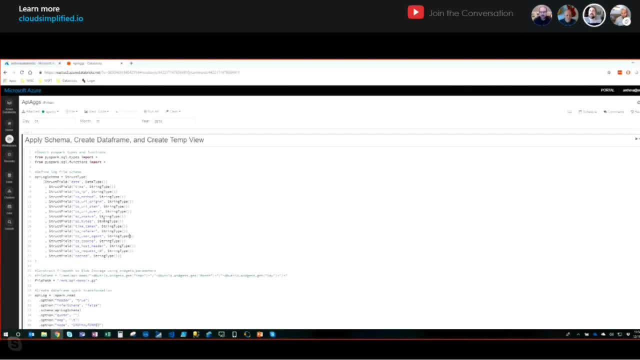 But it's really. it's just a repository that you can dump data into, with some rules to kind of define how it's- using your word- partitioned or physically stored to be able to access and retrieve it, And it's accessible by services such as Databricks. 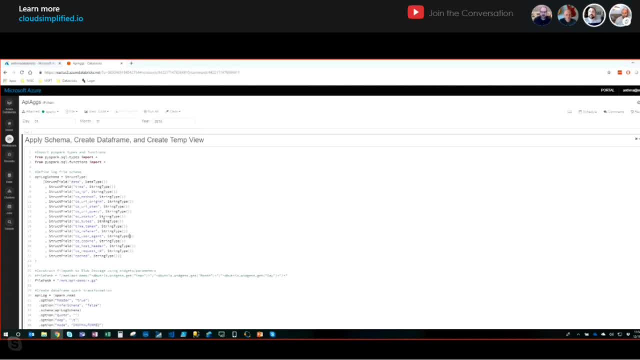 Right, Exactly And in simplest nature, a data lake is a distributed file system that doesn't have any sort of limitations on file size. Yep, Okay, Unbounded. There you go. That's a good way to Okay, Gotcha. 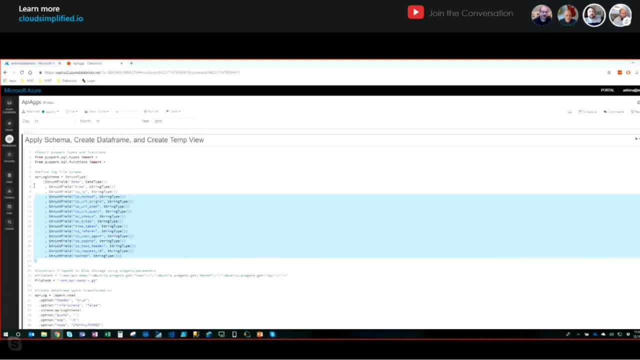 Yep. So if we take a look at the script, the first thing that we're doing here is this is some Python And really it's just defining structure. So we're defining structure to those underlying files. So it's a comma separated file. 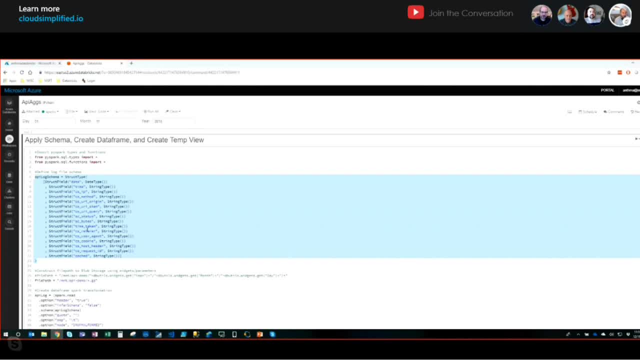 These GZIP files that are coming across, And they do have structure to them. So all I'm doing here is I'm going to define my schema that we're going to utilize. So, hey, it's got dates, It's got times. 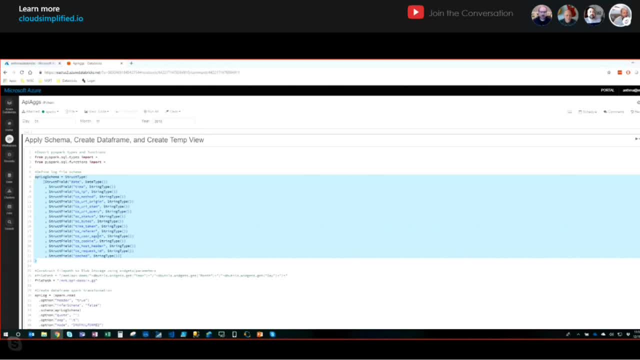 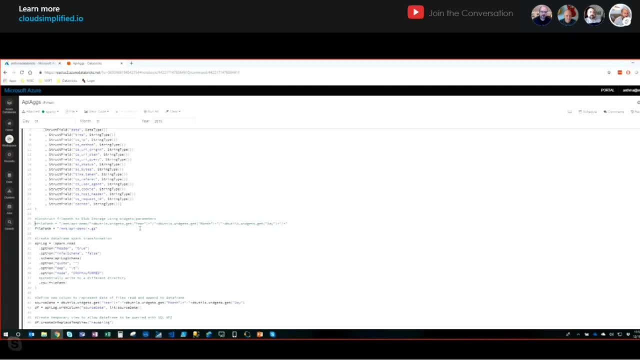 It's got IP addresses, It's got tokens and different things. We're really just defining the structure. We define the file path that we want to read from. You notice that I kind of got this commented out. This was kind of more production worthy. 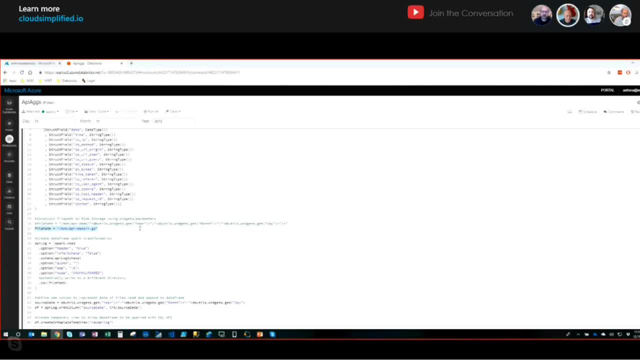 This is definitely a simplified version. So, hey, if I just got a single file for in terms of demo purposes, I'm just reading from this mount point, And that mount point is pointing to blob storage, And I have a container and a directory. 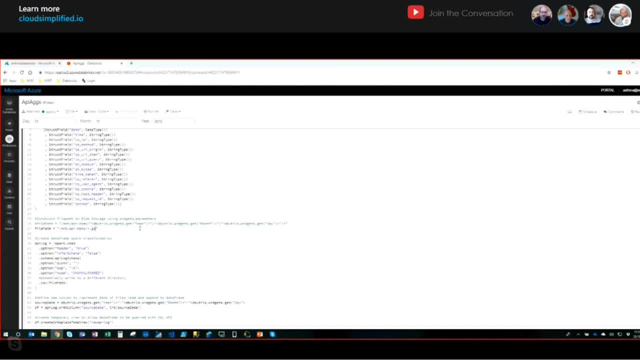 And I'm going to read all the given files with a gzip extension, Okay, Of that container. The next piece is to call a sparkread, And you can. everything is kind of self-explanatory in terms of the options here. 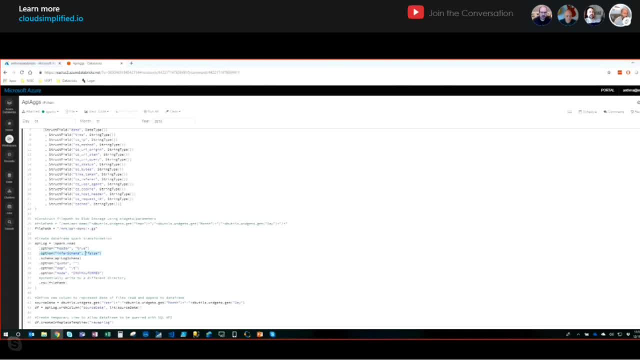 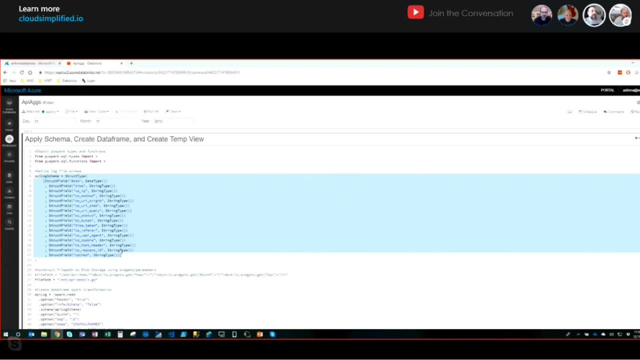 So, hey, my file does have a header. I'm not going to infer the schema, I'm going to use the schema that I defined just above. The API log schema is exactly this thing here. What's the schema or format of our data? 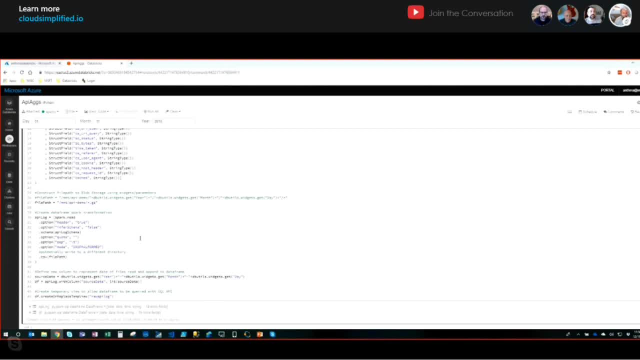 It's going to be tab separated. If we have any sort of issues with bad data, to your point, we can drop those malformed rows, Okay, And we're going to read it in as the CSV file. So it'll drop just the malformed rows, not the entire file. 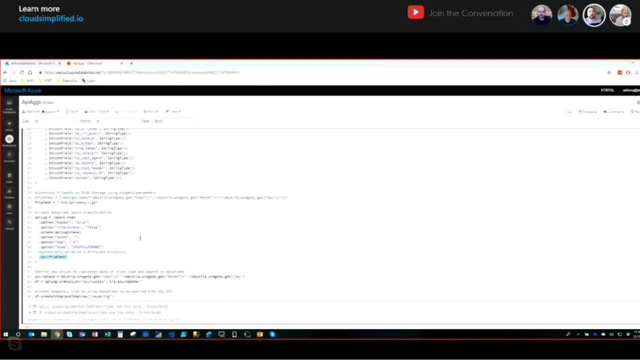 Okay, Okay, And there's some different options that you can have there, But this, any sort of bad rows- we're just dropping them, Okay. So this all goes to a thing called a data frame, So we can then work with this API log. 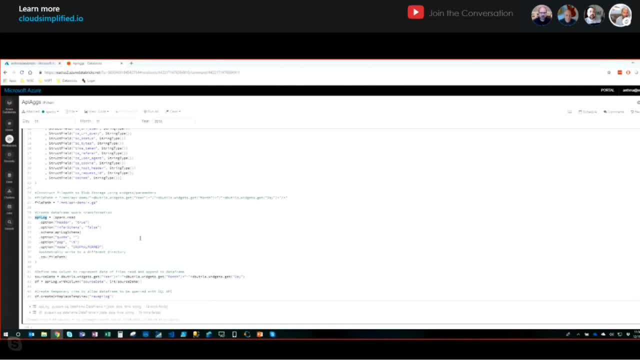 This is going to be this data frame. Think of it as really kind of a table. It's got rows and columns. once we've read in all those files from the file system And we can do different things with it. So we did some other advanced things here, like: hey, it would be really nice if we load all this data. 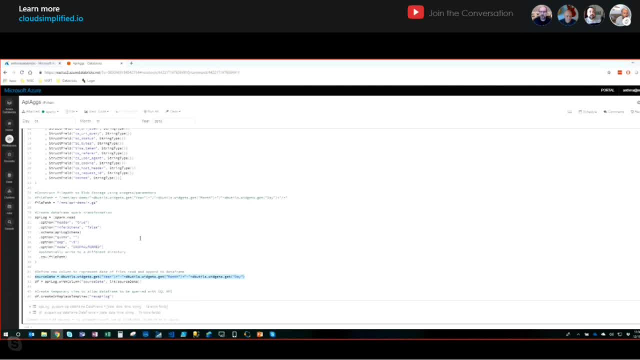 It would be cool to understand which rows within the files we're able to understand that. So, hey, which rows of data came from this file versus? here's just all the data, rows and columns That came from hundreds of files or thousands of files. 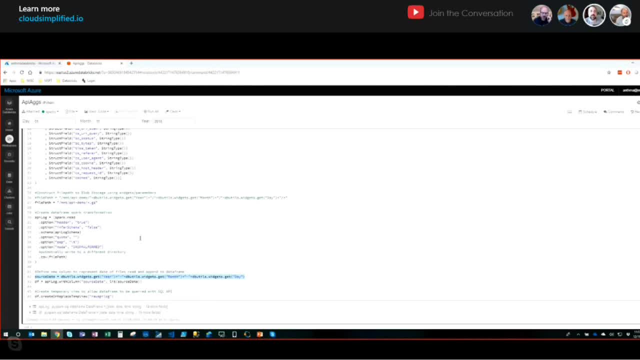 Let's just append, Let's get the file name and the specific source date And let's append that to the data frame, And then, finally, we create a thing called a view on top of that data frame so that we can start to work with it in the SQL API. 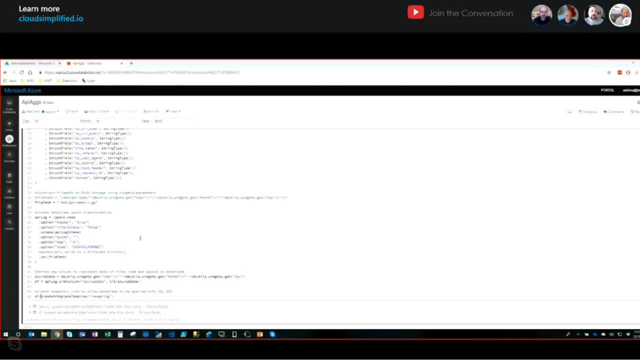 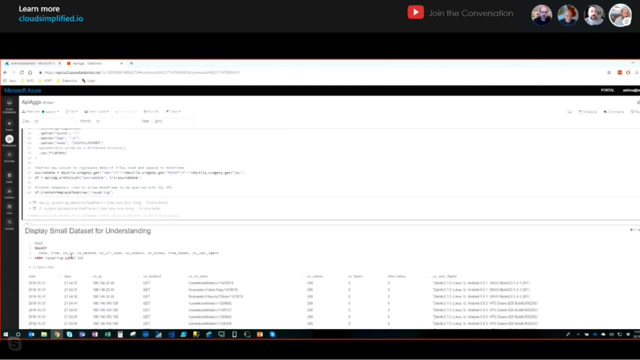 So I just run like a control execute that's going to send this cell to the cluster And it's going to execute fairly quickly, So you know a third of a second And then, because it's in that view, I can run it. 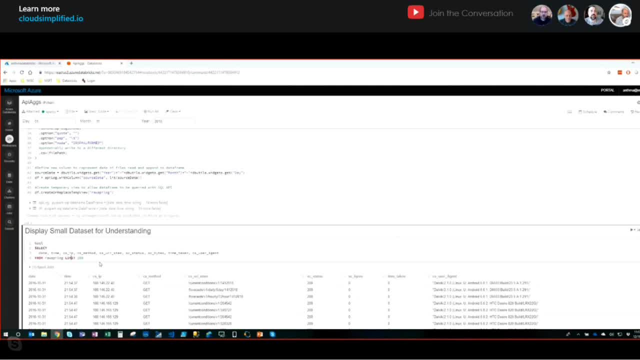 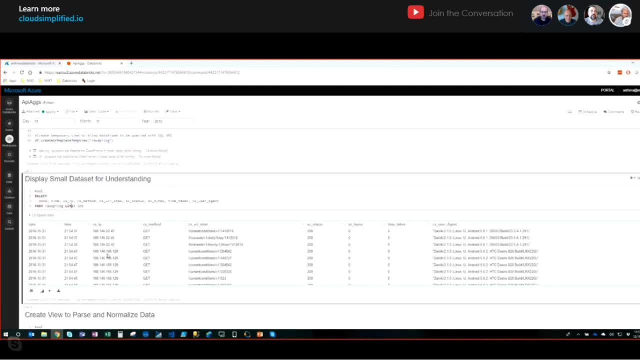 I can then just use my own skill set that I'm very comfortable with in SQL, And I can just query this in SQL. So now I have a data frame, I can run it, It will execute it against the cluster And I get to start to see the results. 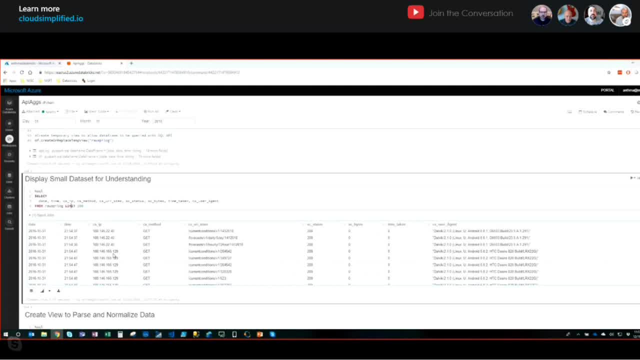 So we can- this is the first piece- Apply the structure, Then take a look at what the data looks like So you can see. I have dates, I got times, I got IPs. I can see the different APIs, that they're hidden from that URI stack. 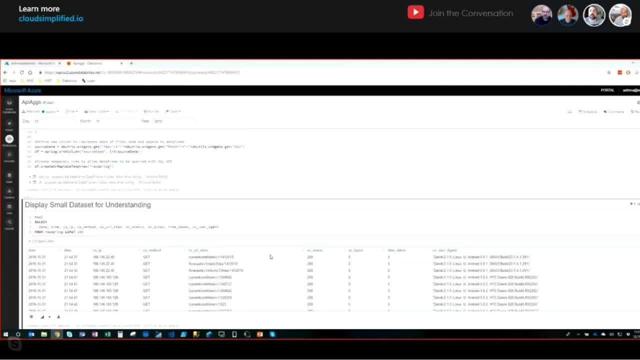 Oh man, that's cool, Yeah. So this is a good way to do some exploratory work, to see you know what does your data set look like, That you're actually going to work with, to kind of pass on to subsequent phases. 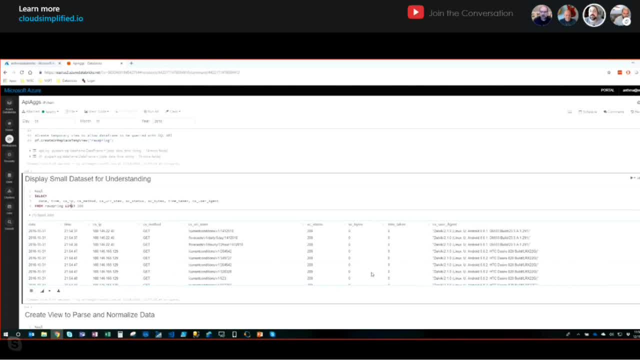 So this is kind of the iterative approach you take as a Databricks developer really, Exactly. Yeah, Yeah, Okay, That's cool, One of the cool things: you can see what kind of devices are our end users using. 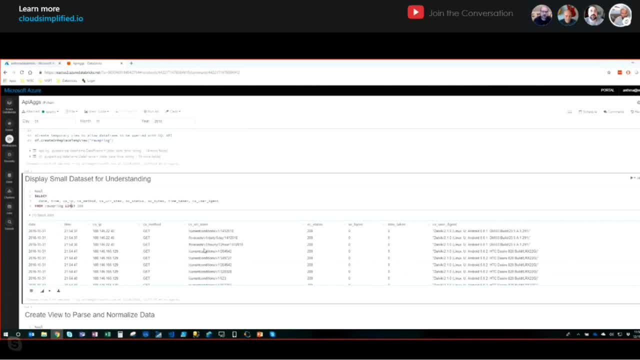 You know, are they using iOS, What versions of all these things? But if you'll notice, like I talked about before, we need to kind of break this apart so it can be analyzed Like this isn't all that helpful when it's in this long query string. 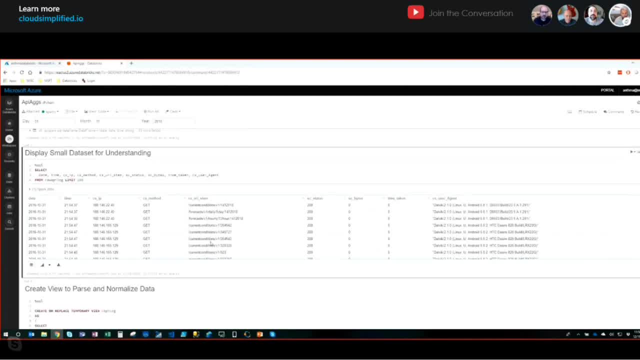 So what we'll do in this next step is let's start to break this apart and define. you know, define specific columns or fields for these different pieces of these stems or different pieces of you know the user agent thing here. So this is a. I'm not going to go into too much depth here, but this is what that looks like in SQL. 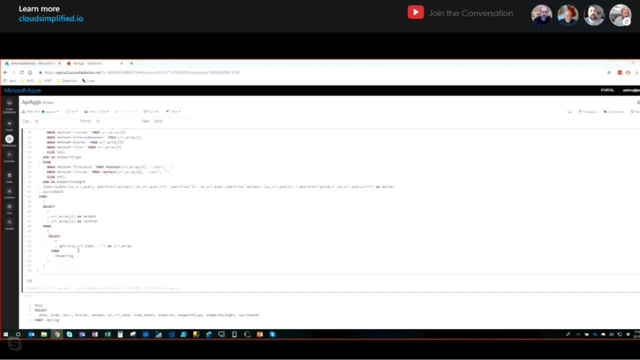 So we've got some case statements and more splitting based off of the URI stem here. So this is kind of the data transformation. How can we get break apart these different data elements that were previously stored in one column and get them into their own separate data columns for analysis? 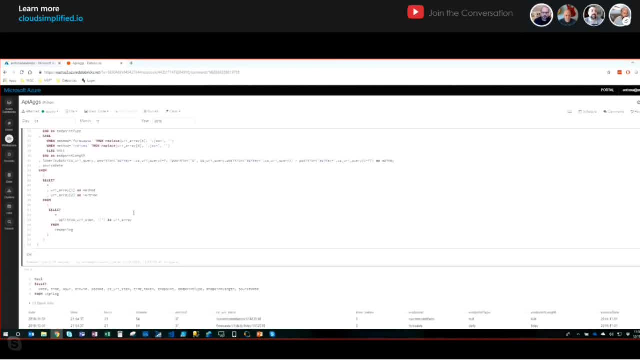 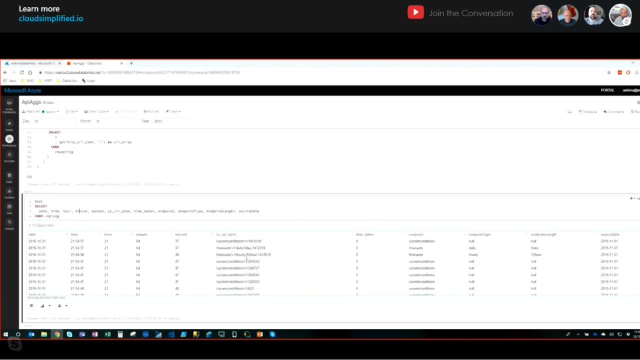 Okay. So if we run that little guy there, it'll run, And then what we can then do is run against that new view and we'll start to see what things look like. So if we take this, for instance, we can see- okay, here's my endpoint- current conditions and the type of endpoint. 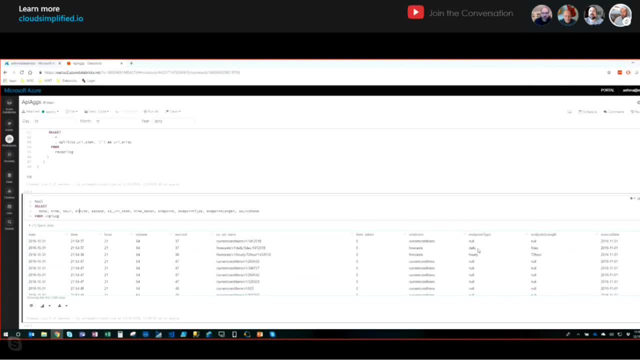 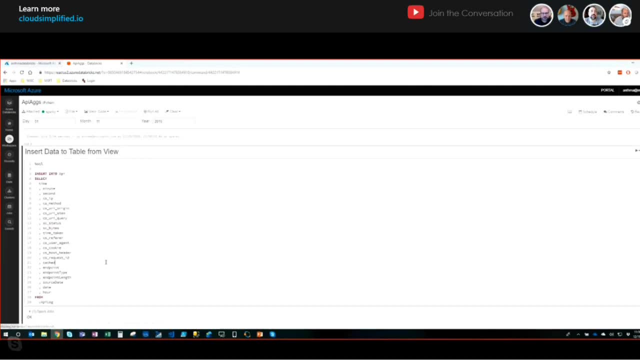 Is it daily versus hourly, And are they looking for the five-day forecast or 72 hours? So we can start to break that apart and ultimately we can then start to analyze it a bit easier. Okay, Yeah, The next piece. let's, what we would do is then log that into a table. 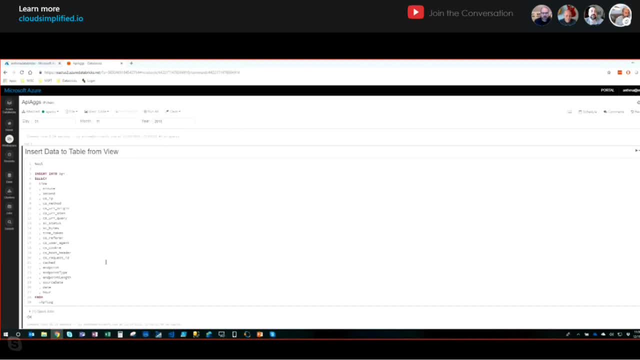 So, as the batch processing runs, let's get this into a single entity and we create hive tables for this. So this goes to: we're inserting the data into this API. I'm not going to run that. How would you, for those familiar with, like the relational database world, how would you compare a hive table to you know a table in SQL? 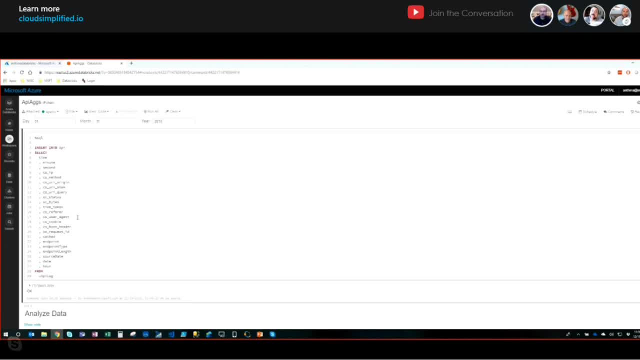 Very, very similar. Okay, Yeah, I mean, obviously you're querying it similarly. Yeah, I just didn't know if you had a. okay, So that. so that's, that's so, yeah, Okay. 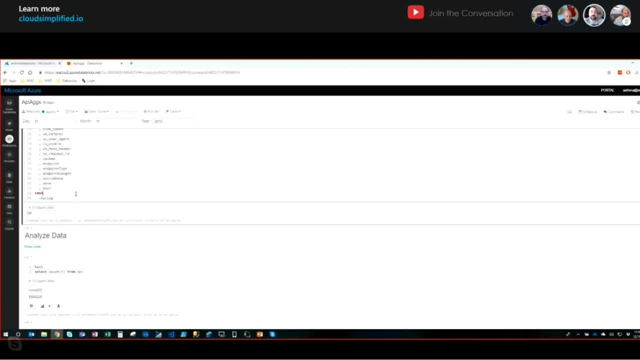 That's Spark's way of being able to, to make it easier to be able to, to do things like this in a structured manner and be able to get data back out Exactly Okay, Okay, And then we can do our traditional analysis. 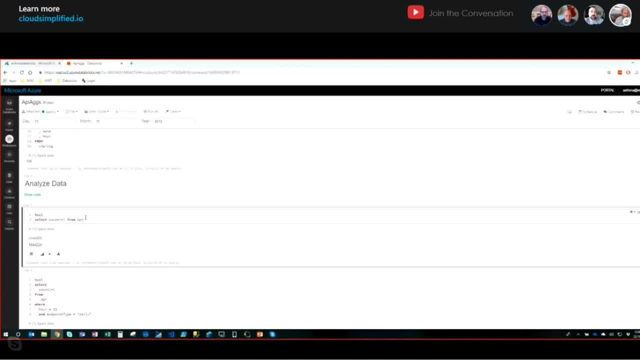 Hey, how many rows of data came in for today. So things like simple count star, So you can see. you know what do? we got 1.8 million rows. This was just a single file, but when there's thousands, obviously we talked about the data volume that grows pretty rapidly. 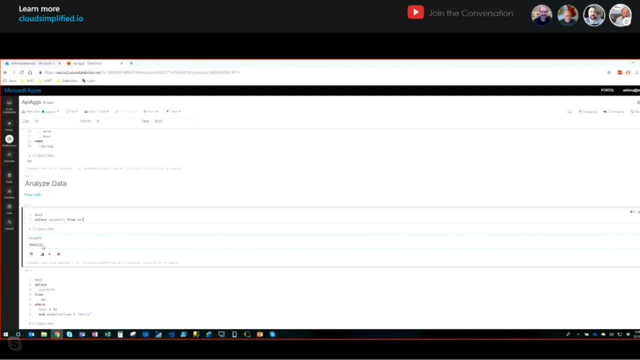 Yeah, And you'd be shocked really by how fast it, when you scale it, Yeah, When you scale it up to the number of cluster nodes that is appropriate, it returns very, very quickly. Okay, It's just a million rows, Ryan. 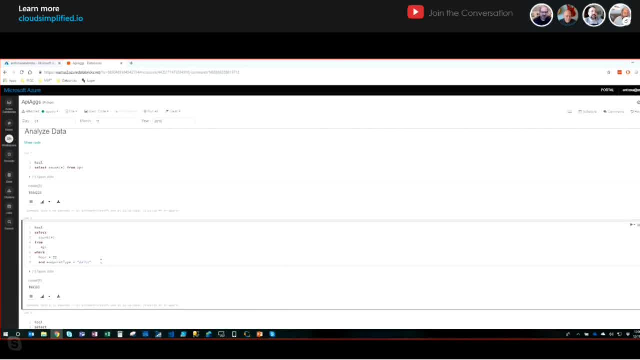 Yeah, Just a million. Yeah, Yeah. So then you can see you can do different things. Hey, I'm interested in you know a specific hour and I want this specific endpoint type. You can then run those queries, get results very interactively and you're not. 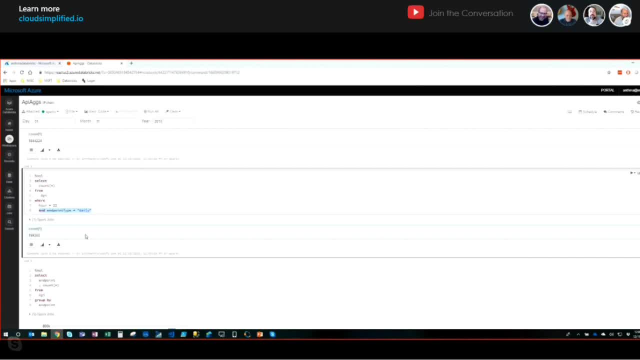 That's actually. that's actually crazy fast when you think about I was going to say: you see how quick it's coming back. Yeah, That's insane. And when there's more data, it also. This is: you were accessing it in a kind of a, you know, relational way, but it doesn't have indices and all of the other things that kind of go along with a relational data store. 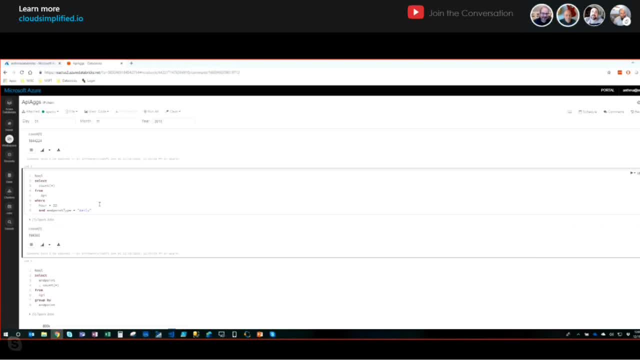 So when you think about Nothing to make it fast, Yeah, When you think about that and you have a where clause in there and your, you know some criteria, that's pretty, that's pretty cool. It's not to say that there isn't other optimizations that you could do under the covers, but 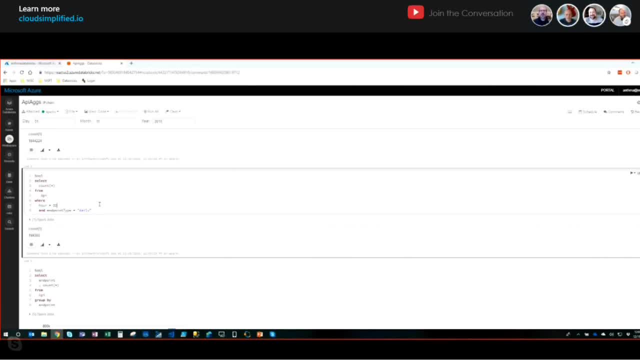 Oh look, he wants to make it go faster. I love that. Oh there's, We can, we can. It's not that slow, Yeah. Another cool thing in the notebook is: you can also. you're not just restricted to rows and columns or single results. 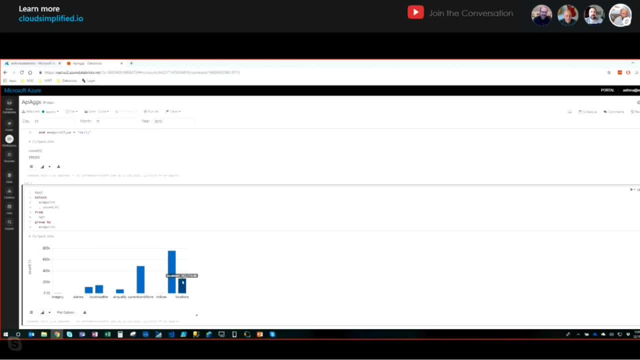 You can also get graphs and start to change the data type. So here we're just plotting a simple column chart and we can see you know what are the endpoint types that are. You had me at graph. Okay, I'm good. 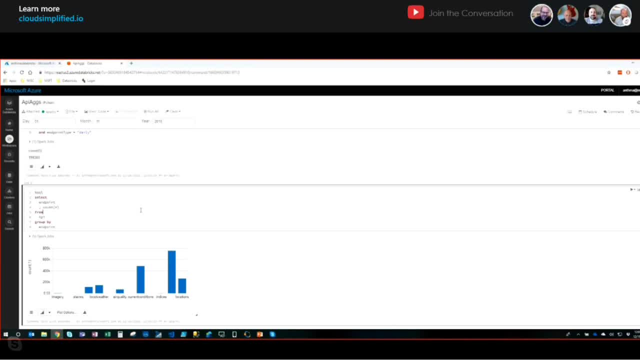 So that's really what I wanted to show you, Kind of just a brief introduction to what the Databricks environment looks like. See how you set up the cluster, see how you can read it in the data set, apply some structure to it and then start to query it in a language that perhaps you know, many of you are familiar with, in the SQL language. 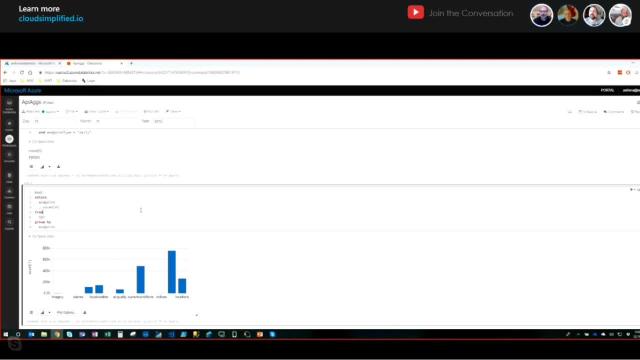 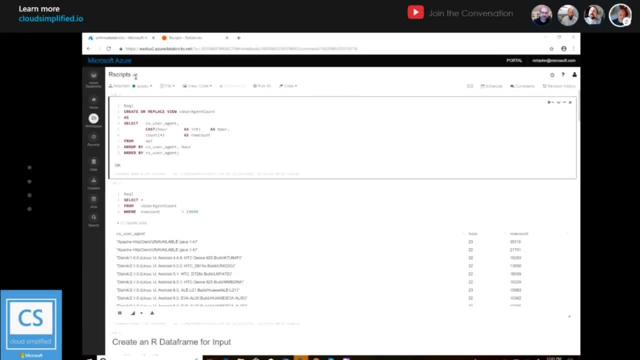 Yeah, not to put you on the spot, Rich, but you got some big shoes to fill here, bud, All right, Okay, Yeah, So this last notebook. if you look up at the top, I just call it R scripts and you can see right next to it: R. 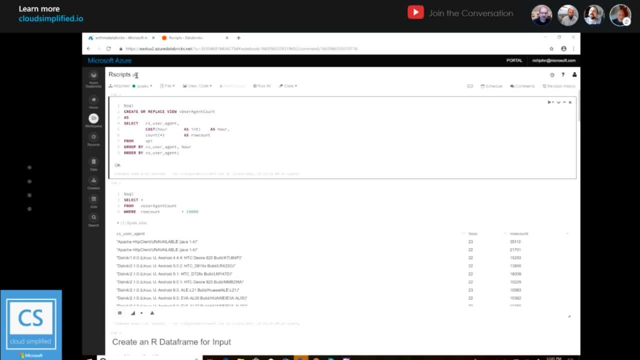 So you know, I have to kind of explain. There's different notebooks. You can create it with the default interpreter for Python or Scala, R in this case, and even SQL, And so I created this notebook just really as kind of a learning experience for myself and then show it to some of the people at this customer so that it would more be along the lines of data scientists or statisticians. 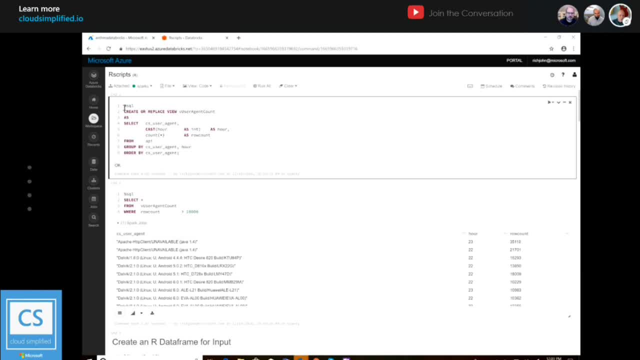 So if you notice, here there's this little percent SQL command in this first step, in these next couple steps, And that says, hey, I know this is an R notebook, but treat this next command for this cell as a SQL script. 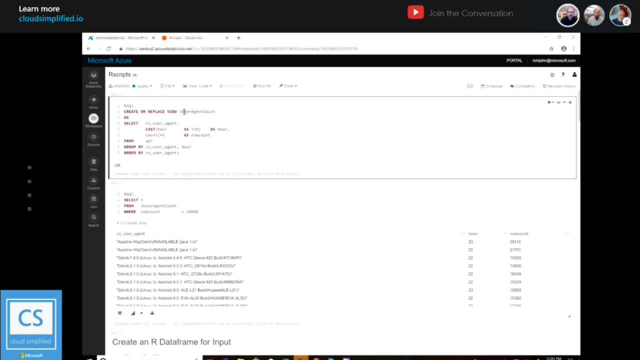 So, as we showed you, As we showed before, simple things like creating or replacing a view is just a select against a data table you may have out here, And so typical things we would do is just select on some data, maybe a group by, in this case, agent an hour and order it and then return that count. 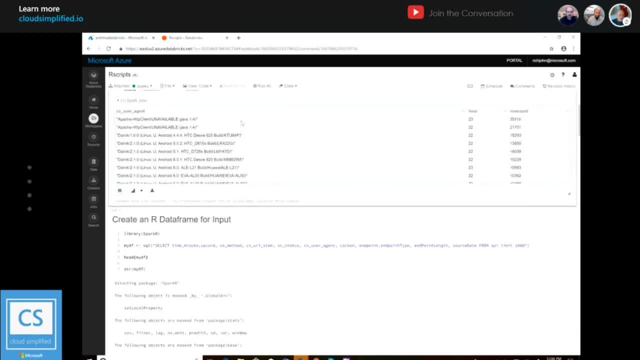 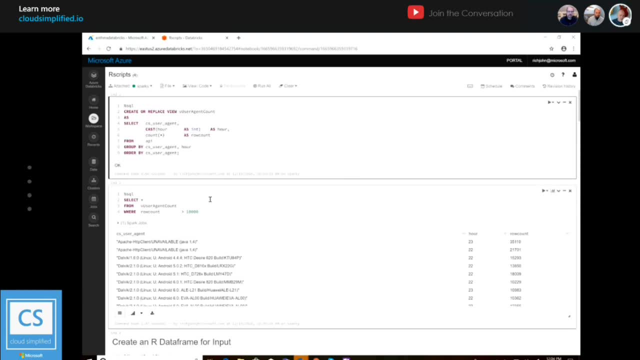 And then in this next one as well. So here's a similar query to what Anthony was showing. I just want to show now that I created this view up in the first cell, this V user agent. I want to select star from that. 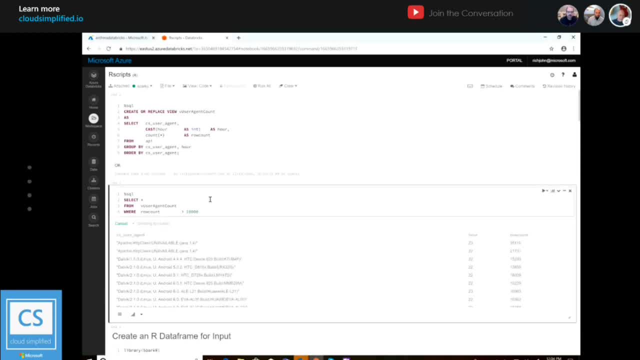 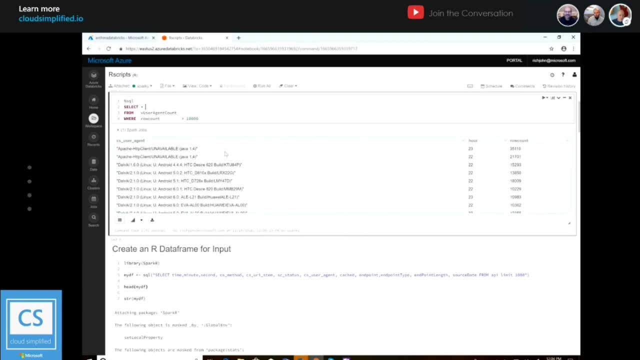 We're row count. It's greater than 10,000.. So I can go ahead and control, enter, execute that And you see it comes back Again pretty quick. It's the same data that we were looking at before. 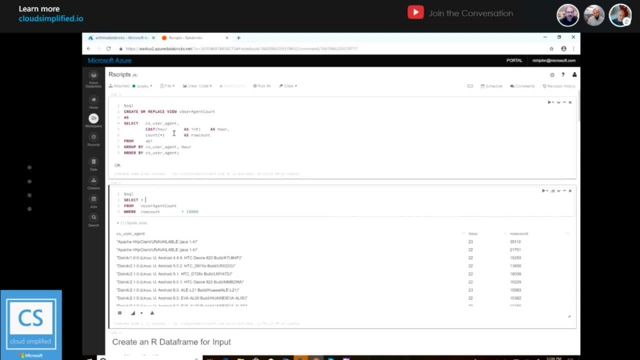 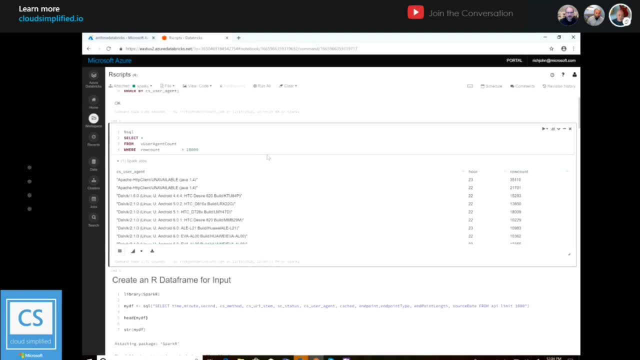 But now that I've got this view, it's aggregated up at the agent and hour level. So this is when we talked earlier that maybe you want to aggregate data for certain personas or user, business groups, business segments in your organization. They may want just this optimized data every hour or every day. 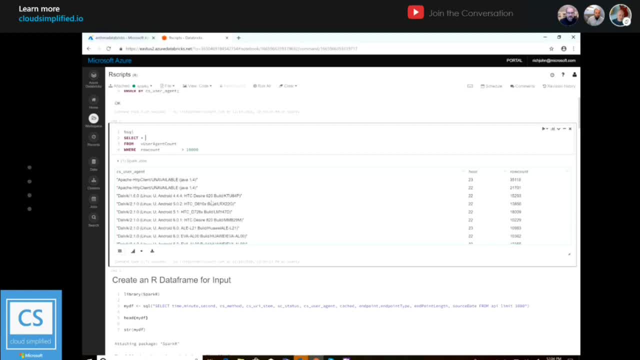 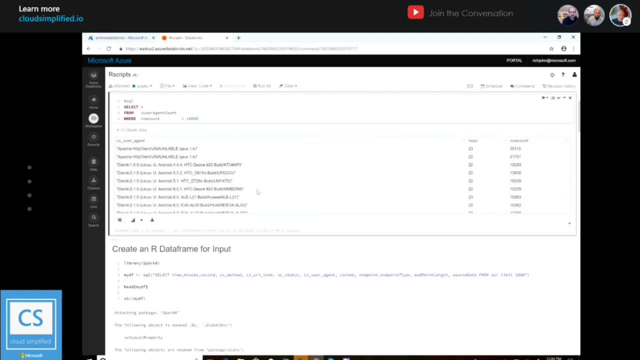 Just to look at things like counts by different clients And maybe they specifically do something with it. So nothing too terribly difficult here. But then you know how do we take some of these temporary views and put it into a data frame. 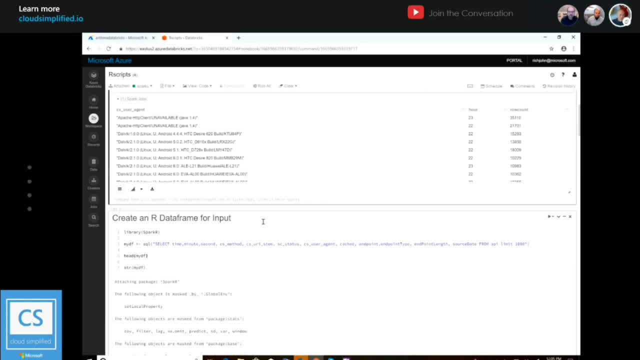 Things like data scientists are used to right. If you work in R or you work in Python, you're a data scientist. you work with things called data frames, So it's as simple as taking, you know, a select statement against that same data set or one of your tables in your client. 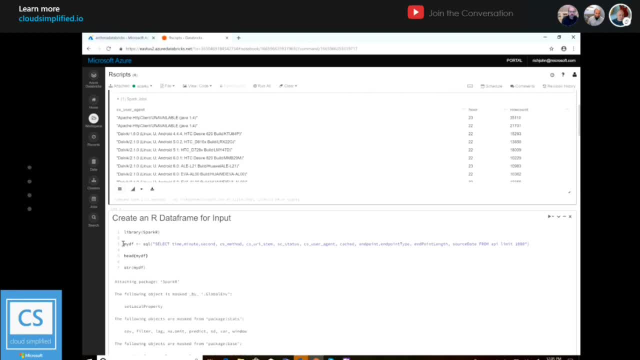 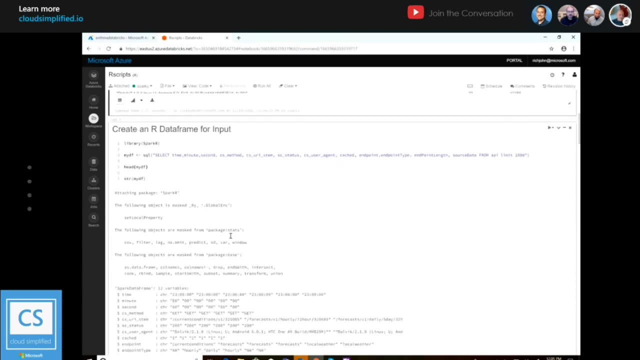 One of your tables in your cluster And this little notation here, mydf or my data frame, you know, with this pointer here to the SQL statement, will create a data frame. So once I have a data frame, if I'm a data scientist, then you can do things like you can look at the structure of that data frame. 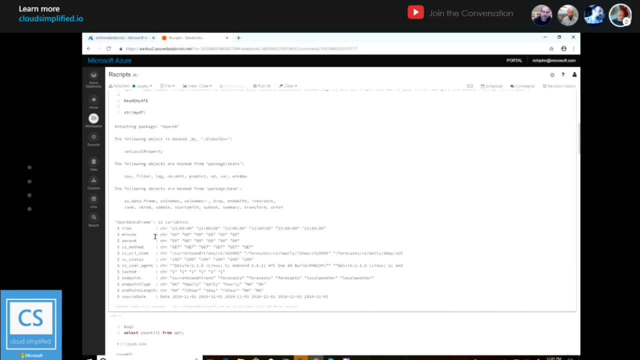 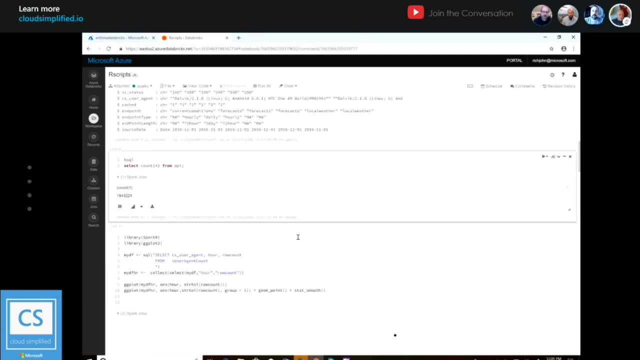 And you can see what it's composed of and you know from the different data types and features that are part of that data frame. I'll skip past this one. So once I have a data frame, then I can do things as a typical data scientist. 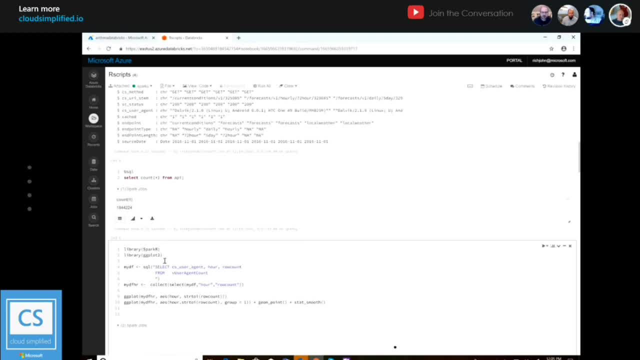 I can use these libraries like ggplot2, and I can use Spark R libraries to do things like plot my data. So here's another data frame creation where I'm just saying: hey, select from this view I created above And again, give me the agent, the hour and the row count. 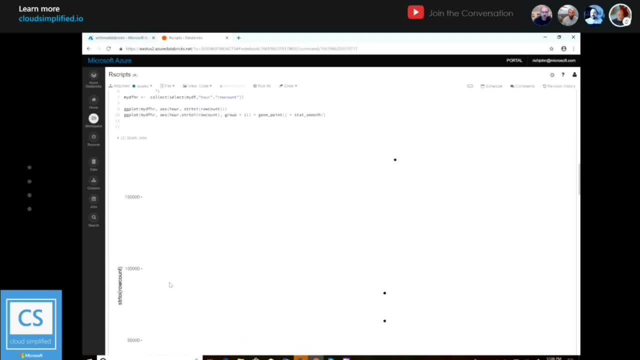 And then I want to go ahead and plot that data frame. So nothing terribly difficult, Nothing exciting here. But you know, if you're a data scientist, I mean ggplot2, there's just hundreds of different visuals you can make. 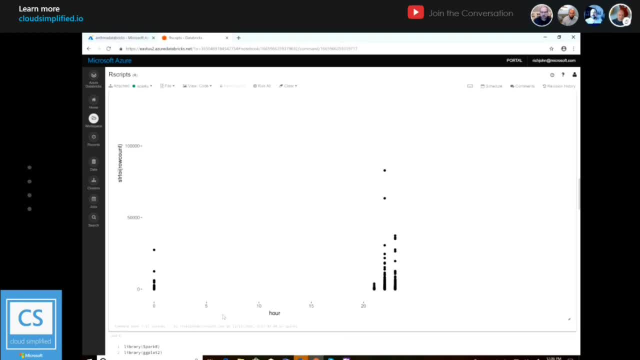 So you can see it aggregating across the x-axis by hour and then by row, count off the y-axis. So you can see a lot in this particular query. a lot of the hits are happening in this 50,000 or below at this, you know, between the hours of 20,000 and midnight. 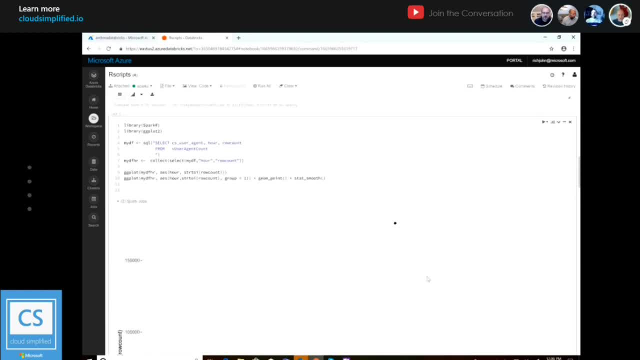 So just a simple plot. Is there a question in there? No, I'm mm-hmm, I'm mm-hmm, I'm mm-hmm. And then I noticed too, that it also was done in less than eight seconds. 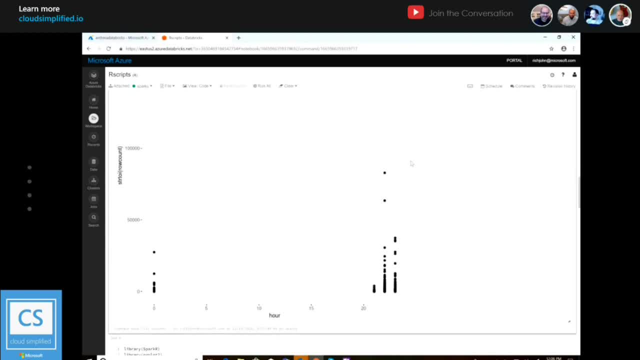 So, mm-hmm, That's good, All right, So we'll move to the next cell. Just a couple more here, So it gets a little more interesting. So if I create a data frame again- and in this case I kind of changed the name here- 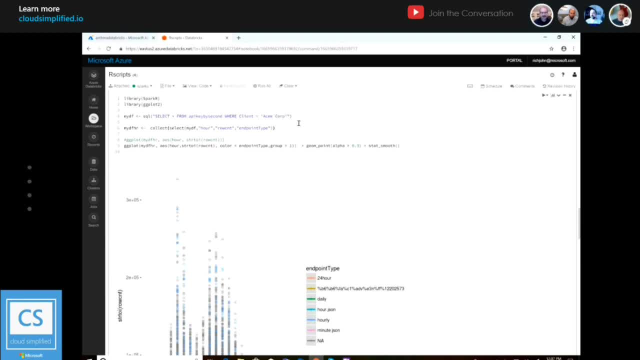 It was another actual client name, But I want to select for that. where I, for a specific client who maybe I'm, who's just a client, Who's generating revenue for me because they're using my service heavily, Then I want to look at when are their peak times. 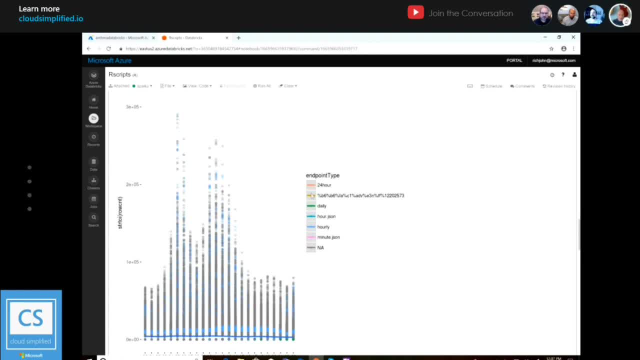 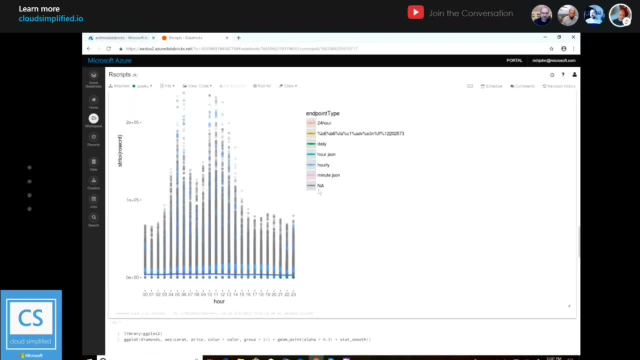 And what are the main. you know those end points. Anthony showed before What are the main end points And how are those being hit across a day And you can quickly see how that breaks out. That definitely hourly and there's some unknowns in here. 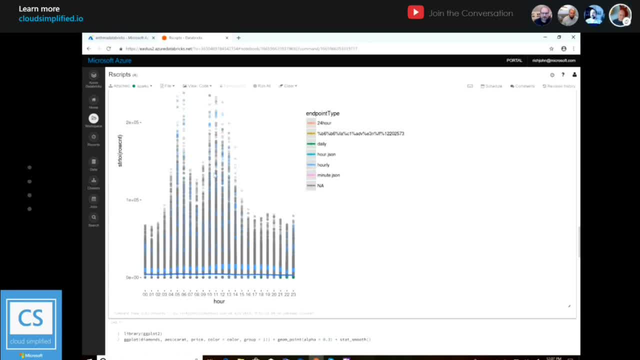 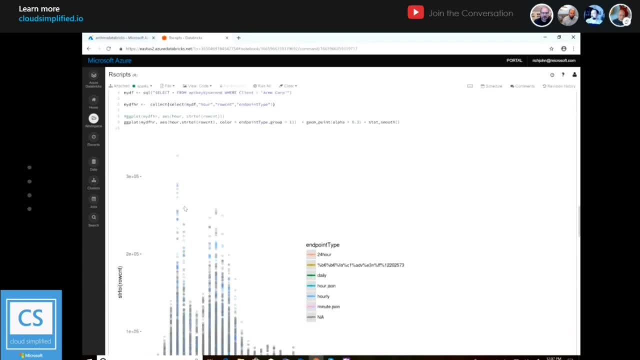 But the hourly type forecast seems to be hit a lot And you can see the different peaks throughout that 24-hour period. Oh, that's insane. This is amazing how rich the data can be so quickly. You know just how to bring it back. 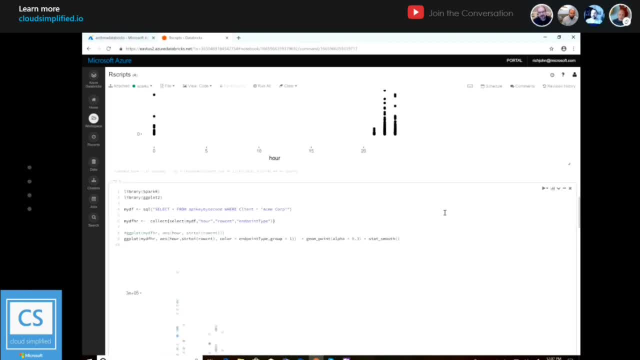 And again the other thing on scale. we're looking at a relatively small file in this use case, right Like 1.8 million rows, But when we were hitting it on a day level, I don't remember what the total count was, Anthony. 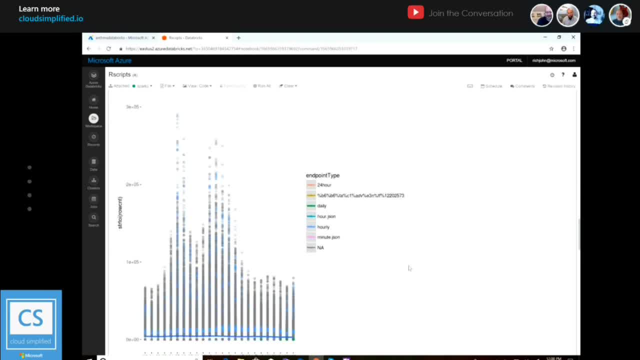 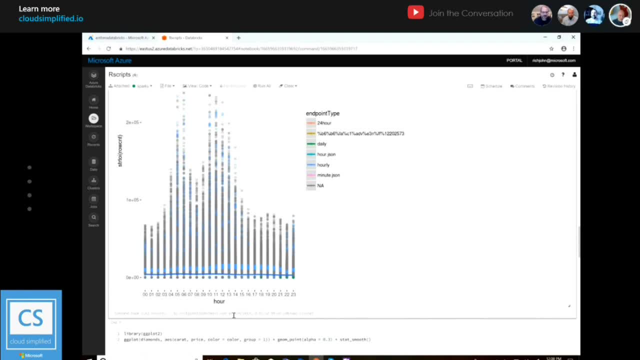 But it was in the billions of rows And we're getting, you know, generating these graphs and charts in the same amount of time this one took, And this actually was an old run against the entire cluster back in the day. You can see the date down here. 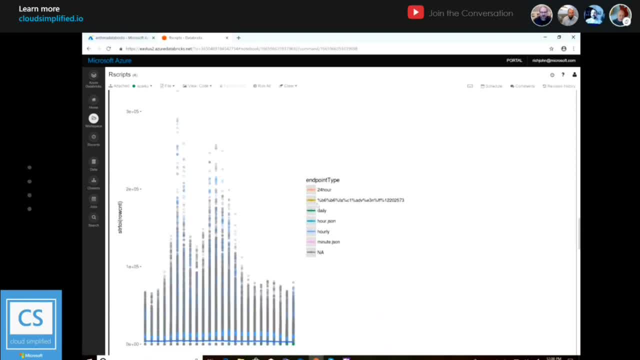 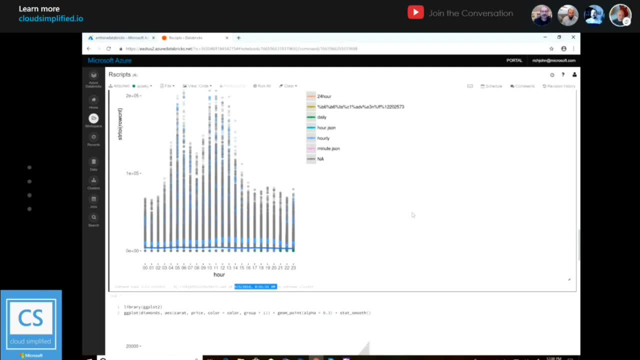 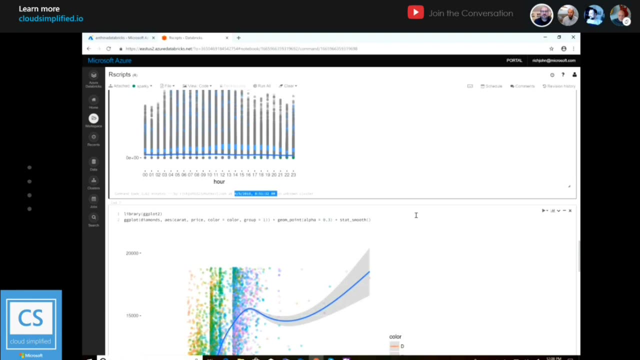 I just saved this cell for display purposes, But this was like in three minutes across that whole 20-some terabytes of data doing this type of aggregation and generation Dude. I mean, you know, I have witnessed multi-million dollar data systems go into companies and never be able to do things like this this quickly. 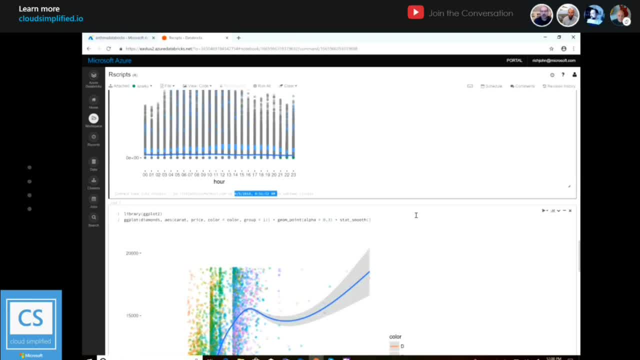 Or ever achieve these types of goals Ever. And companies struggle, Departments who justify the expense of these struggle to keep their jobs. because there's like you know business is like I need something to come back Right To. typically need very high performance disks. 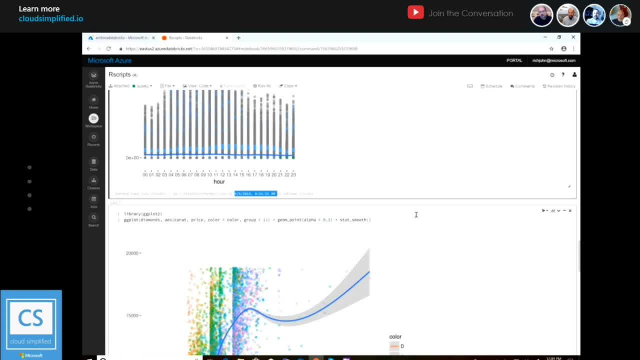 Oh yeah, I mean, oh yeah, You know, And again you're talking to an old timer like me, So I kind of take this for granted now, But I was the one that did all that planning to buy that kind of stuff. 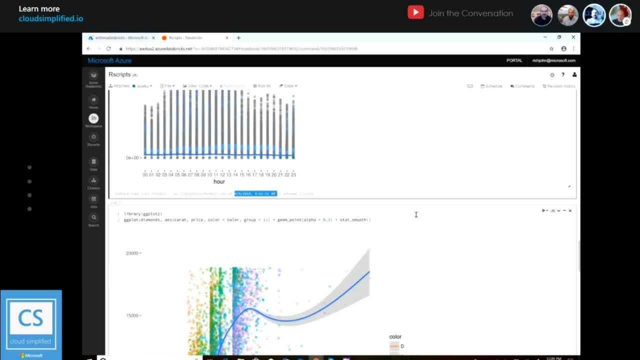 Oh yeah, Yeah, And it was not expensive. We're in multi-million dollars now. We're spinning up, you know, $10 million clusters here. if we need it for just five minutes of work and tear it back down to get these kind of results. 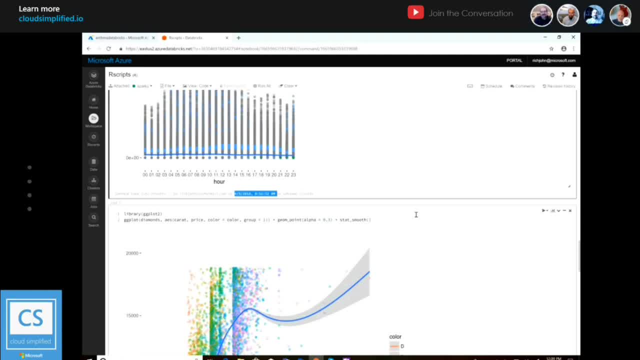 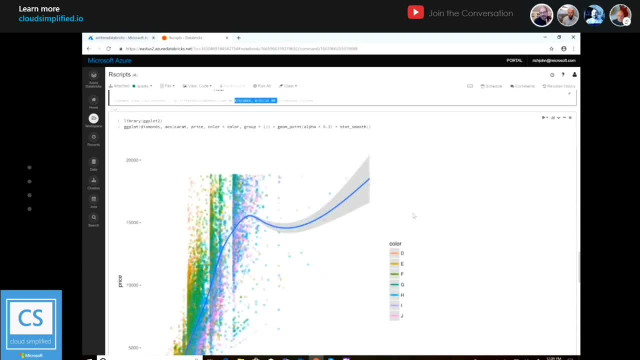 So it's mind-boggling when you look at the whole work we're doing here. Yeah, There's three- you know three-letter initial companies that made their billions off of this stuff, doing it on-premise. Absolutely, We'll mention them. 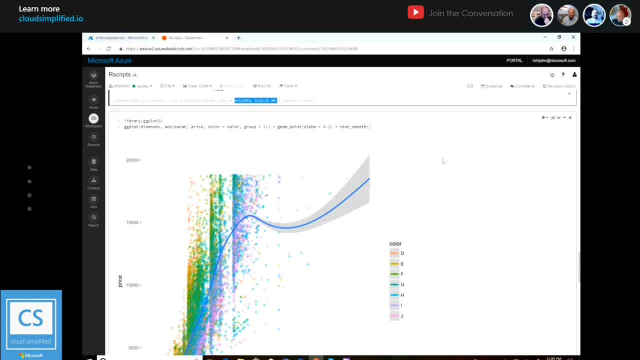 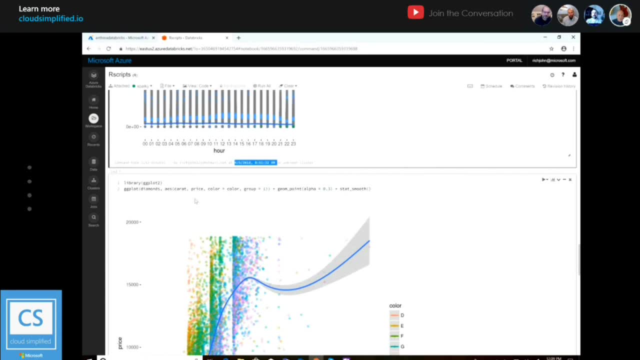 But just three, Yeah, So I think this might be the last example. This is one of the built-in data sets called Diamond, just to show you some of the full richness of like these plot libraries that are available to people who work in R. 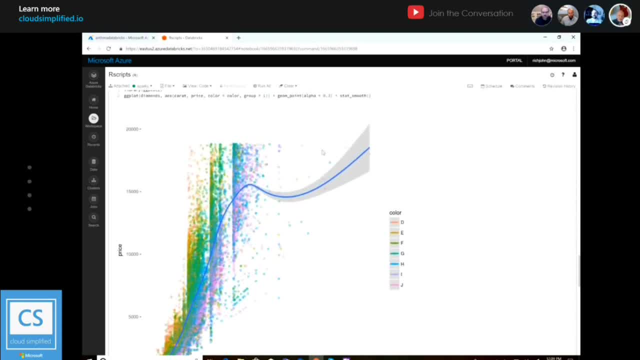 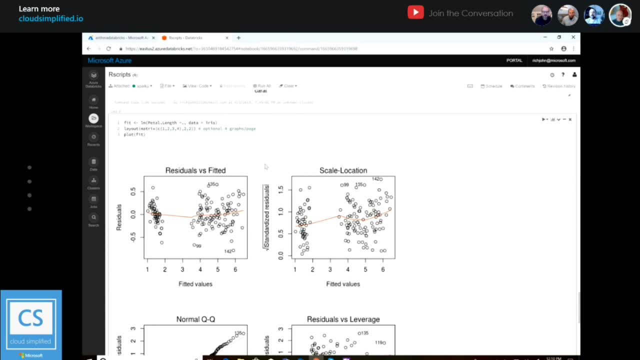 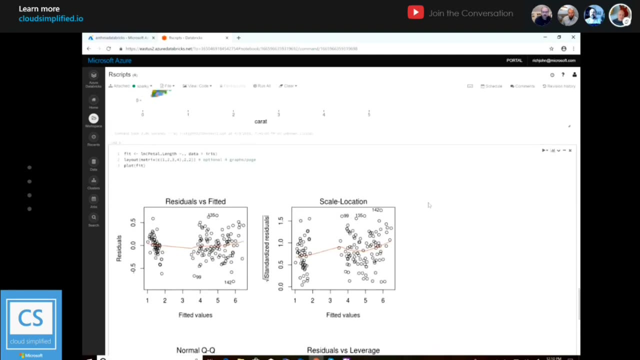 And you can do some pretty much rich visualizations. And then you know the real statistical work when you look at things like quantiles and residuals, fitted models and probabilities and all that. So you've got all that richness. So again, if you're a data scientist, you're looking at a few lines of code here in the Spark Databricks cluster. 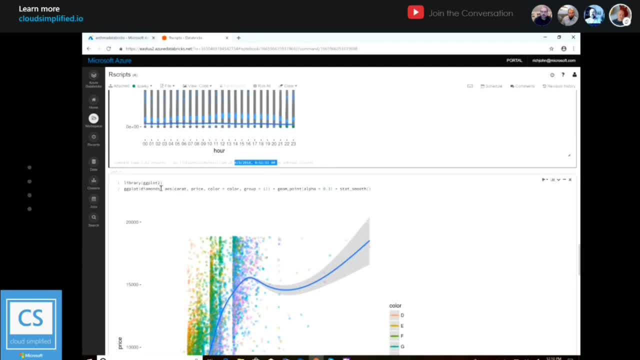 But if you're a data scientist, the ability to attach to that cluster and do this at scale. you know most of these guys in the past have typically got a powerful workstation And they still can't load 600 gigabytes of compressed data day in that workstation. 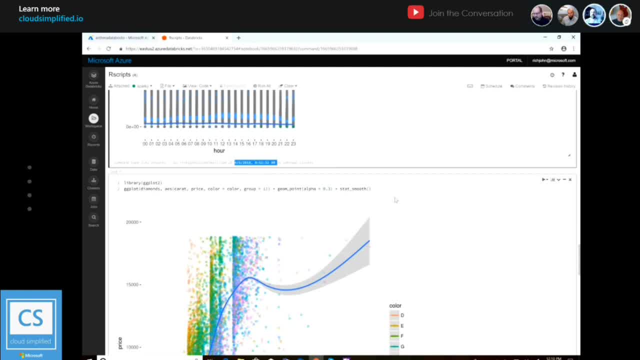 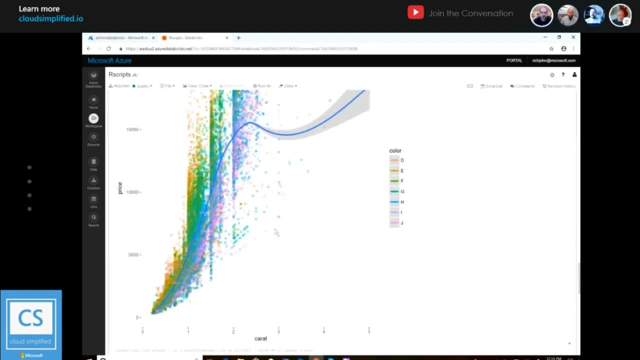 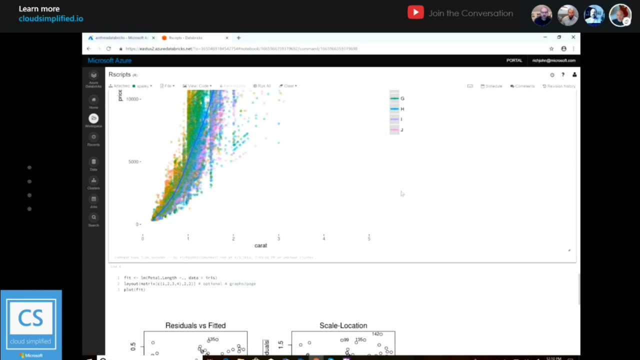 Oh yeah, But now they can take that subset, get it working in their workstation And then just simply take their scripts over here and put it in a cell and generate this kind of analysis against the entire data set and entire cluster. So again, just mind-boggling what they can do at scale with big data. 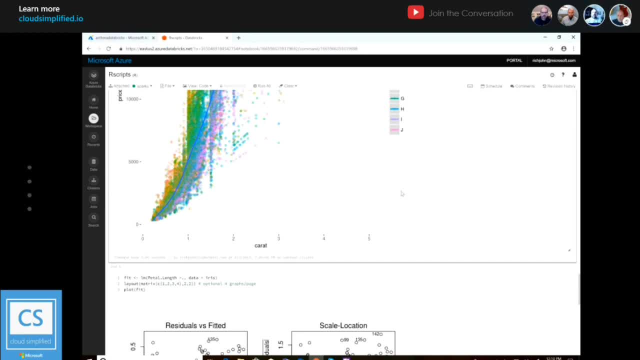 Yeah. So thinking about, like the business problems that this actually you know solved for them, like what did this, how did this change or alter their view or lens into you know data You know before? I mean, it sounds like they had access to these lenses. 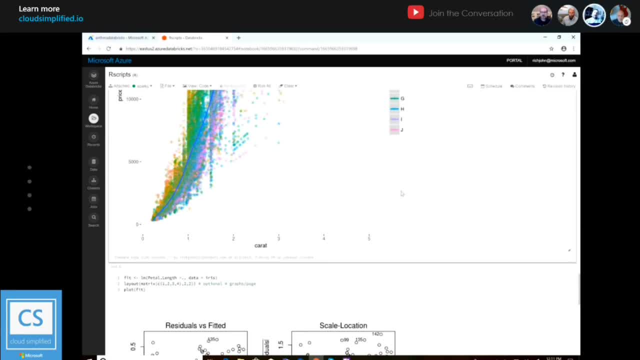 Yeah, They had access to these logs, Maybe not as readily able to consume and digest them as this extended to them. I know you said that they were using HDInsight. Maybe they were doing something to this degree, maybe just not as easily. 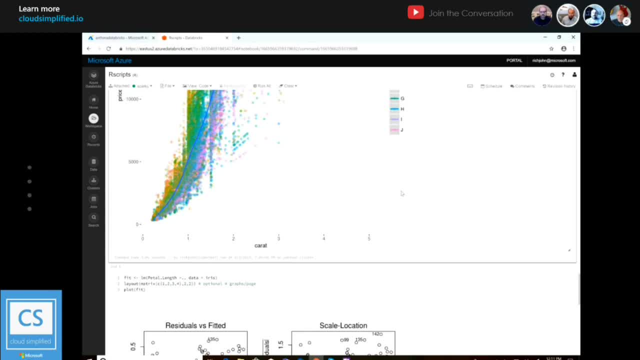 Is that just trying to kind of net it all out in terms of business value, you know, to your customer. So, in a lot of different ways, I mean one. they need to make sure that clients that have access to the different APIs are utilizing that data. 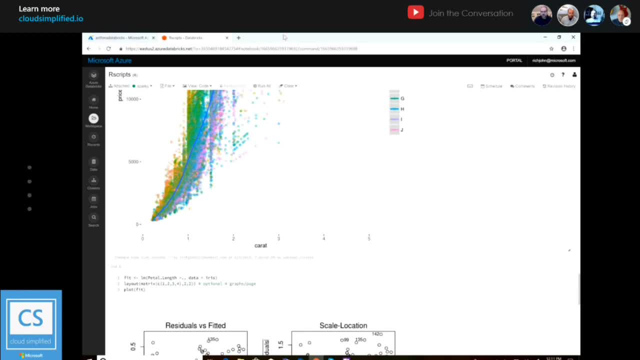 Other APIs are utilizing them based on kind of the criteria that was in that business agreement. so they can now start to analyze that more efficiently to make sure that people aren't using making tons more API calls than they should be. Okay, But what they're looking to do now that they can do this so easily and they can get different groups of users collaborating in this central environment, they're going to pull in additional data sets so that they can. hey, our API spikeage tends to happen when different weather things happen. 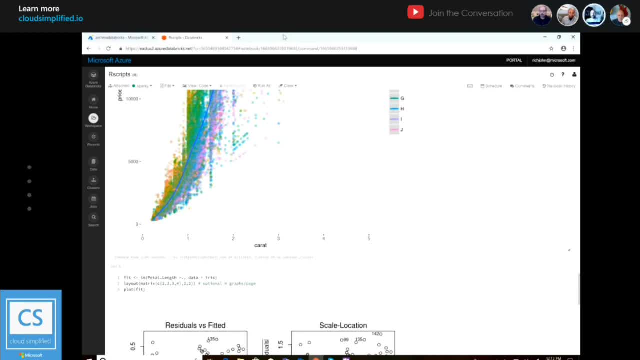 So they can use that for you know different ads that want to get shown things along that nature. It just helps them understand their business a lot more efficiently. Okay, Okay, Yeah, We just kind of touched on that a little bit. the collaboration: 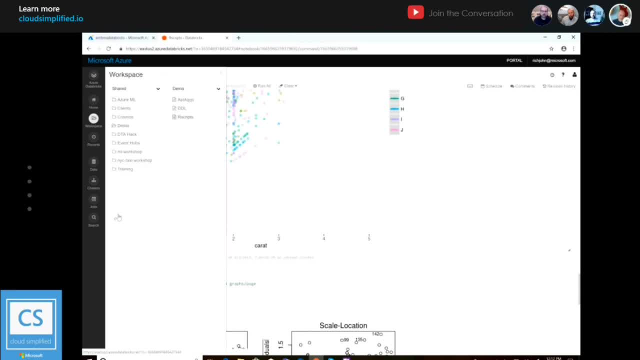 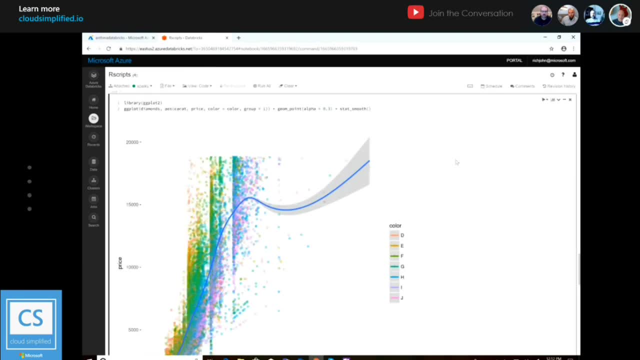 But, like Anthony showed the workspaces right, You could have these shared workspaces so and you can give permissions to different business groups and that to see their work. And again, these notebooks are so self-documenting that you can go through and see the analysis that someone went through to get to these topics. 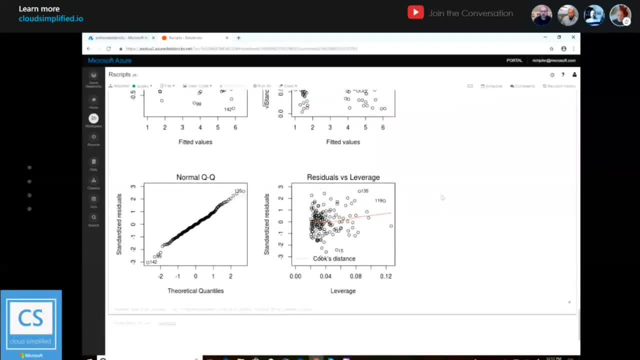 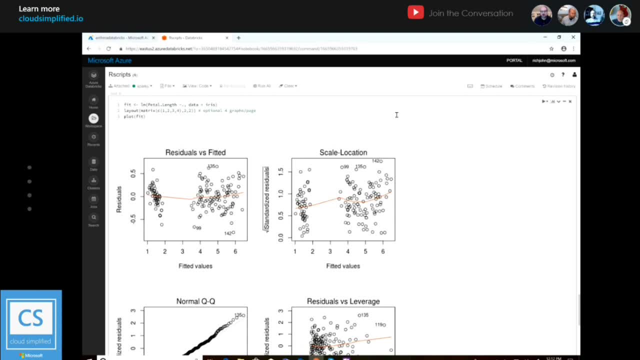 Okay And you can go through and see the analysis that someone went through to get to these types of plots and visualizations And then you can simply borrow that work or create a new notebook. So I mean, the collaboration environment for data scientists, again on a cluster at scale, is just. it was something again that was very surprising to both Anthony and Howard.